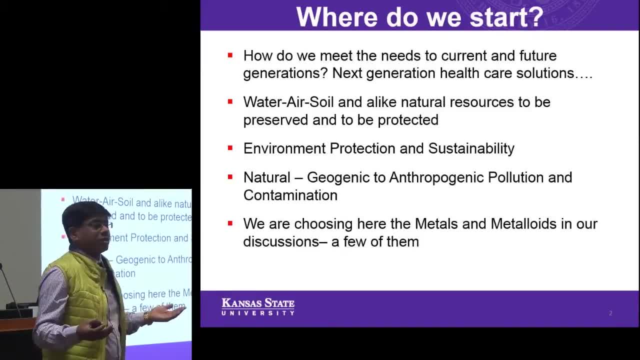 That means it is naturally produced by natural processes of the earth. And when they are human induced, definitely they are the anthropogenic, But they are related to each other, They feed onto each other, And that is what I will try to build the story upon today. 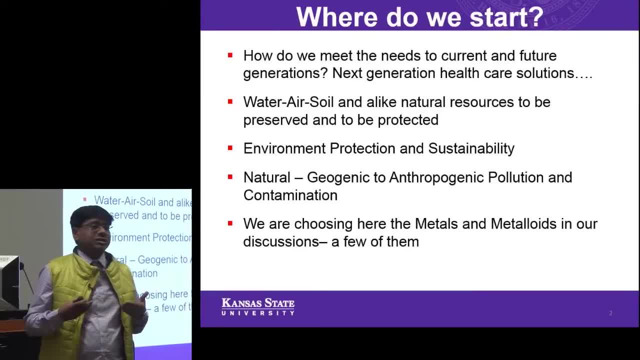 As to how these metals and metalloids are actually not just natural but also quite a bit experienced by the anthropogenic pollution scale too, And we are going to choose for this talk on the metals and metalloids, and we will discuss a few of them. 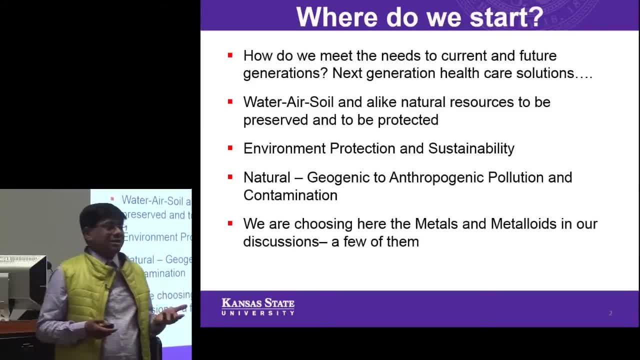 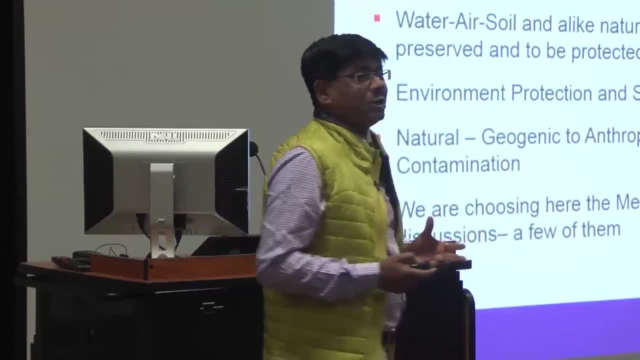 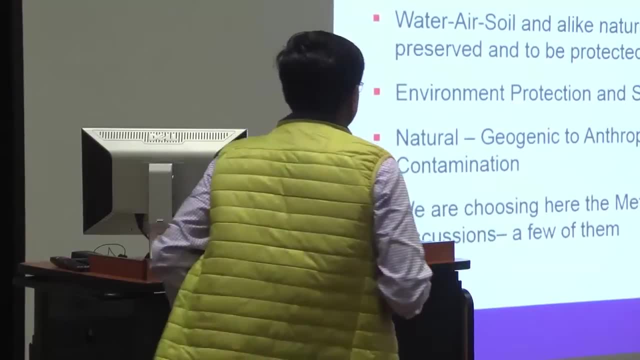 As you will see that there are so many to discuss about the beneficial and the toxic components of these elements, It is very difficult to choose all of them, So I chose some of my favorites, Let's put it in that way, And I am going to give a little bit of a brief introduction to each one of them. 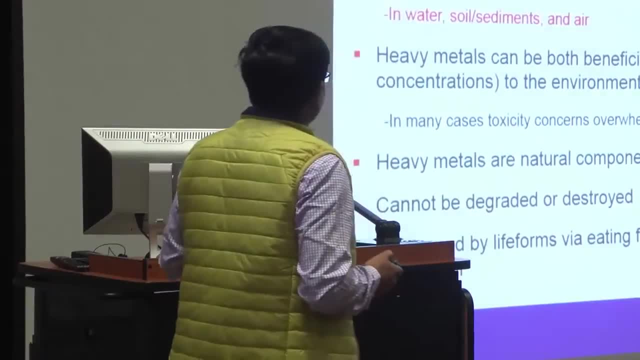 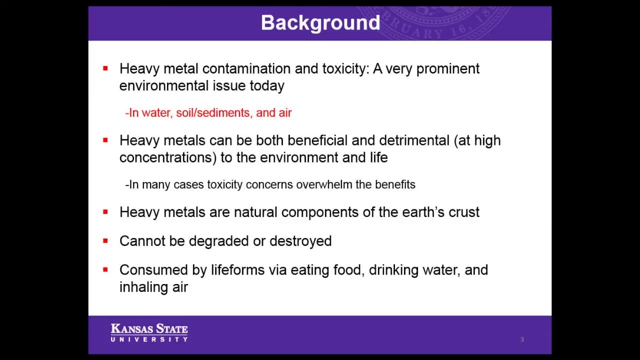 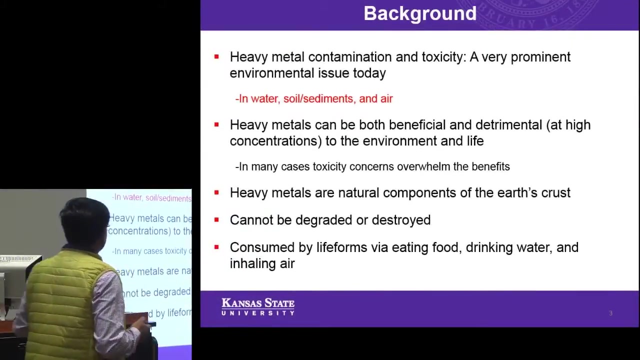 So just a little bit of background before we start. Heavy metal contamination and toxicity: these are related terms Because they are very prominent environmental issue today And the issue is for environmental restoration. for the water, air and soils. They can be both beneficial and detrimental. 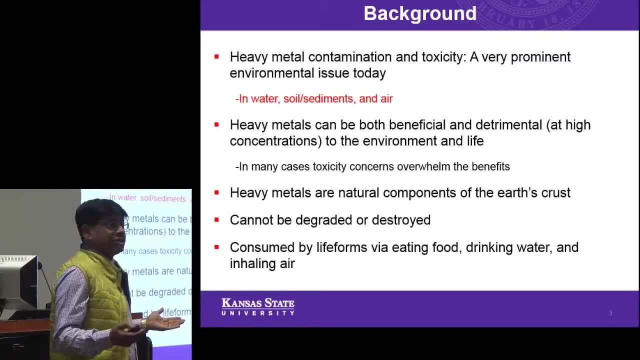 That means at high concentrations, these same elements, which might be essential to our ecosystem, may be not only just toxic, but it may be fatal. Now, in many cases, the toxicity actually Overwhelms the benefits of those elements to the ecosystem. And the heavy metals are mostly, as I said, are the natural components of the earth's crust. 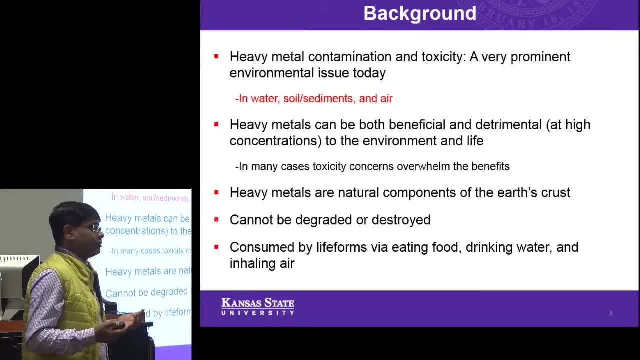 So it comes as a background level in majority of the earth's crust that we work with. I am not including the radionuclides, So I am safe to say that these metals that I am going to talk about cannot be degraded or destroyed. 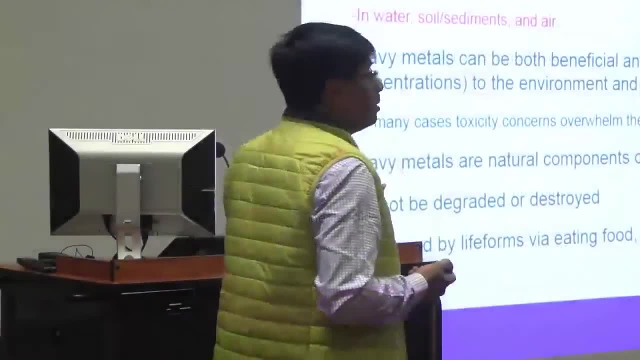 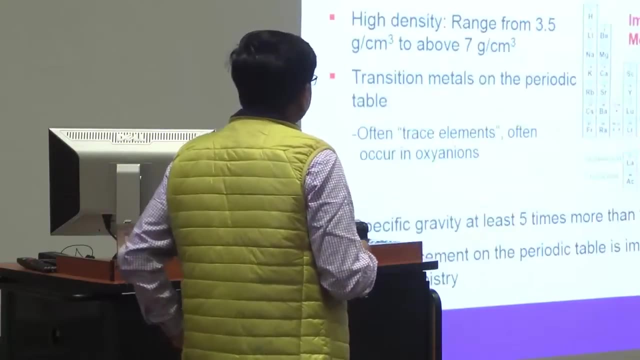 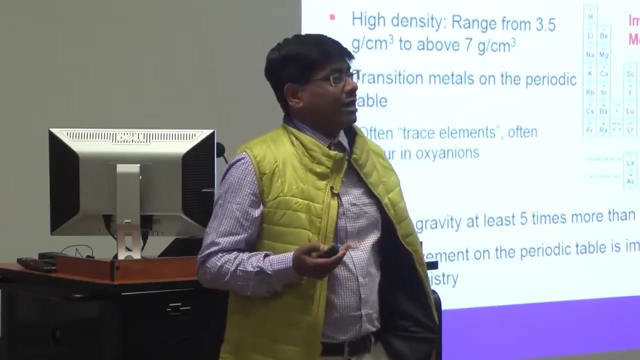 And hence these are consumed by life forms via three pathways: by eating food, drinking water and inhaling air. So the three subsets that I just mentioned. So some very basics of the heavy metals. The definition wise: any metallic chemical element that has relatively high specific gravity. 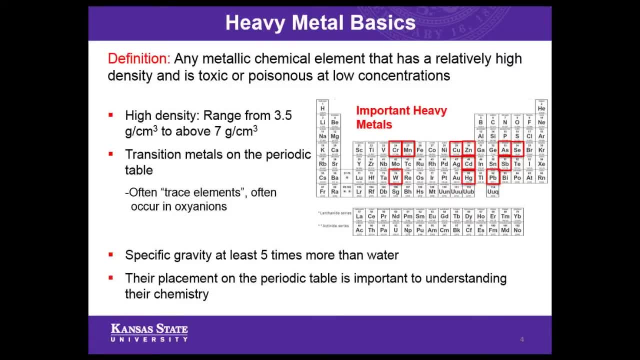 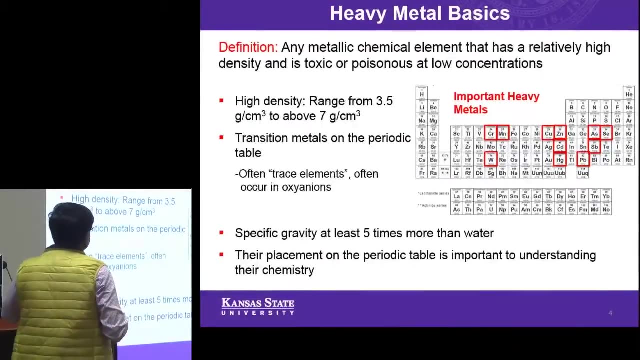 And is toxic or poisonous at low concentrations, And this term low concentration actually has a big meaning to it. What level of the concentration you are exposing a population to is a major debate, And lot of these toxic elements may not be toxic at some concentrations. 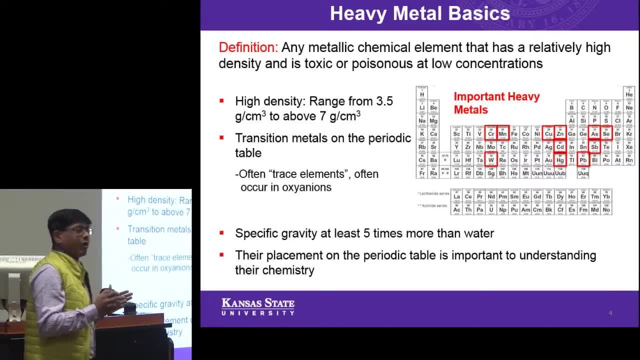 So always this dose response: feedback is important. when we talk about heavy metals and their toxicity, Again it is their high density. Usually the density ranges from 3.5 to 7 grams per cubic centimeter. They are usually in a periodic table. 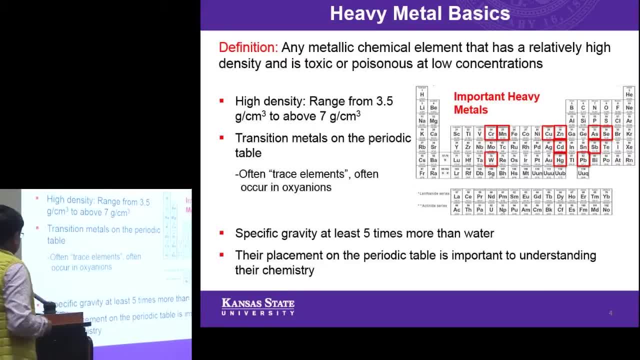 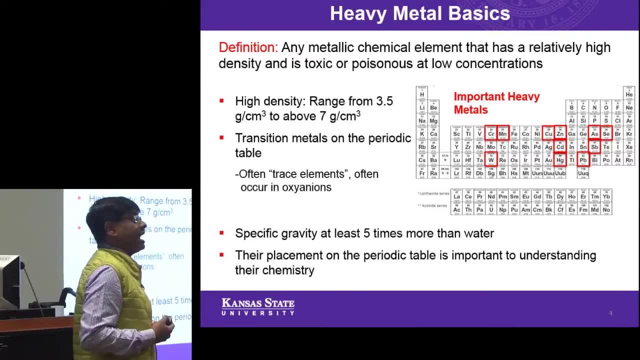 In the chemistry classes that you have taken. definitely all of you are exposed to that. They are usually the transition metals. Not all of them are transition metals that are heavy metals. They may be some of the F block elements also, And they are sometimes also termed as trace elements. 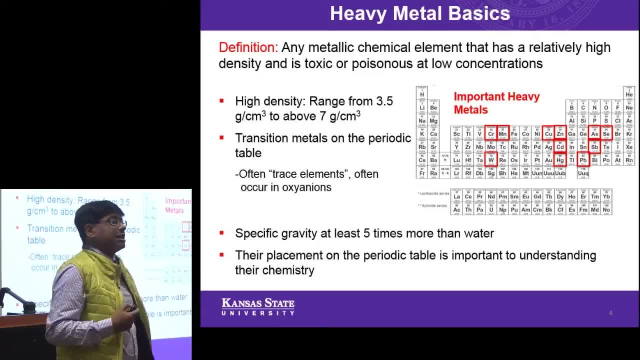 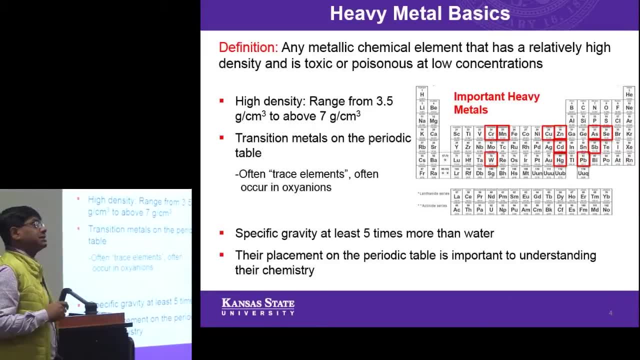 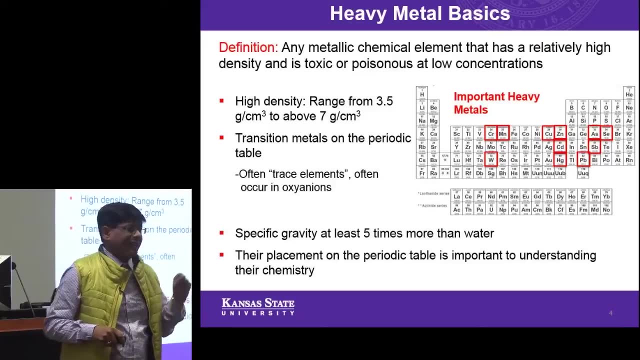 And the elements that are usually in the water form or in the air as oxides, And such elements are called oxyanions. Now, the trace elements part is more of a concentration term. Heavy metals is more of a chemical term, So there is a distinction between the two. 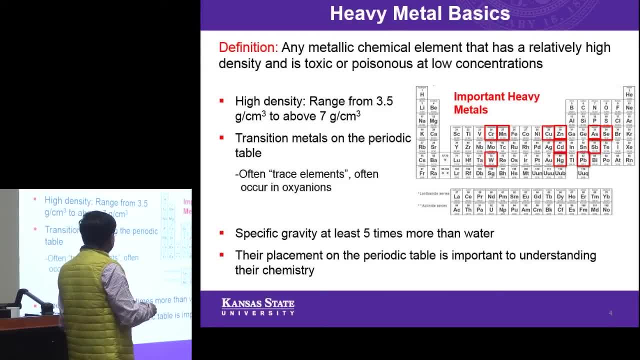 And again, the specific gravity when we talk about is has to be about 5 times more than water, And their placement in the periodic table is very important to understand the chemistries behind it. A very simple example of this and I am going to talk about a little bit at the end. 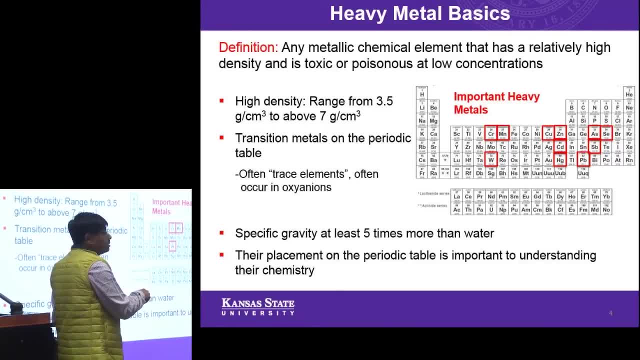 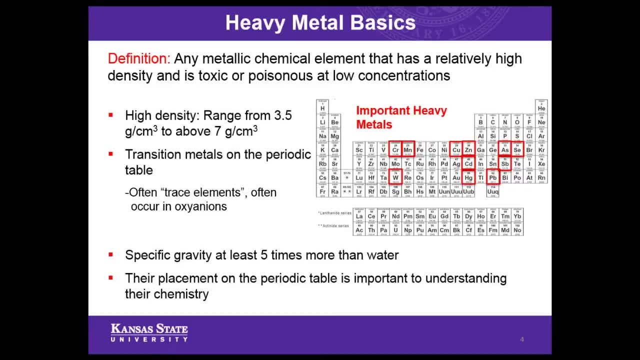 Is between molybdenum, which I didn't actually encircle, and tungsten. Now you might be quite surprised to hear these elements about. A tungsten is a pretty toxic element in nature, But it is very beneficial. We don't know much about tungsten. 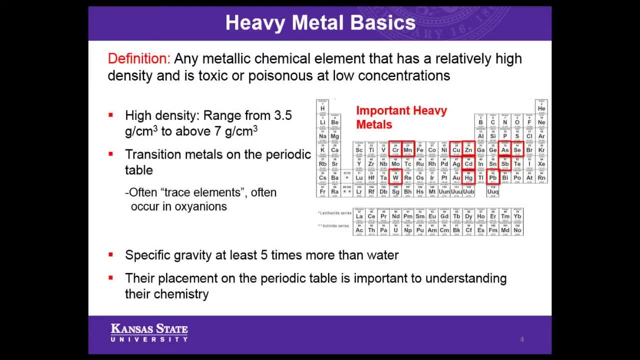 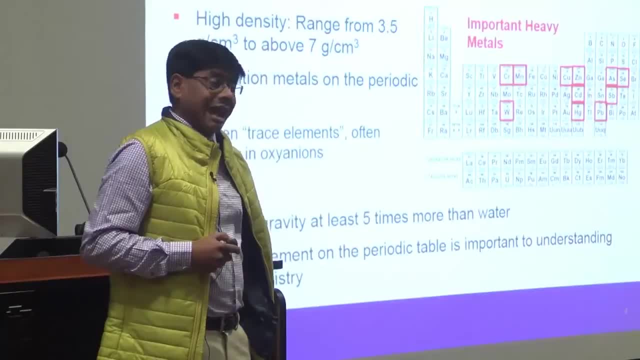 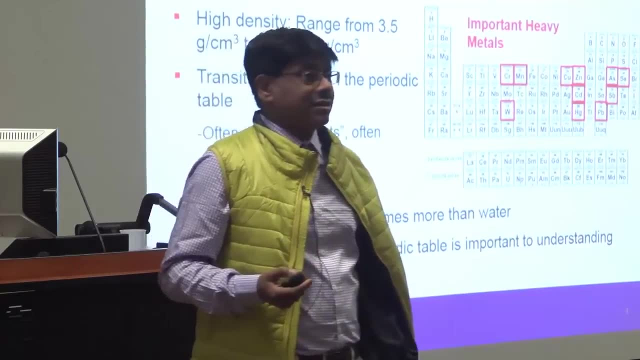 To study tungsten, we need another element to study And that is molybdenum, Because the molybdenum chemistry in natural waters and in air is very well studied And people understand. scientists understand that much better. So the geochemical association of elements like tungsten and molybdenum are important to understand. 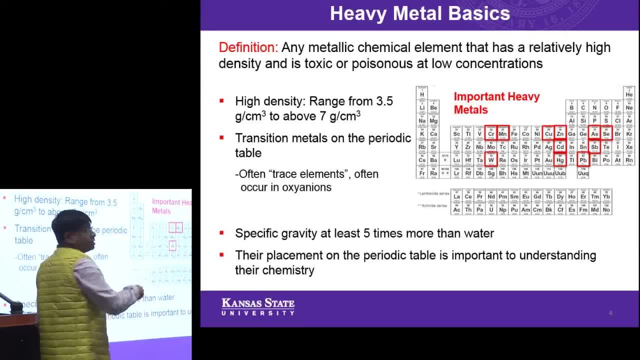 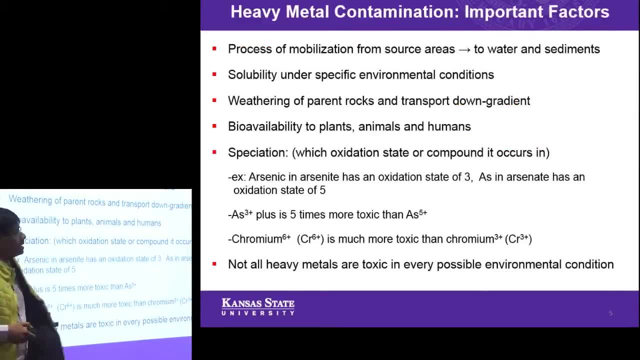 So that the deficiency of information on tungsten can be fulfilled by understanding molybdenum. So, with that in mind, some important factors that I like to point out. For example, the processes of mobilization, So, as we can see, these metals have to come from a source area. 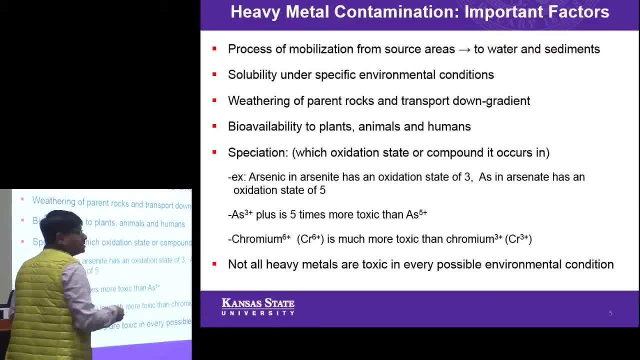 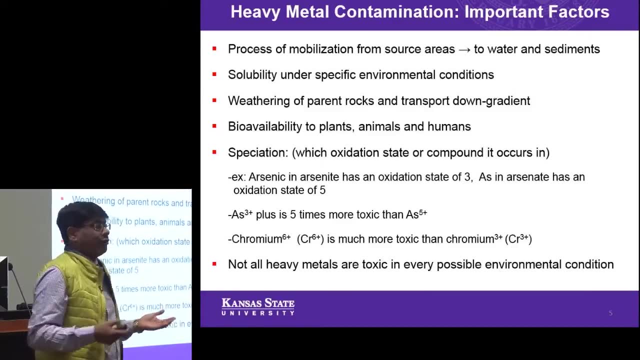 And the mobilization process happens in the water and in the sediments. Usually these metals can be soluble under specific environmental conditions. When soluble, they are fast dispersed in the environment, Usually in the natural environment- weathering of rocks- And then they are transported down gradient. 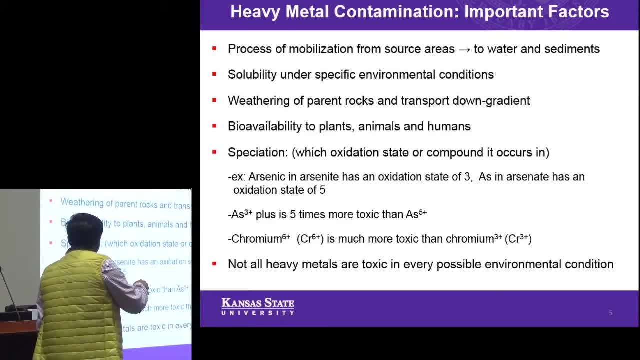 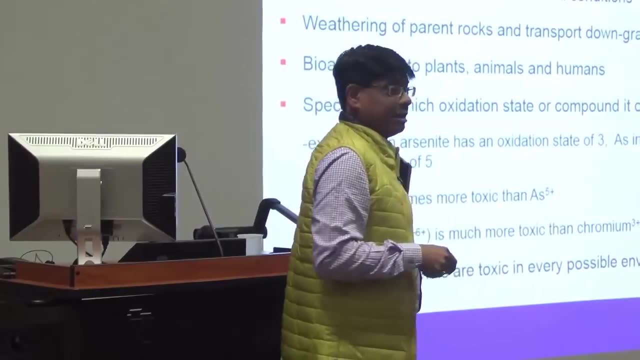 Causes the accumulation of these heavy metals. These metals are bioavailable to plants, animals and humans. The important concept of heavy metals is their oxidation states or speciation. For example, arsenic you might have heard about is a toxic element in nature. 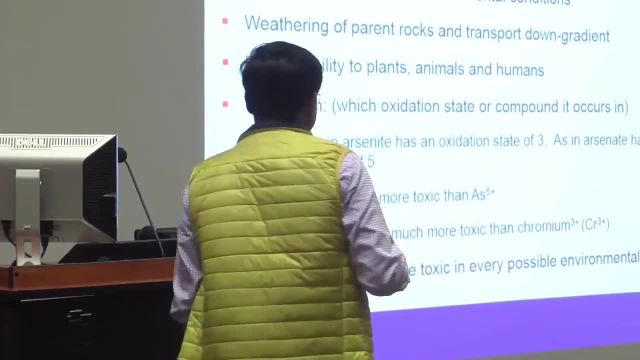 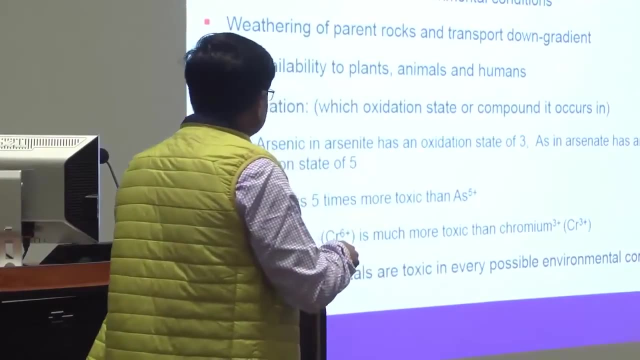 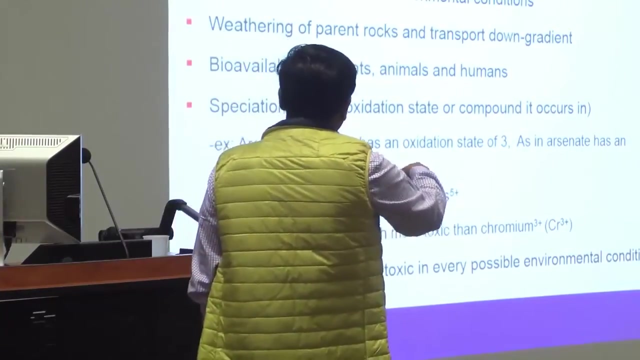 It usually is present in two oxidation states: One is plus three and one is plus five. Plus three, which is a trivalent arsenic, is five times more toxic in the environment than plus five, So the speciation is an important concept for each one of the elements that I am going to talk about. 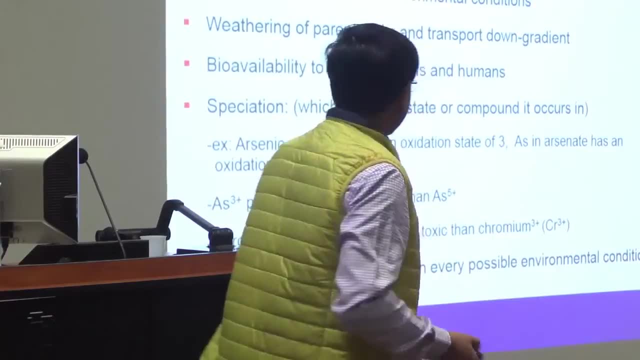 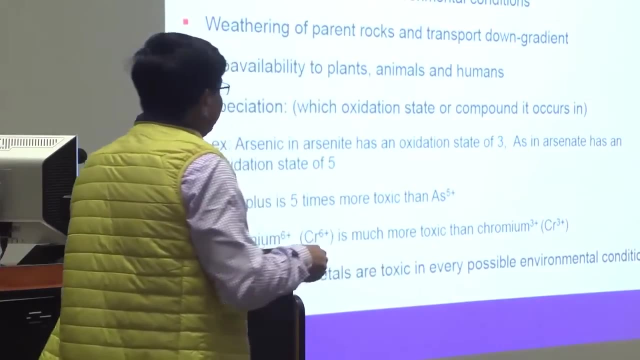 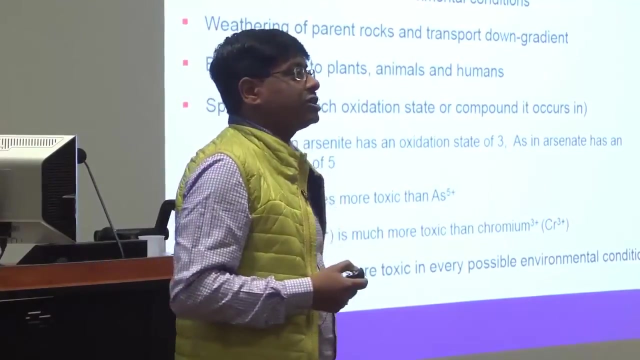 And each one of the elements that I may not be touching upon today. Similarly, chromium six is much more toxic than chromium three. Now, not all heavy metals are toxic at every concentration. Rather, I will say that at possible environmental conditions certain elements are toxic. 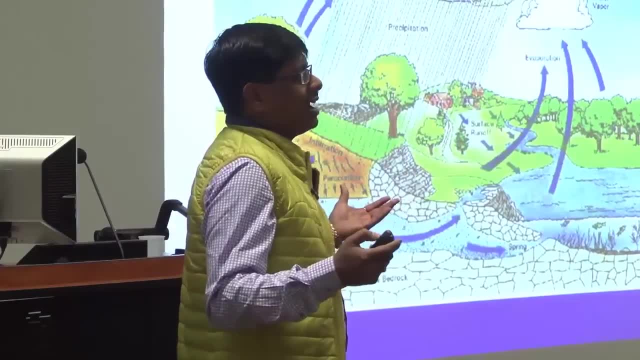 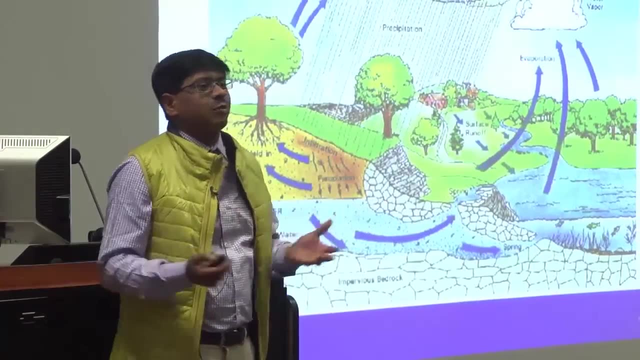 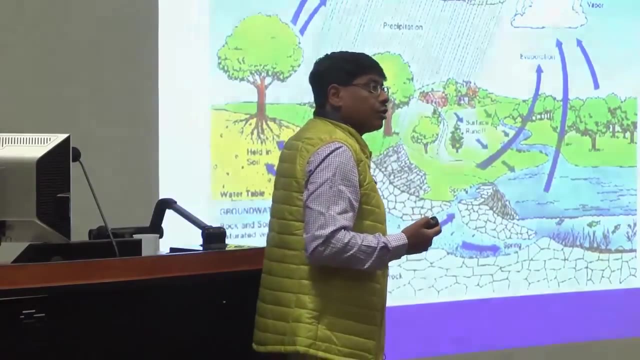 When we talk about dispersion in the environment, one cannot escape the hydrologic cycle Or, in a very simple sense, the water cycle. You might have been exposed to the water cycle in many forms. These are the major pathways When the precipitation happens, then the runoff goes into the ocean. 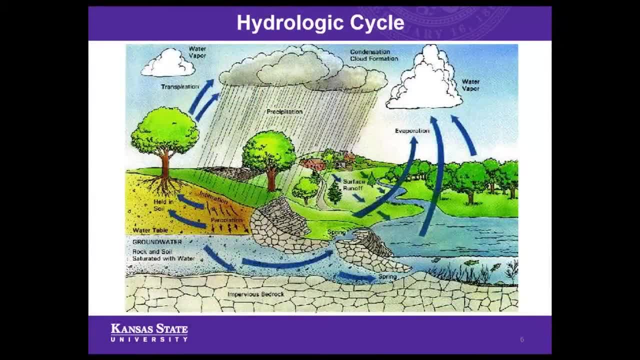 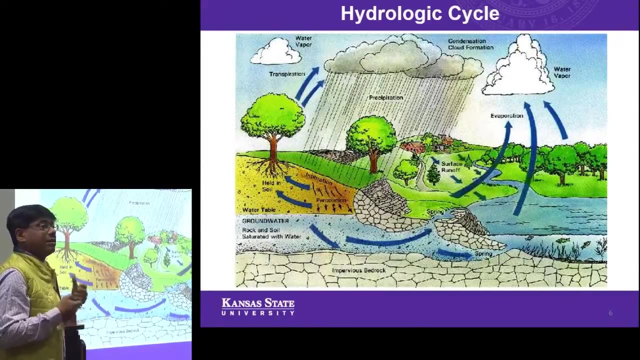 In filters down into the aquifer as ground water. All these are different pathways and reservoirs where heavy metals can reside and can get dispersed. So this is an important framework under which, in water, essentially you can understand the dispersion mechanism of heavy metals. So when we talk about the transport processes of these metals, 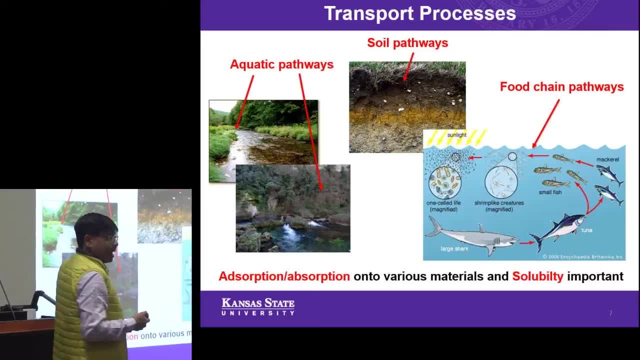 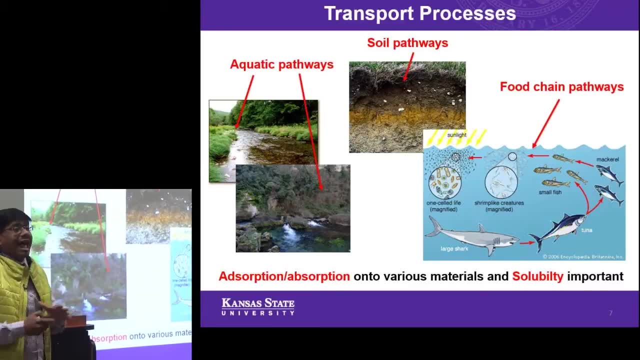 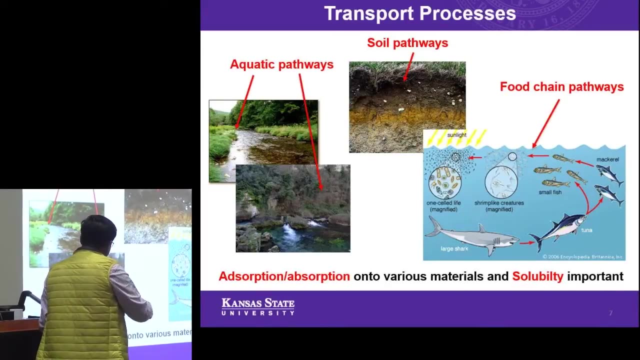 Important path is the aquatic pathway, in the water resources From the soil leaching from the soil down, vertically down and then accumulating up the food chain And the processes that leads to it are the process of absorption and absorption onto the various substrates: soil, sediments or water or particulates. 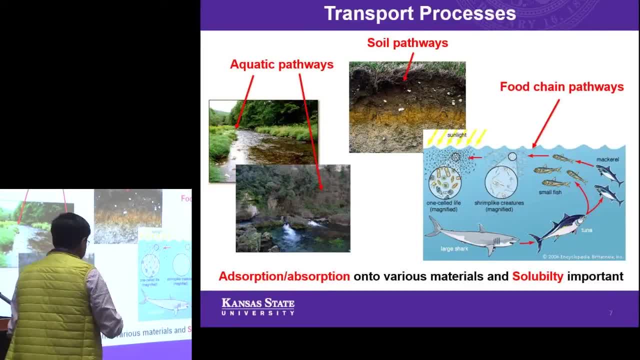 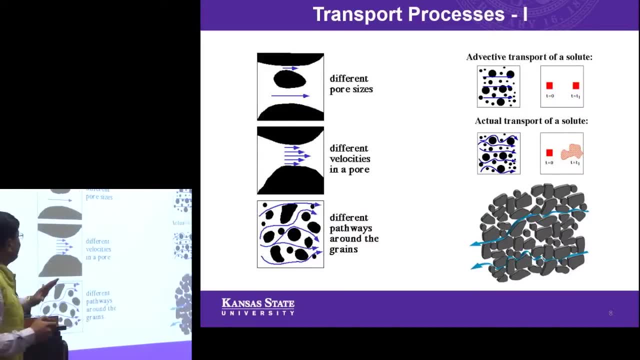 And solubility is an important factor over here for these metals When we go a little bit more in depth into the transport process. I just wanted to give you a brief sense of how this happens in a closed environment, like in your aquifer, Down underground, in where the ground water resides. 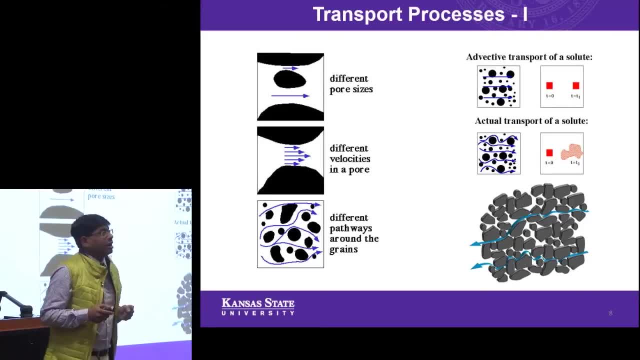 The transport process depends upon particles, because the water has to percolate through the particles that are present there. So what we need are different pores, The different sizes of the pores. The arrows indicate that a smaller pore size is a smaller velocity of the water with the plume of the contaminant. 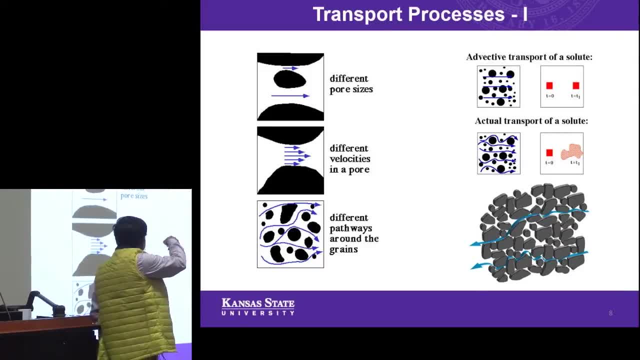 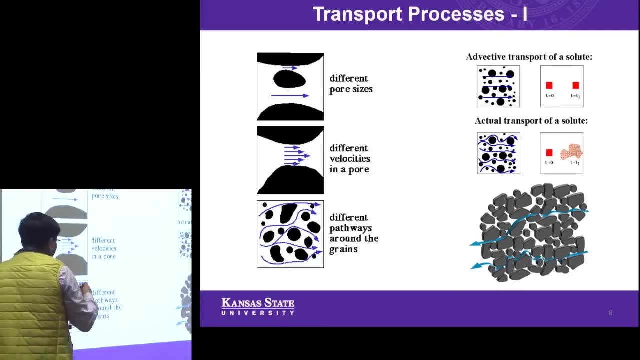 And a much more dilated pore will have a much higher velocity of the contaminant along with the contaminant. essentially, Now, when we have a single pore but much you know, much more dilation, then the central part of the pore will have the maximum velocity. 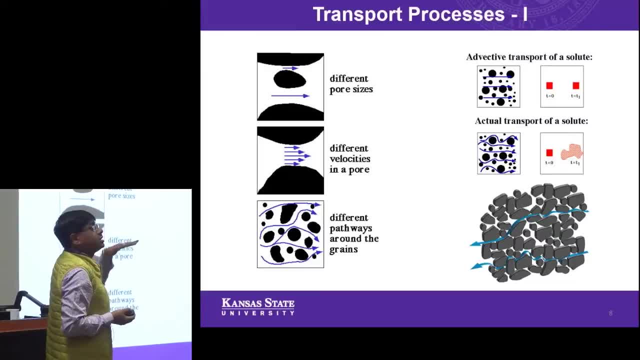 While towards the grain boundaries, because of the friction, the velocity will be less And again water in a system, in an aquifer, ground water, usually progrades in a sinusoidal pathway Because it tries to find the pore spaces which are connected and hence it is not a linear pathway. 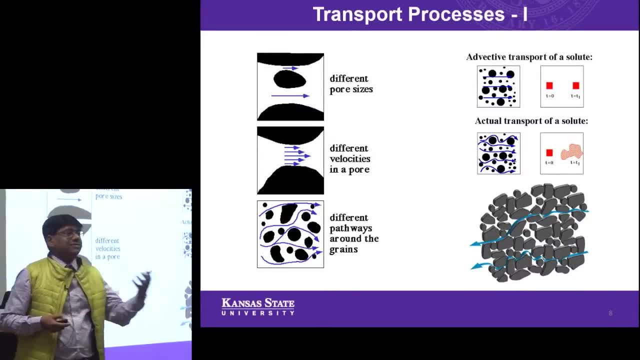 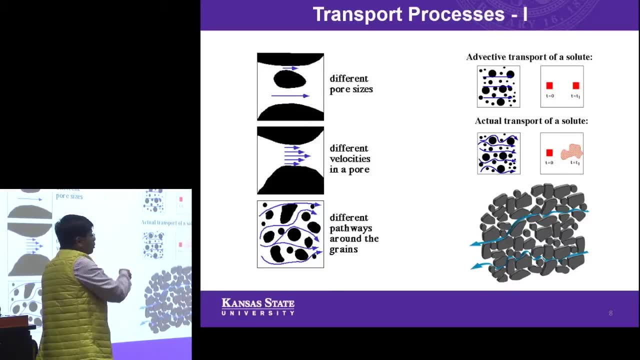 Now there are when we actually transfer a solute meaning, in this case the metal. We may do that in an advective process of transport, That means the body itself moves, Or when we look at the actual transport process of the contaminant, this metal. 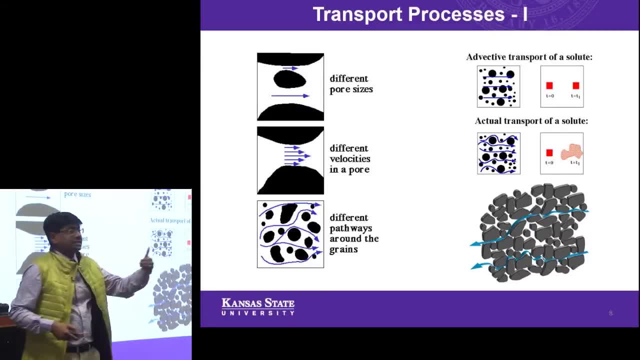 It might actually spread for a distance. So t is the time through which that metal has prograded. Now, as I said before, that along the particles, this is the water pathway or the parcel through which the water with the contaminant will move A little more into it, because this is somewhat necessary to understand this kind of a differentiation here. 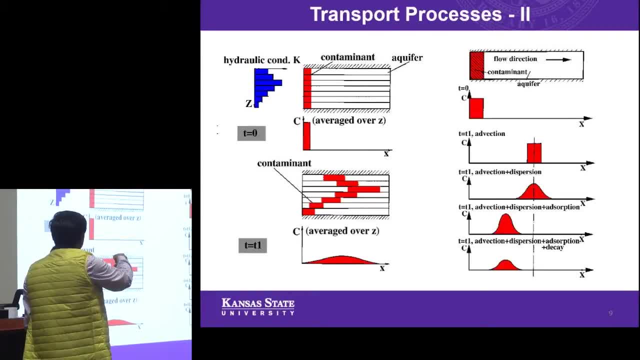 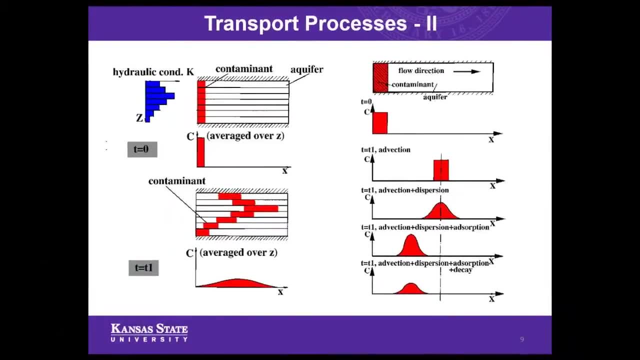 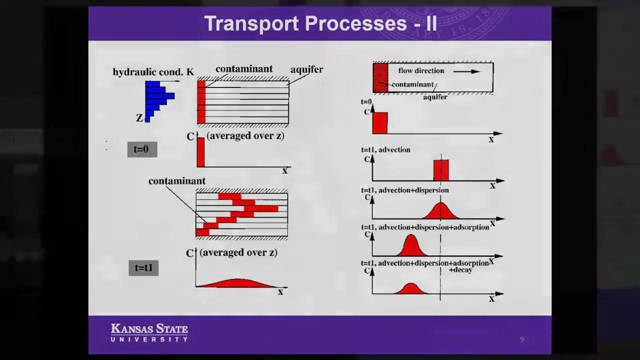 On the left. what I am showing is a distribution of a very important component of the aquifer property is called the hydraulic conductivity. Now, when the hydraulic conductivity is high, the mass will proceed in a much higher distance. this is the x axis. So basically, a contaminant with the water will move further distance in the layer where hydraulic conductivity is higher. 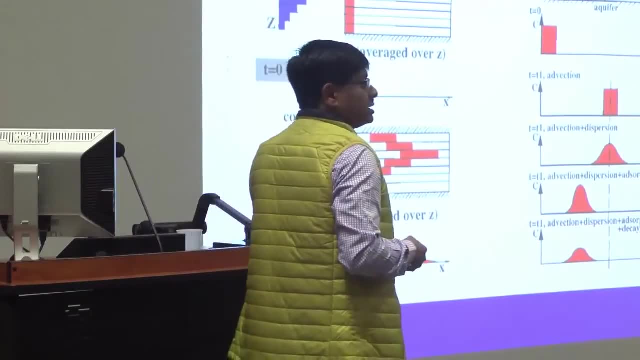 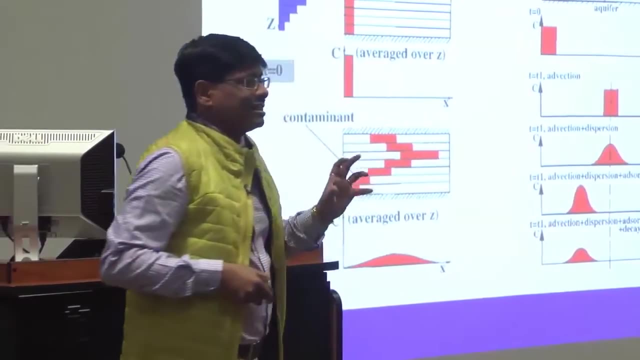 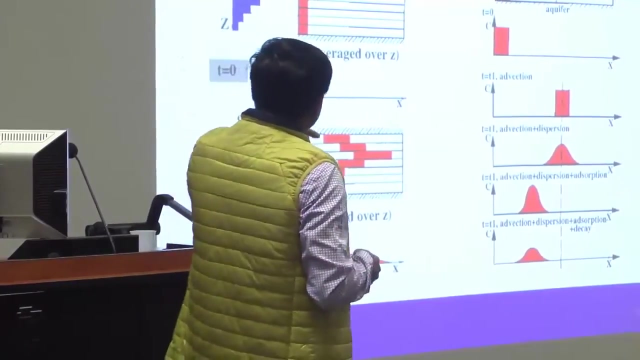 And lower, it will move much smaller distance on the x axis when the hydraulic conductivity will be lower. So essentially, the guidance by which a concentration of a contaminant, in this case a metal, will move through the aquifer will depend upon the aquifer characteristic. 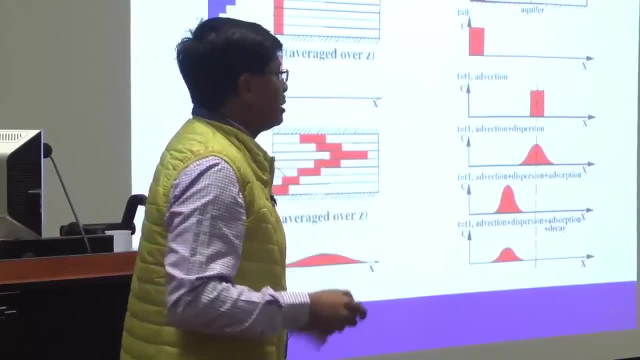 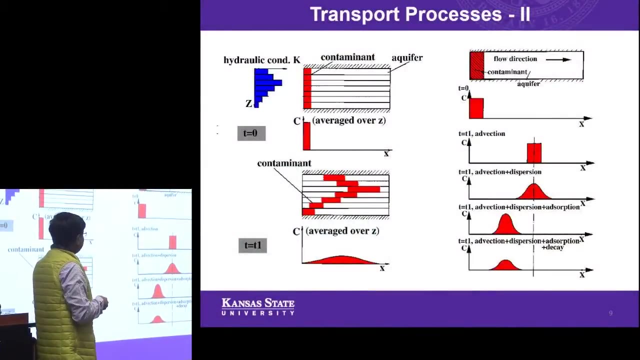 There are four modes of movement of contaminants, very basic way, And those four movements are: One is advection, where the contaminant itself moves in an x direction, like, as I said, When dispersion is added to it, it just disperses a little bit more on the x axis, as you can see. 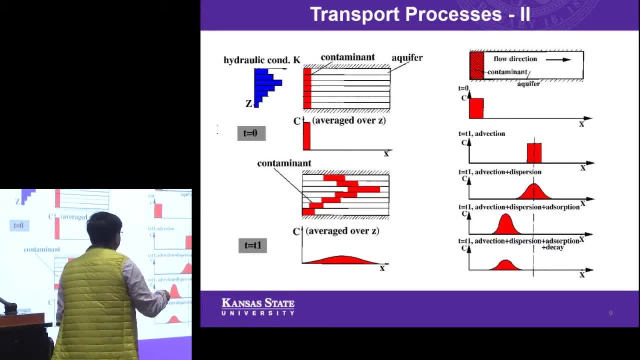 Maybe it may not reach that much of a concentration, but it might disperse into the both the directions. While adsorption is added to it. it slows down, hence the movement is much less, or the x distance is much less, but it might have a higher concentration. 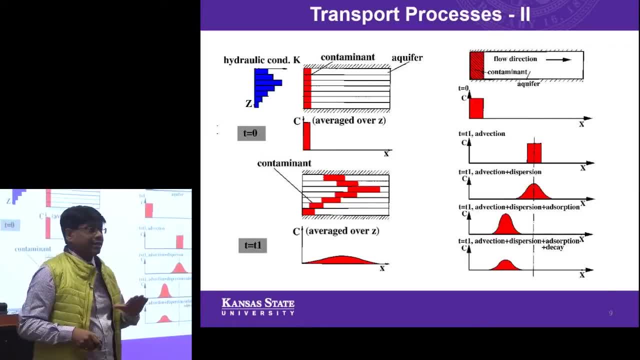 And when decay is attached to it, there will be a decrease in the concentration as the metal proceeds to move along with the plume of water. So these are some of the phases by which a heavy metal or a metalloid moves in the water systems. 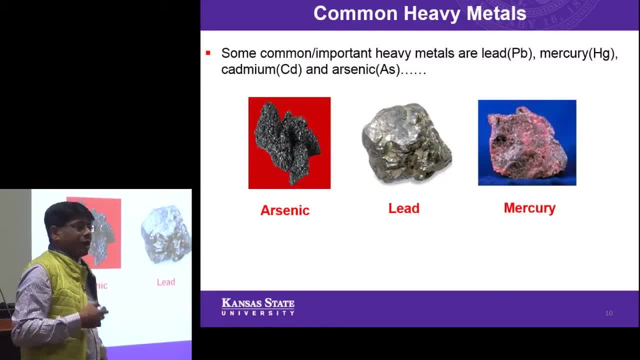 Some of the common heavy metals to come from the processes part, So you might have heard some of them, most of them rather, You know: lead, mercury, cadmium, arsenic. These are some of the heavy metals that we are concerned about in nature. 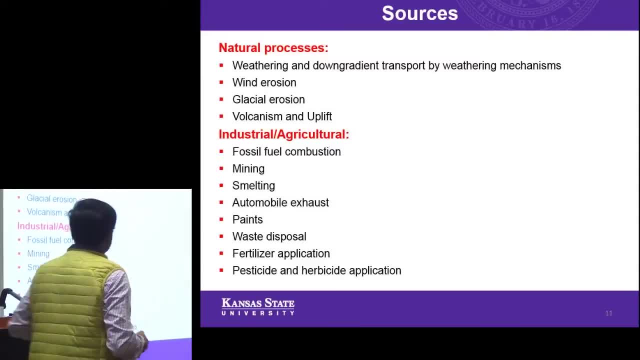 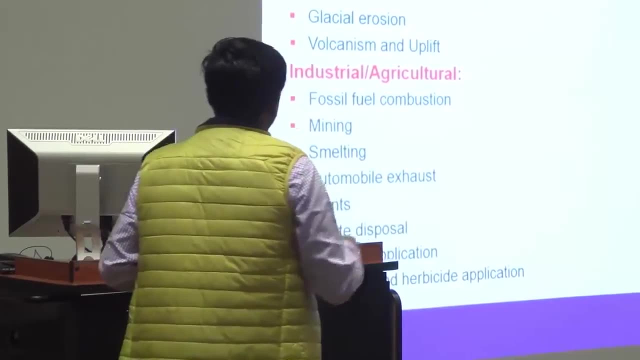 So a very brief outline of the sources of these contaminants, of these metals, for example, A major part is a natural process, Because of the process of weathering down gradient transport by the rivers or by other weathering agents Like wind, glacier, or even by volcanology. 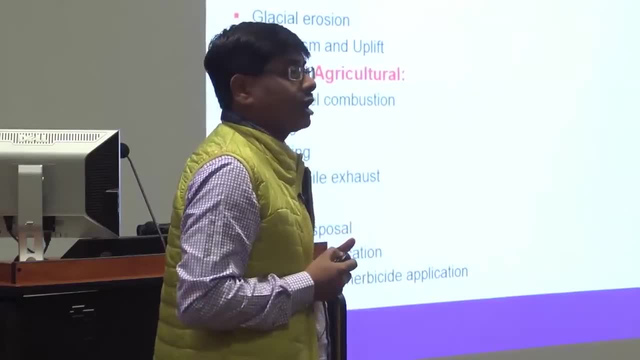 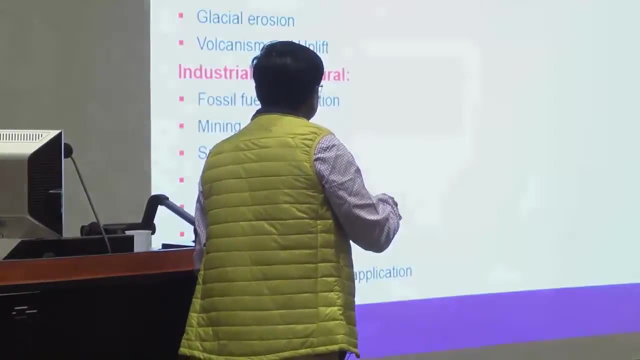 So it is a natural addition of metals in the environment because of volcanism and uplift or tectonics. Now we don't- I don't have to say too much about the industrial and agricultural or the human influence. You might be already exposed to that. there are so many of such sources, are there? 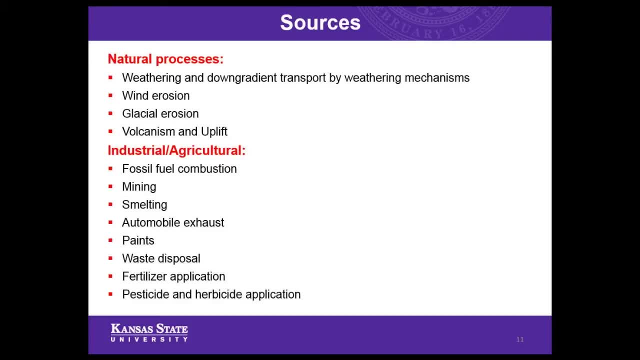 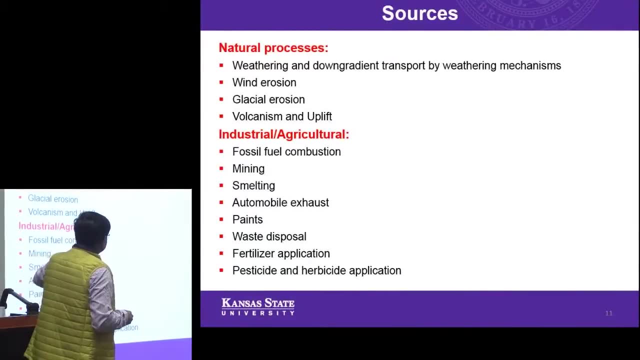 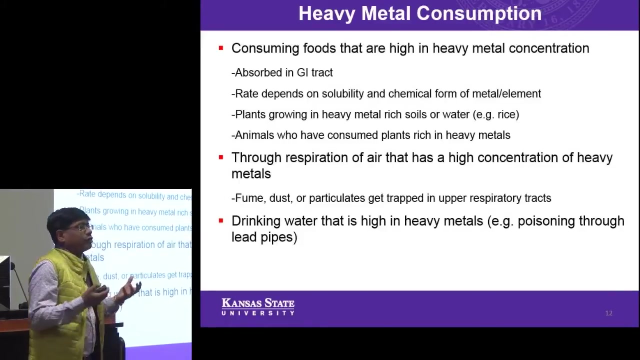 Starting from, you know, fossil fuel burning to application of pesticide and herbicides to your agricultural land. So there are many such, I would say Much vast exposure of the heavy metals from the, from the anthropogenic sources. Now, if that is the case, we might want to think about that. where is the process of consumption coming in, or how are we going to consume this heavy metals? 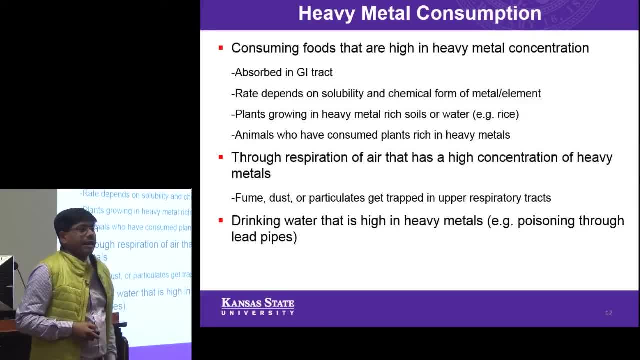 Well, one of the very simple ones is by consuming the foods. Now, usually they are metals- are usually absorbed in the gastrointestinal tracts. The rate at which this move depends on the solubility of these metals And in what chemical form these metals are in. 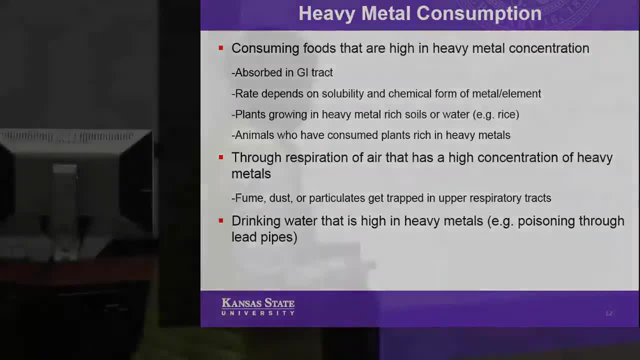 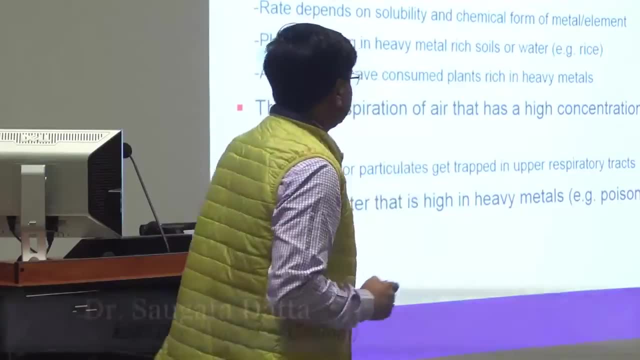 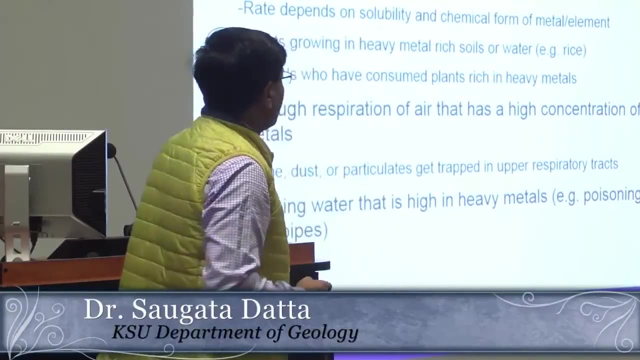 And that takes the speciation point of view also. Plants that are growing this. heavy metal rich soils, for example- and I will give an example of that- is rice That we use as a staple food. Animals can actually consume this plant, which are rich in heavy metals and that can also enhance with the help of bioaccumulation. 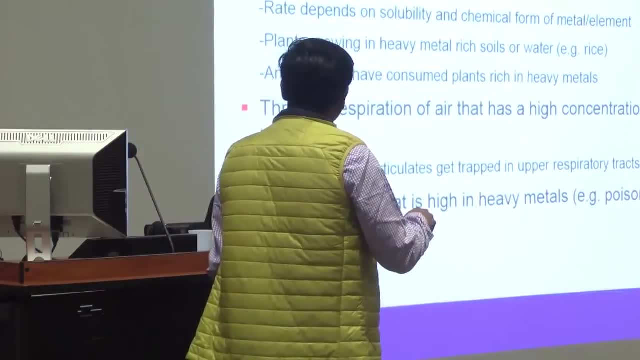 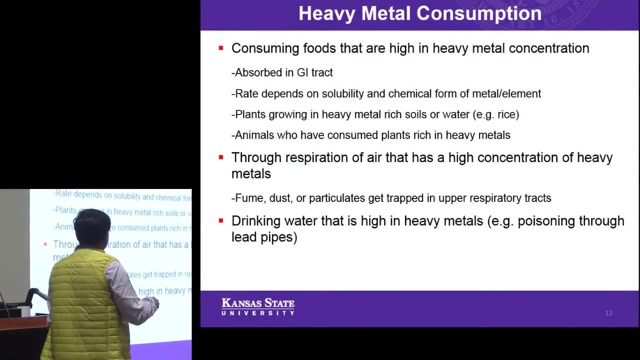 That happens with mercury, for example, in a water system. Now another pathway is respiration By air inhalation, Now by means of fumes or dust or small particulates, usually less than 2.5 micron fractions. These are the ones which are trapped in the upper respiratory tracts. 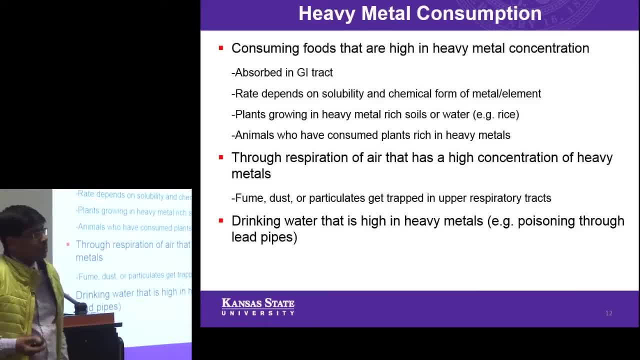 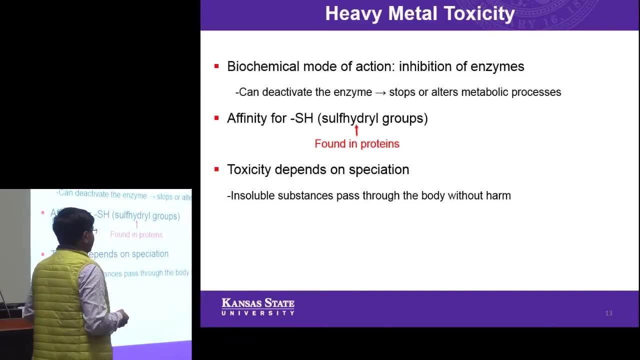 Now, drinking water as such is the most, one of the most important pathways of the ingestion of the heavy metals, And one of the examples is by the lead pipes. So the toxicity, if you want to little bit more clarify Inside the organism, rather there are. mostly they are associated with the biochemical mode of action. 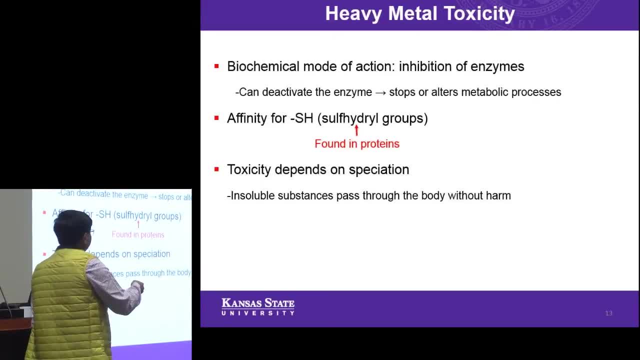 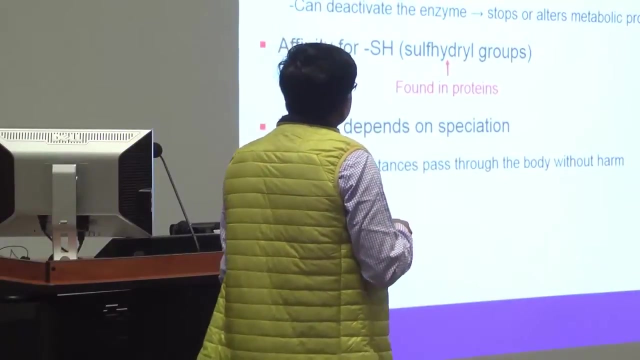 And by means of that what I mean is by inhibiting a plethora of the enzymes That are actually being affected. Now, what you happen is that you deactivate the enzyme and by that they stop or alter some of the major metabolic processes. Now, metals have a heavy. metals have a very high susceptibility, or rather affinity, to the sulfohydride groups. 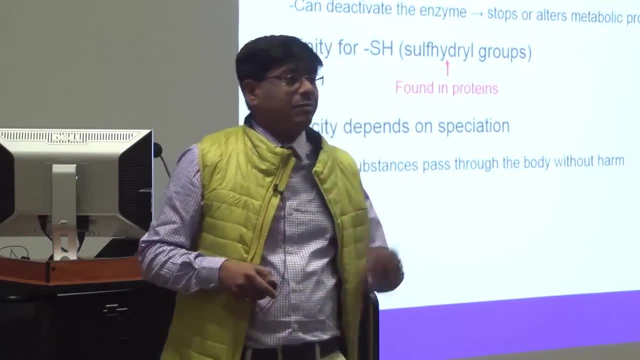 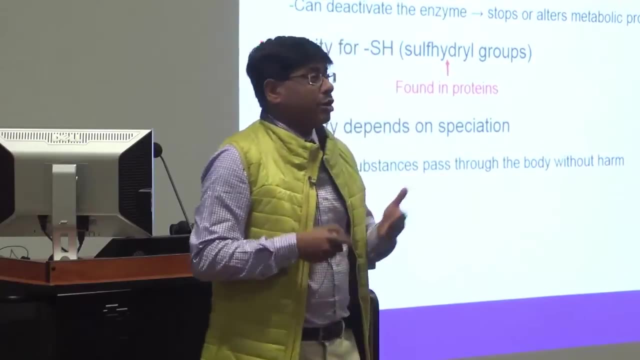 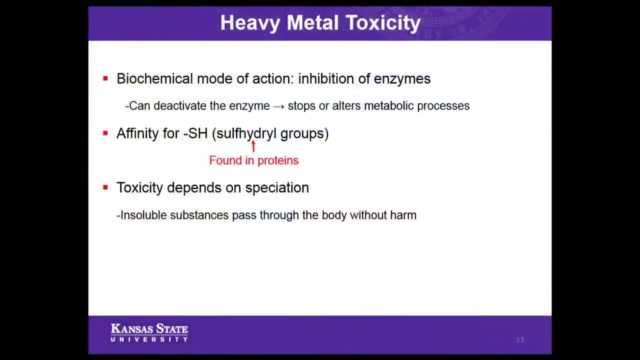 So the sulfur and hydride groups together, And they are the basic blocks of formation of proteins. So protein bound metals are very common within the animal tissues, for example. But again, as I said, toxicity or formation of the sulfur hydride groups will depend upon the speciation. 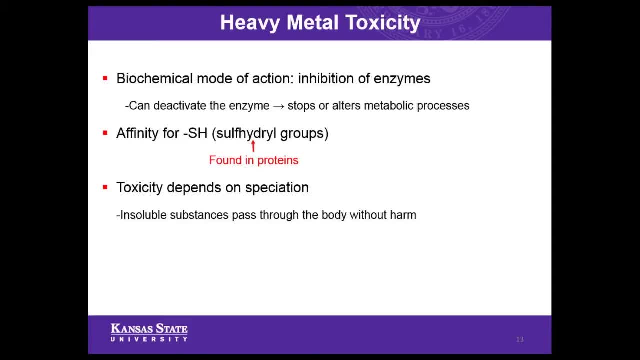 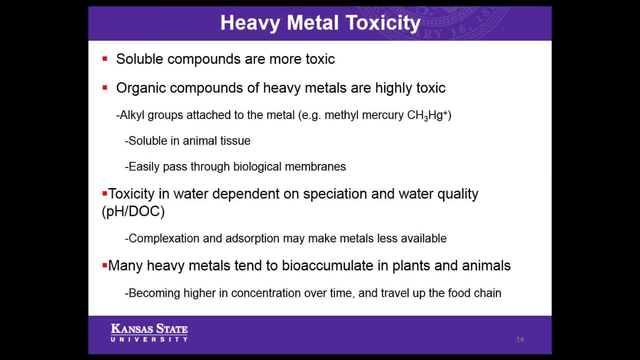 Most of the insoluble substances within the body may pass through the body without any harm. Now, so most of them, most of the toxic ones, have to be soluble. Some are in the form of organic compounds, For example, mercury in the form of methyl mercury. 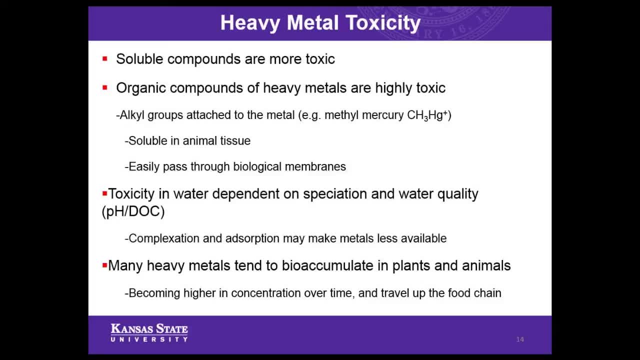 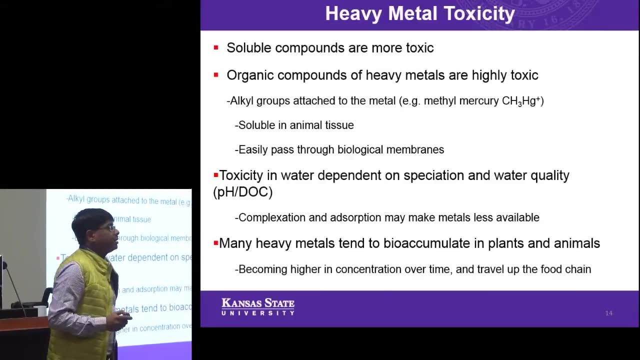 It is an organic bound. they are attached to the metal, the organic molecules. They are soluble, as in animal tissue, and they pass through the biological membranes. Now the toxicity in the water depends upon the water quality- also that I did not mention, For example, 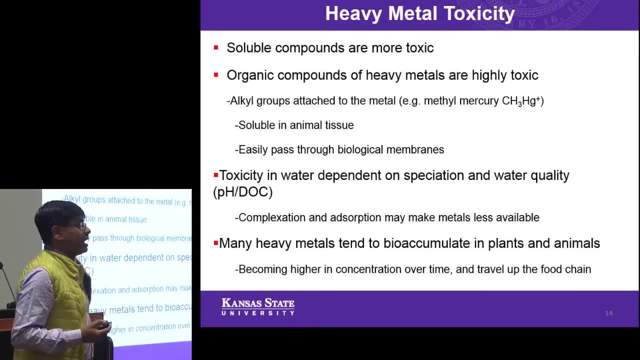 Some of the parameters of water quality that are very important to analyze are, for example, the pH, Or the amount of dissolved organic carbon that is present within the water. I will show you why with one of my, with one of the favorite elements that I am going to talk about. 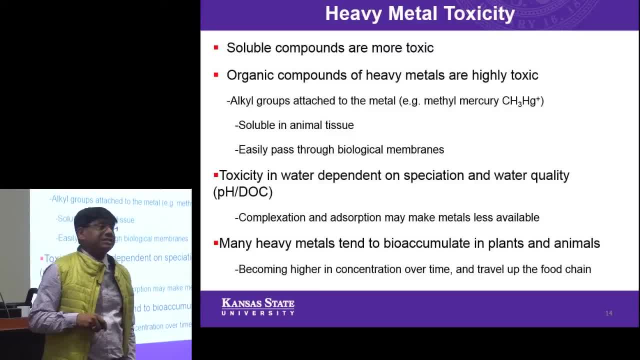 And so the process of complexation and adsorption of these metals are definitely. if you have more of these, then they are less bioavailable. So a process of remediation or bioremediation also comes into play, if we understand this process as well. 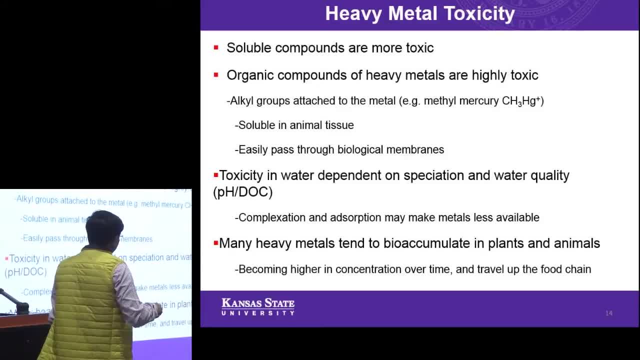 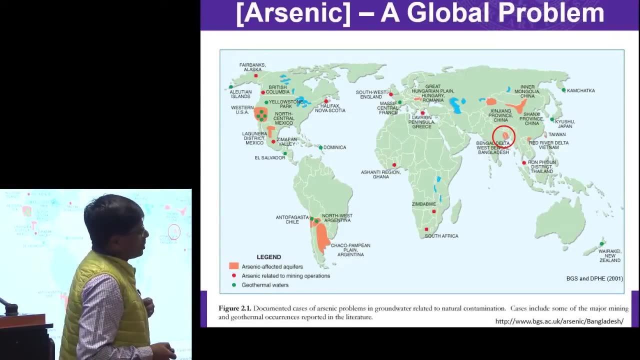 And again, heavy metals can tend to bioaccumulate in plants and animals and become higher in concentration as time proceeds or we travel up the food chain. So we start with one of the examples. in this case, I am starting with arsenic. I term it as it is, a global problem. 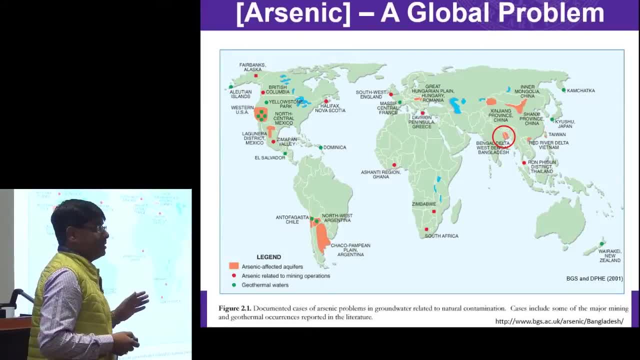 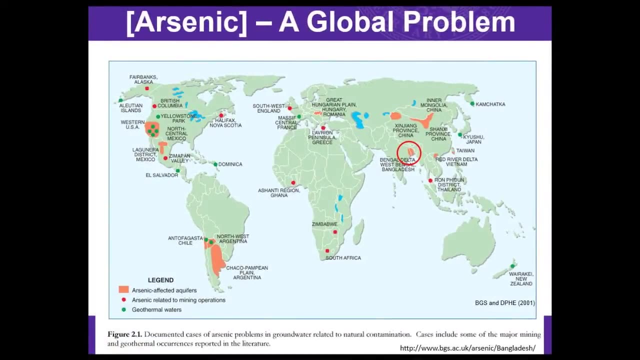 So this is my first element of discussion, which is a heavy metal or a metalloid, Usually is present in water forms and also in sediments in high concentrations to some extent, And you might see from this map- this is a British geological survey map. that was around the 2007-2008 it was produced- 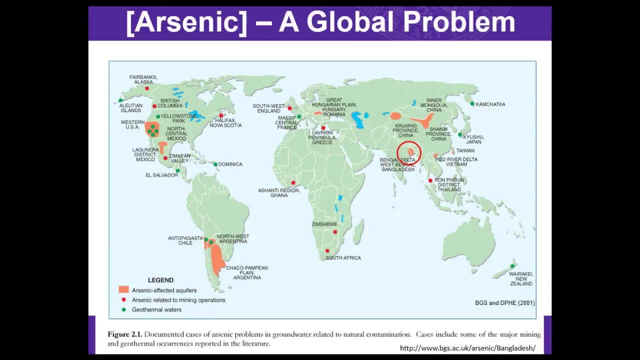 Actually, it shows that some of the sedimentary aquifers, ground water based aquifers, are the maximum polluted arsenic. So this is a global view of arsenic aquifers of the world- Those orange patches that you see, for example, here, a big part of here. these are some of the major aquifers, or sedimentary aquifers. 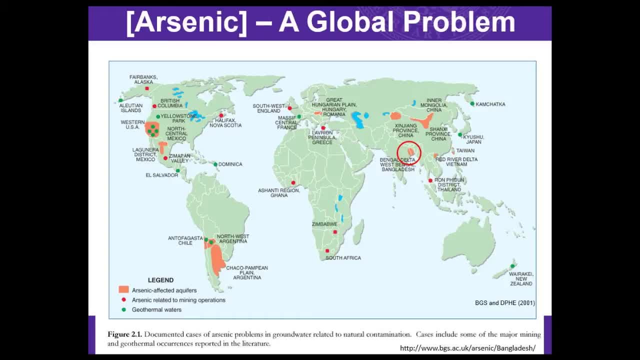 Which are river fed deltaic systems that have high concentrations of arsenic in their drinking water. Arsenic can be also found in mining related operations and then definitely in some of the geothermal waters, But geothermal waters are usually low in concentrations for arsenic. 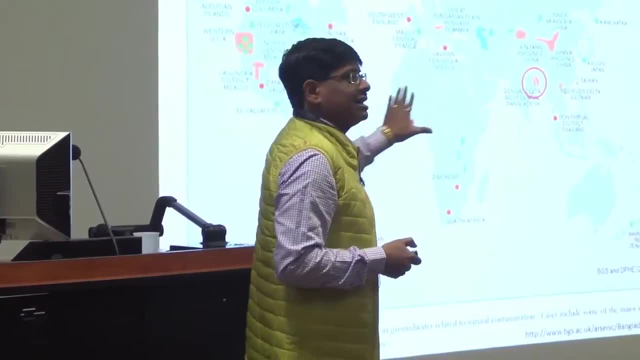 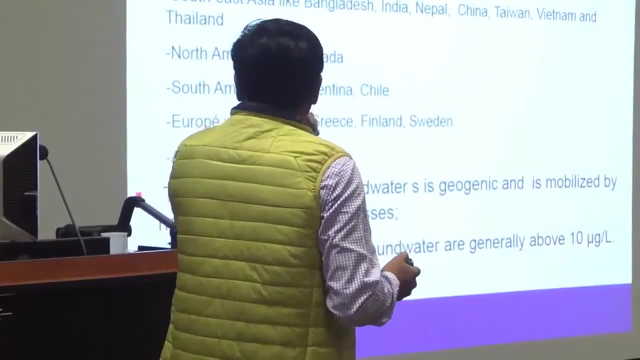 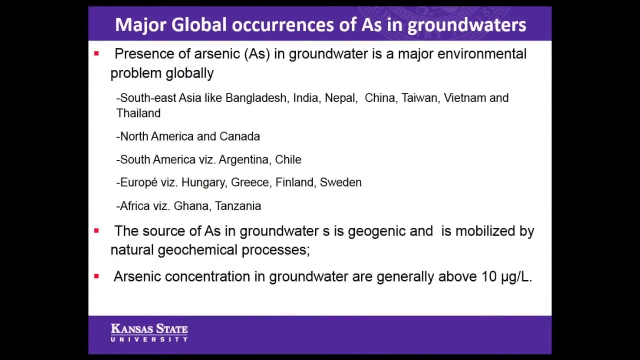 So this is a kind of a global view of where arsenic is in different parts of the world, Just to give you the concept here a little clearer. There are many global problems in various parts of the world, like in Southeast Asia, In countries like Bangladesh, India and even in North America, and I will discuss this in a minute. 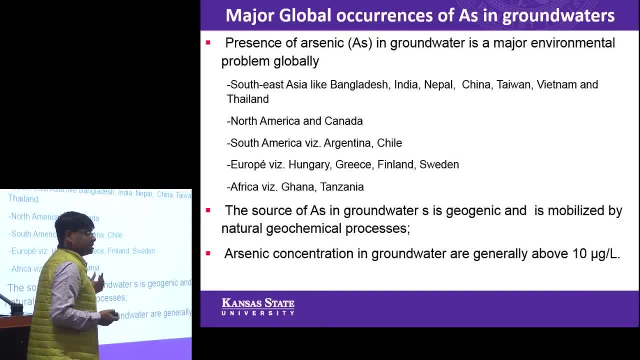 And even in Canada, for example. South America, you saw in Argentina and Chile, Parts of Europe and parts of Asia, Parts of Africa. Now, more and more, we are knowing about the exposure of high arsenic in the drinking waters in certain areas, And the source of the arsenic in the water is mostly here, geogenic. 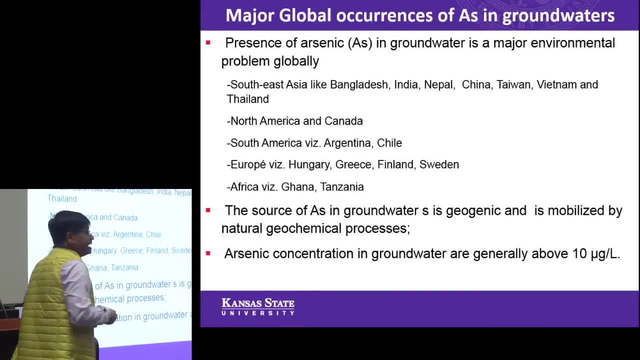 All the processes that I just talked about, And they are mobilized by natural geochemical and biogeochemical processes. And arsenic concentration in ground water is the MCL, or the maximum contaminant limit Is 10 microgram per liter or 10 ppb. 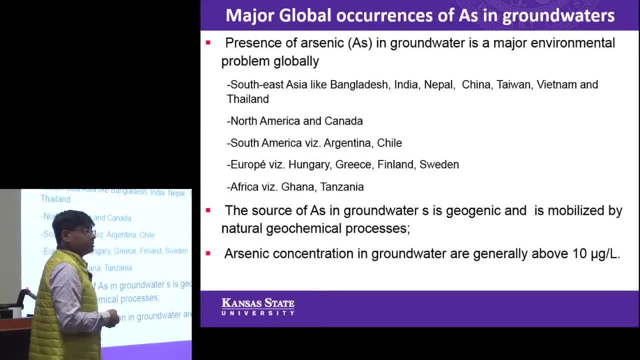 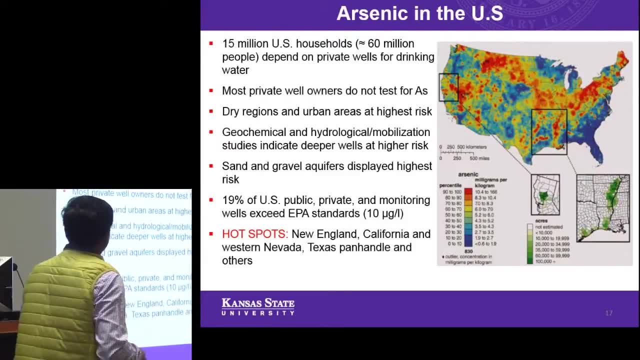 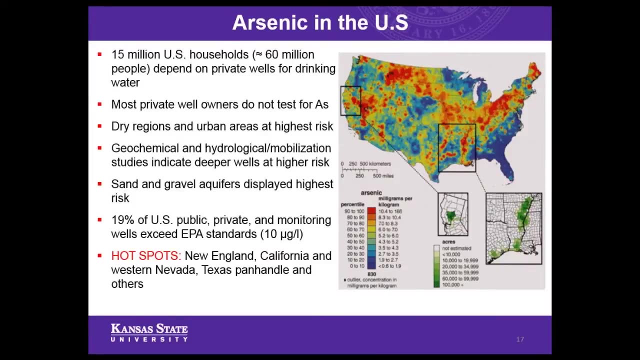 That is said by the World Health Organization or the EPA, and both rather Arsenic. in the US and you might be very interested to know about this. About 15 million US households- This is an USGS database- About 60 million people depend upon the private wells for the drinking waters. 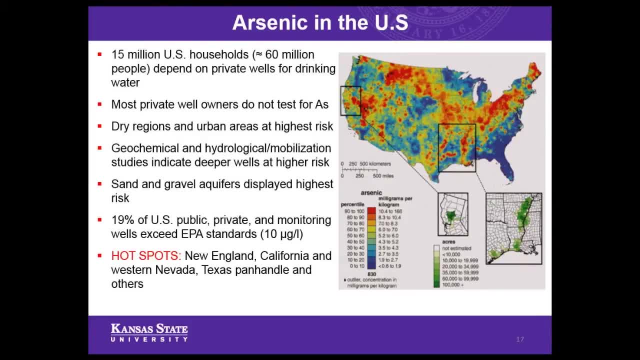 Well, most of the private well owners do not test for arsenic Number one And it varies. the concentration of arsenic in various in waters of US, Mostly concentrated in the dry regions or some of the urban areas. We really need to know the geochemical and the hydrological processes. 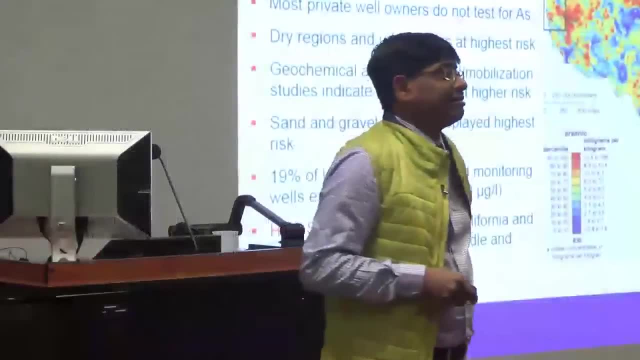 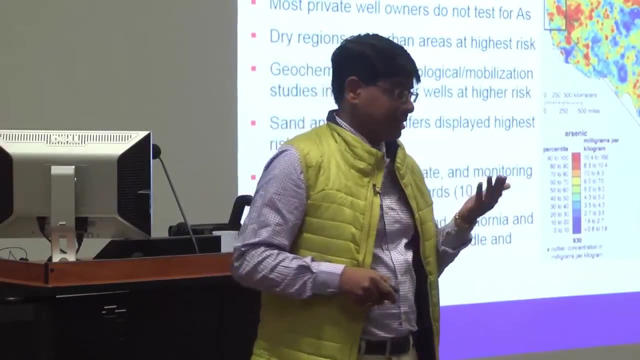 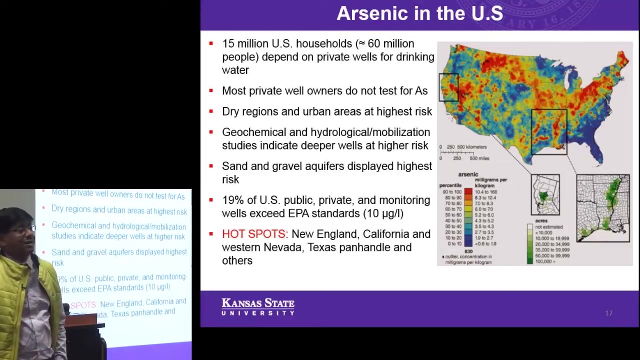 That indicate that maybe the deeper wells might be at higher risk for arsenic. Usually, the sand and gravel aquifers display the highest concentration of arsenic in the sediment phase. 19% of the US public, private and monitoring wells exceed the EPA standard of drinking water for arsenic. 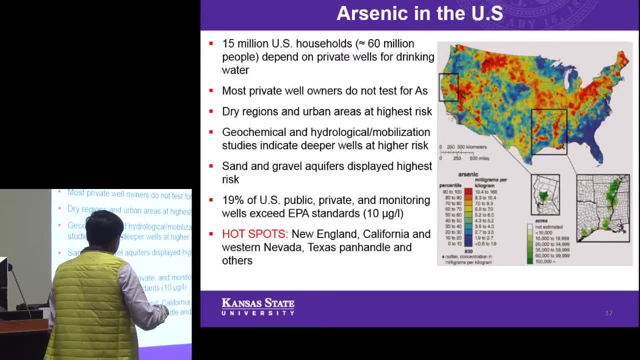 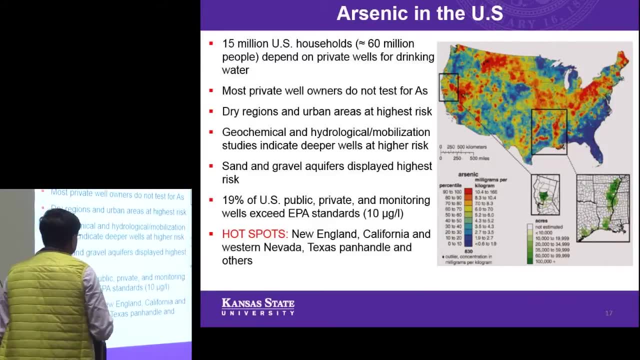 The 10 microgram per liter, And the hot spots are in various locations like in New England, California, Western Nevada and parts of Texas Panhandle. Even in the East Coast have started to find that now. So it is a metalloid. 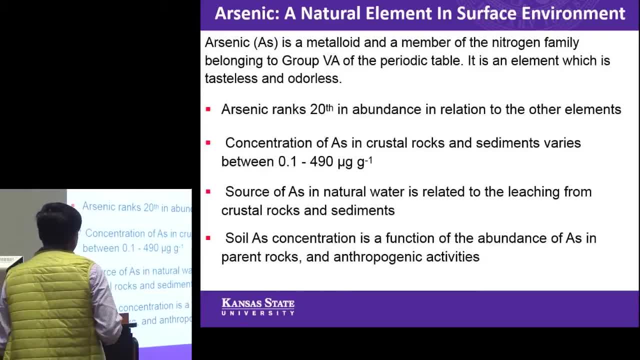 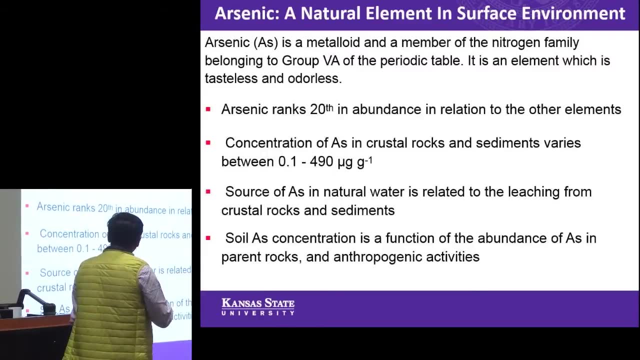 It is in the part of the group 5A family in the periodic table. Actually, arsenic ranks as the 20th most abundant elements in the earth's crust In the rocks. The concentration of arsenic in crustal rocks in the background level can range from about 0.1 to 500 microgram per gram. 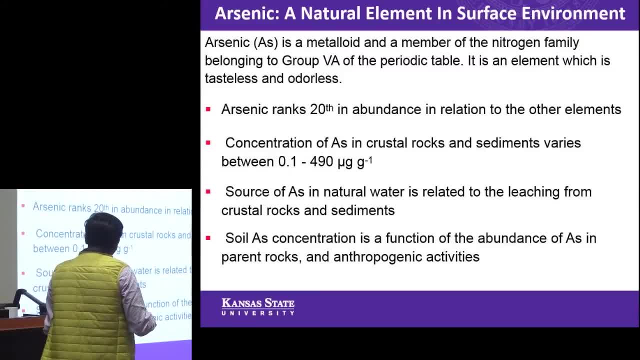 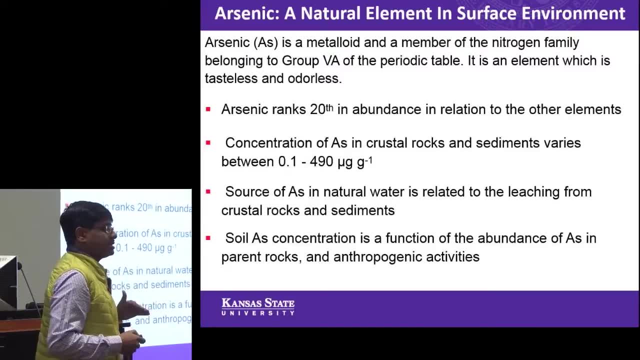 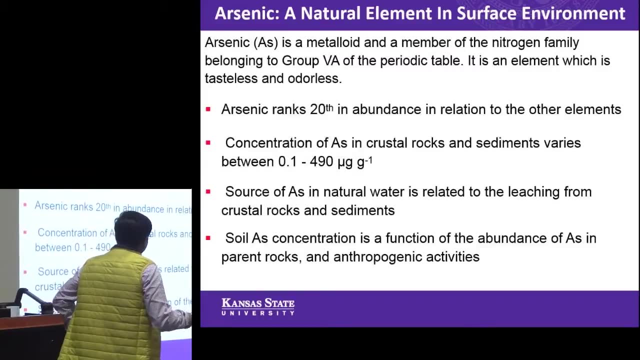 So it is not a high concentration, That much of a high concentration. The source of the arsenic in the natural water is related to the process of leaching of this crustal, rocks and sediments that are enriched in arsenic And soil. arsenic, which is the thin veneer on the top, is a function of an abundance of arsenic that is present in the parent rocks. 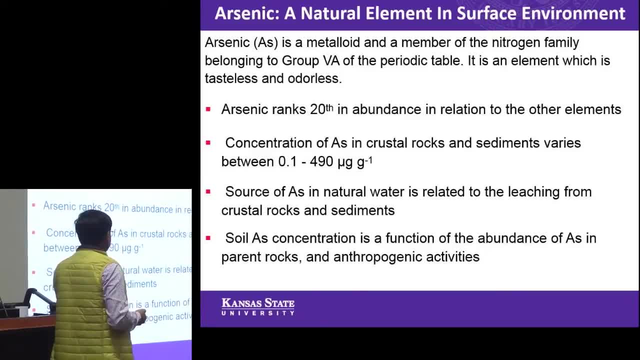 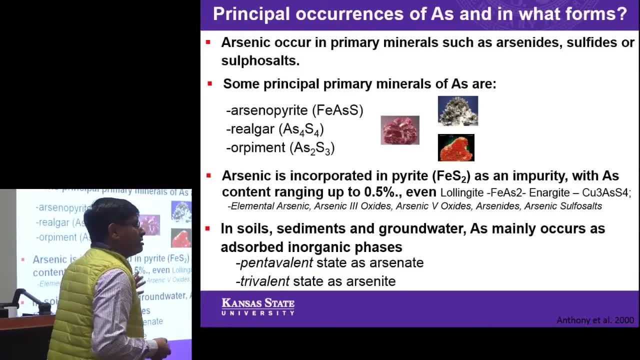 Because it is a weathering product. So wherever the soil is, it depends upon the parent rock from where the soil is being derived. So a very brief understanding of the natural resources. The natural resources for arsenic, for example. Usually they form arsenides or sulphides. 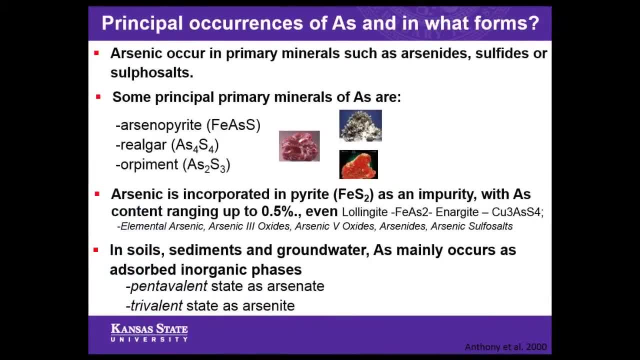 And in sulphosols. We don't have to remember these names of the minerals, But as a geoscientist, we have to at least give you the names of some of the very pretty looking minerals. actually, You might have touched some of them. 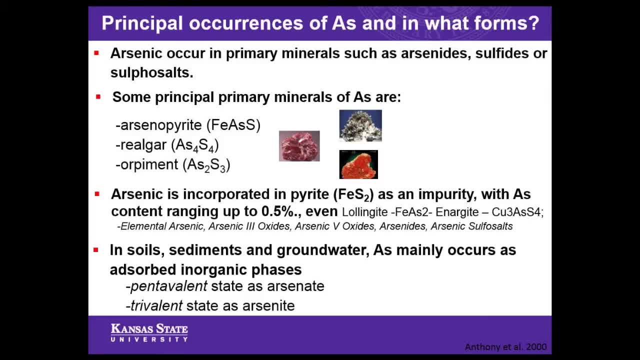 Arsenopyrite, which is an iron arsenic sulphide, Realgar orpiment. these are sulphide bearing arsenic minerals. Arsenic is incorporated in a very common mineral that you might be Knowing is pyrite. It is usually present as an impurity. 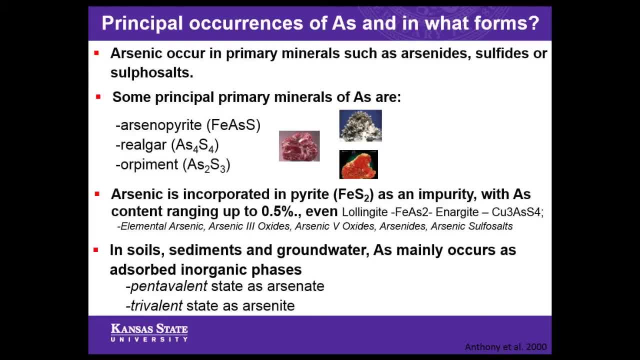 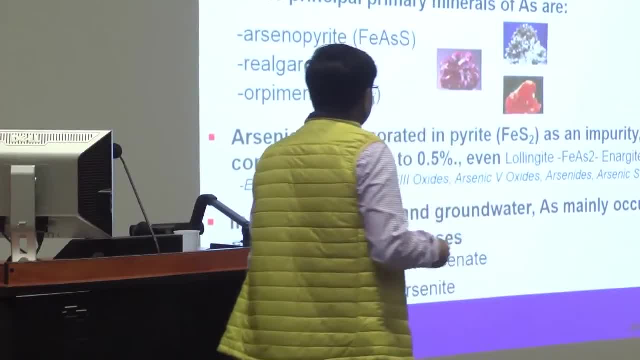 And it can range to about 0.5% of the stoichiometric value for the pyrite mineral In soils and sediments and in ground water. Arsenic usually occurs in two states, as I said, In plus 5 pentavalent or plus 3 trivalent state. 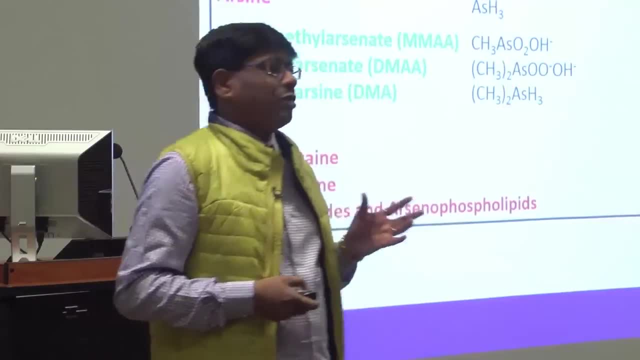 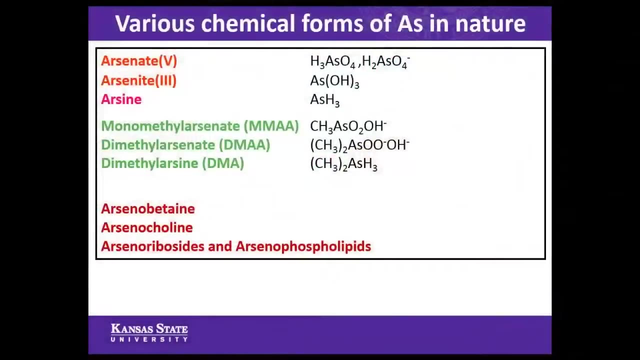 Arsenate or arsenite And the various forms of arsenic in nature, Not just the inorganic phases As a gas, which is arsine gas, Or it is very common in some of the organic complexes to produce to form organic organo arsenic complexes. 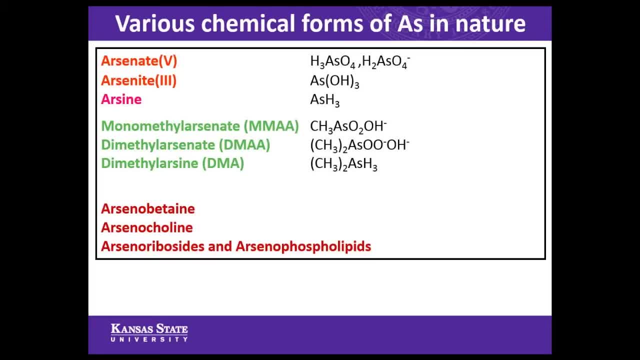 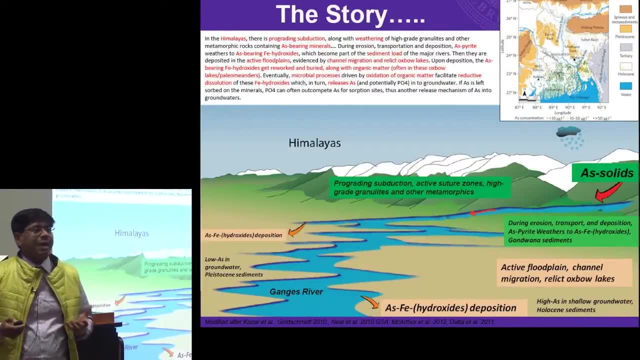 For example, monomethyl arsenate and so on. So these are some of the chemical forms of arsenic in nature. So let's go into the story as to what is really happening for the various metals, And I'm going to give the story for arsenic. 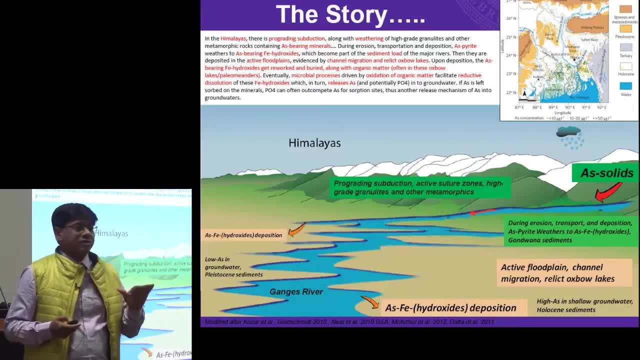 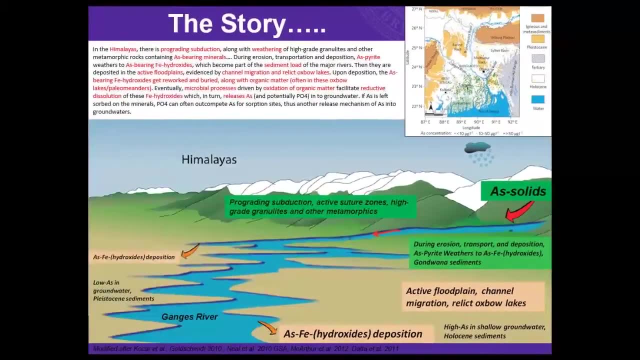 But really this is a story for most of the major elements, Major heavy metals. Usually it starts with heavy erosion or weathering From mostly the mountainous parts Where there is a lot of tectonism going on And processes of subduction or suture formations. 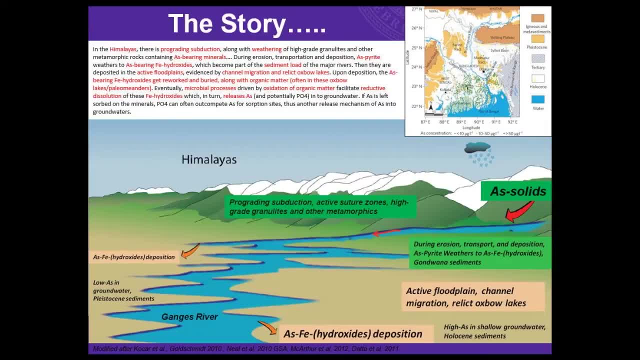 Lot of the metamorphic rocks that are forming. That, from where the erosion actually process, Is usually count down by the river systems or the streams And they flow downwards towards a delta During that process of flow, During process of erosion and transport and then deposition. Certain minerals weather much faster And these minerals, when they weather. One of the complex minerals for hydroxides, or sorry, for the metals, Are iron hydroxides, And this iron hydroxides Are quite common in nature, actually Very high in concentration. 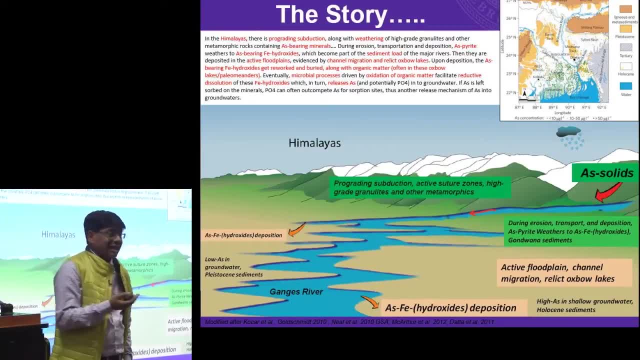 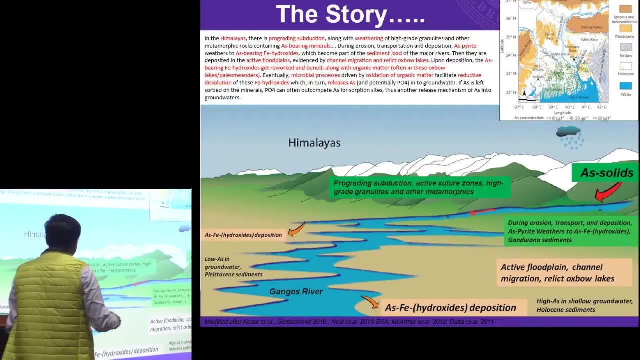 And mostly when the metals flow With these hydroxides, as either adsorbed to those hydroxides Or they're much easily available to the water And in this active plains And active flood plains, rather Because of reworking of the sediments. 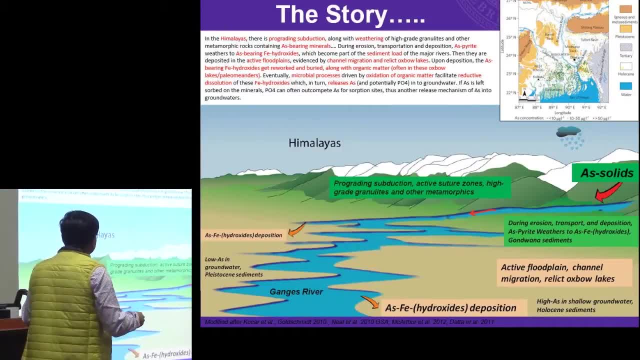 It gets concentrated more and more, So as the river systems flows down, As its velocity decreases, Stream capacity decreases, It just floods the banks. These are the over banks. So some of these heavy metal pollutions naturally Usually might, you might see. 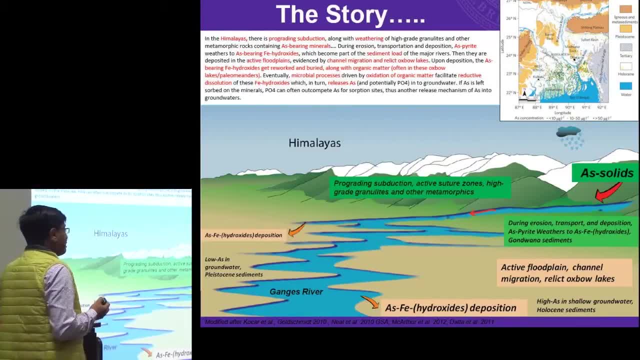 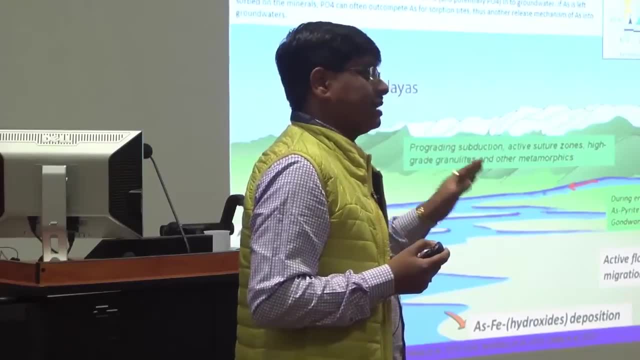 In this fluvial deltaic systems. Arsenic is a classic example of that. In every fluvial deltaic system You might be looking for heavy metals, And one of the ones is arsenic in this case, And you might find that. 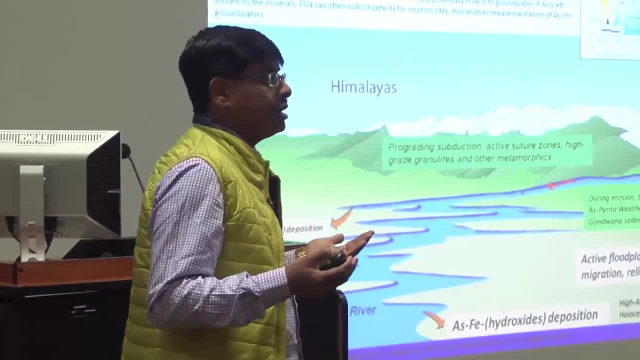 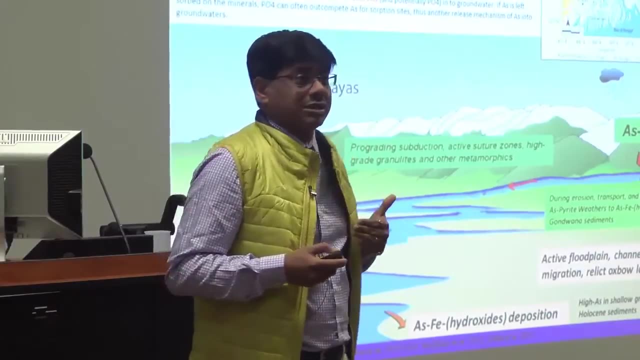 And it actually because the process is quite common. It depends upon the source rocks, But most of the source rocks Usually have common minerals That can have or release arsenic In its transport system. So it is not just the source But also at the same time. 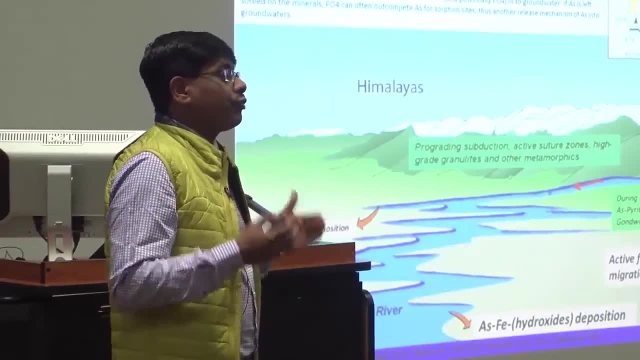 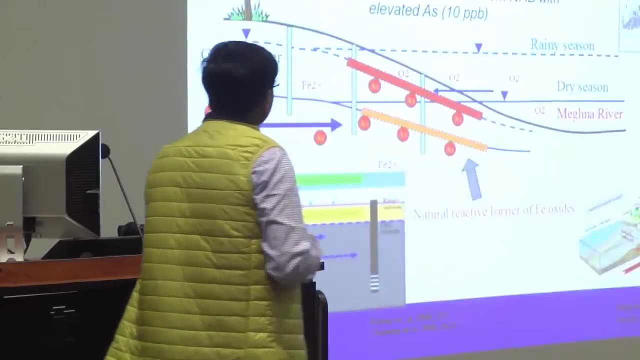 The important theme here Is how these are leached out From the sediments or the rocks, Mostly, in this case, rocks That are degrading down to the sediments. Okay, So a little bit more into the Structure of the process. 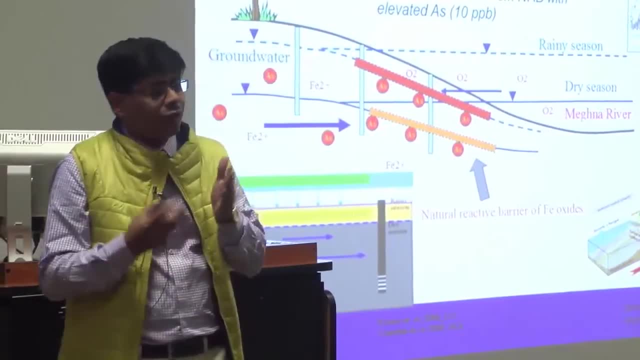 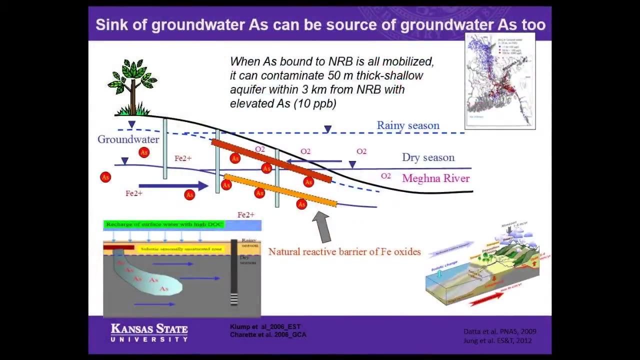 And how these metals form. Again, I am citing an example of arsenic, But it is for most of the metals. in this case, What happens when a river system- Actually when ground water Comes in very close Association with the rivers- It actually disposes of the water into the? 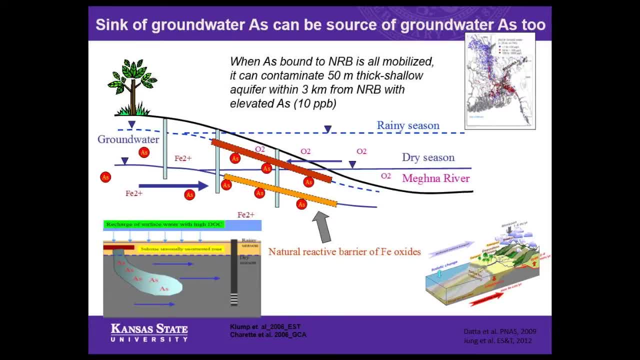 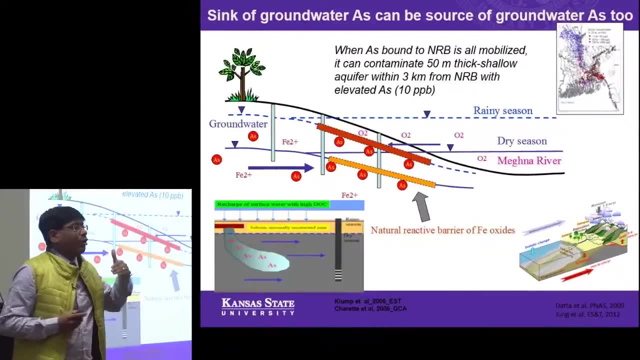 Or it can be both ways: Into the river, or the river water can In filter into the ground water, Into the aquifer, This transect process. Usually there are what we call these barriers, And these barriers Are natural reactive barriers. 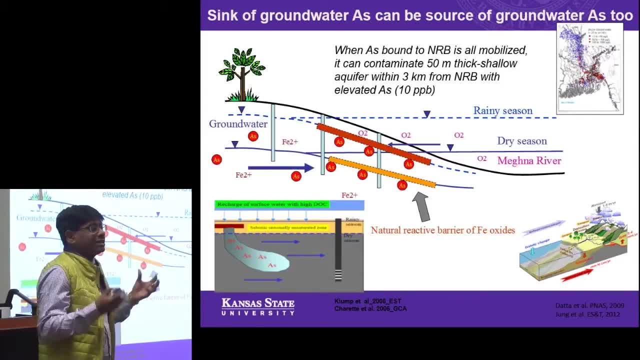 Where maximum of these metals are mobilized In a much higher rate Than anywhere else. So you need A right cocktail picture To make them mobilize. It has to come down from a source. It has to be reworked quite a bit. 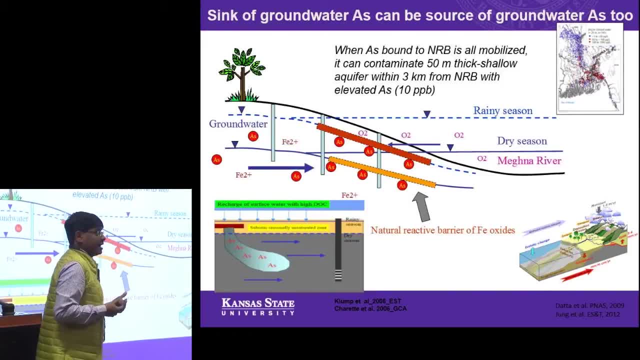 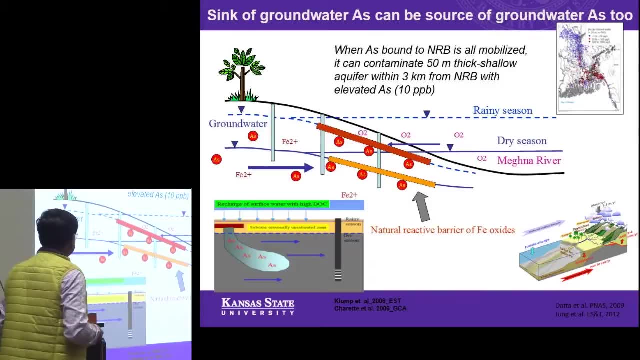 It needs a barrier to stop the flow And then it will just concentrate back into the aquifer. So these are like step wise processes That you have to follow To understand How these are actually getting accentuated. One of the ways to do that. 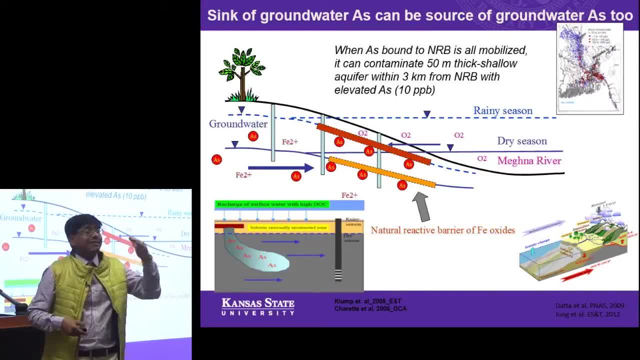 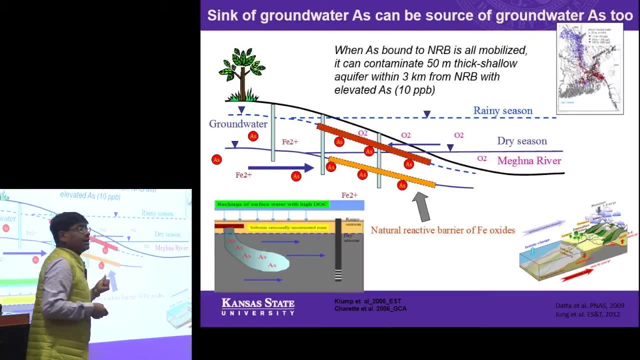 And one of the main, One of the important things Is the seasonal variability In the water systems. for these metals or metalloids It actually varies quite a bit, So you have a lot of information That you have to gather. You know how frequent the rainfall is happening there. 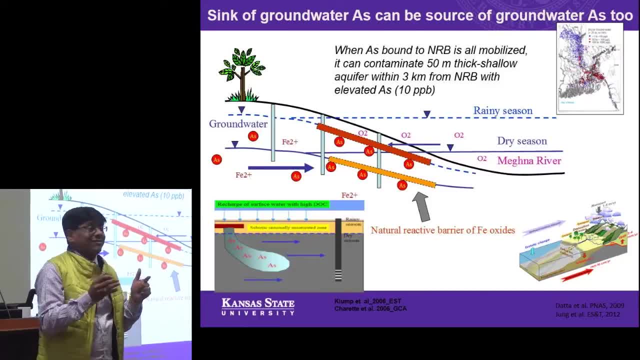 How frequent evaporate Or how much is the rate of the evaporation there? So this classic interface of the hydrologic cycle That I just mentioned In earlier part of the talk Is actually very important to understand How these metals mobilize. 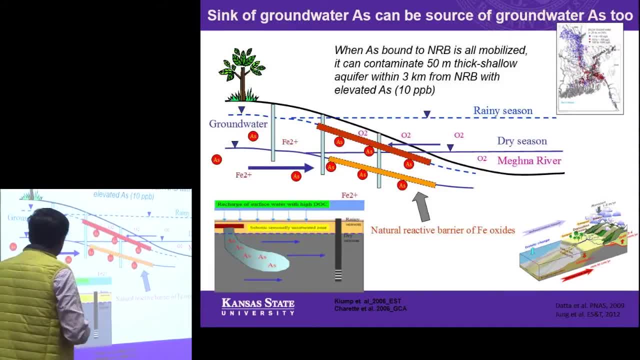 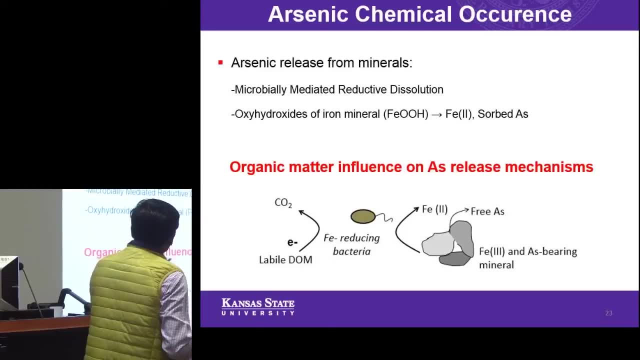 Goes into a well, You pump the well And you get a contaminated water. Okay, so, with that in mind, The chemical occurrence of arsenic, In this case a little bit more, Is that they are. We usually need a microbial mediation there. 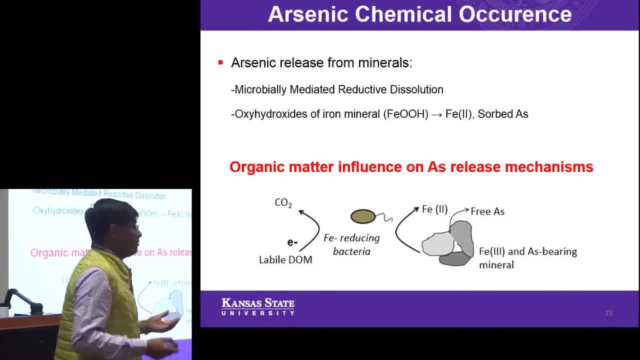 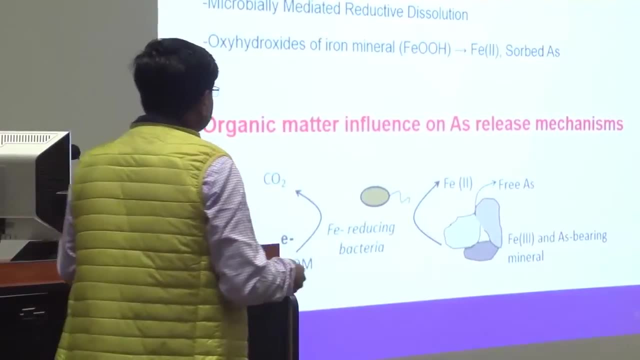 Without the microbes, Nothing gets really released quite fast. So the very, You know, classic way of defining this: as We have dissolved organic matter, It releases electrons And because of the release of electrons In the presence of bacteria or organisms, It releases the metals from the substrates. 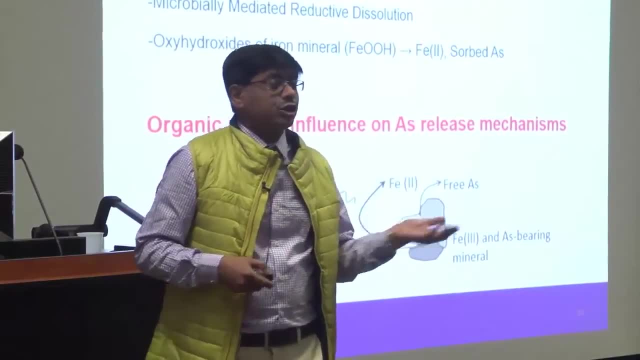 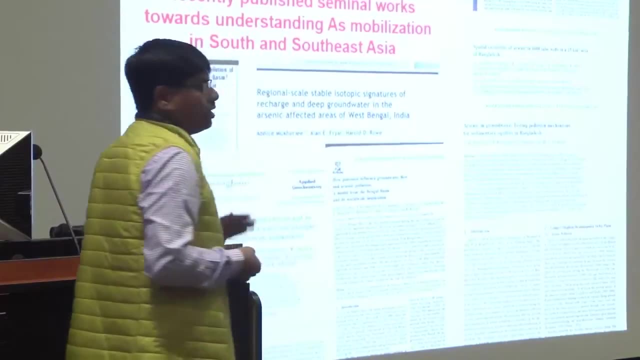 And the free arsenic goes into the water. So- and this is for arsenic, But this is for most of the metals That we know of- There are a plethora of publications That are being made in the last few years If you go into the science citation index. 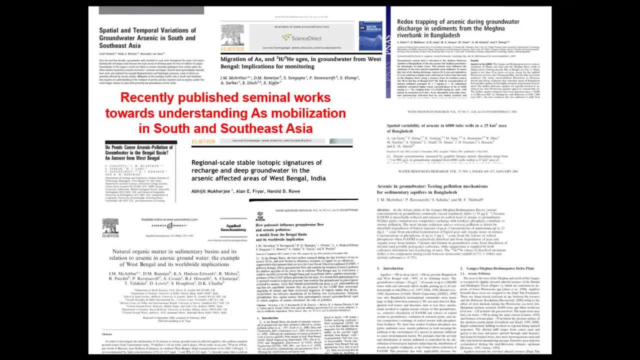 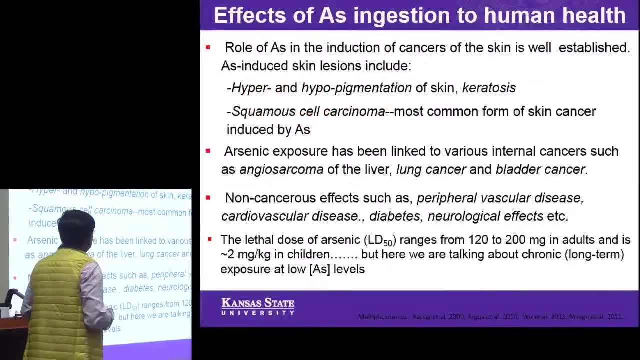 I think if you type in arsenic, You might just get an overload of Almost like 40,000 publications In the last 5 to 10 years only. So it's a huge information That is there for us to understand. 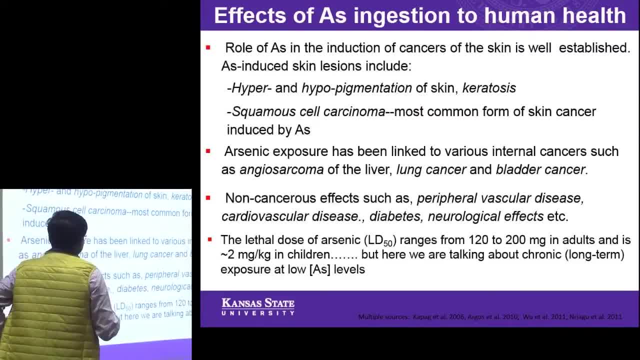 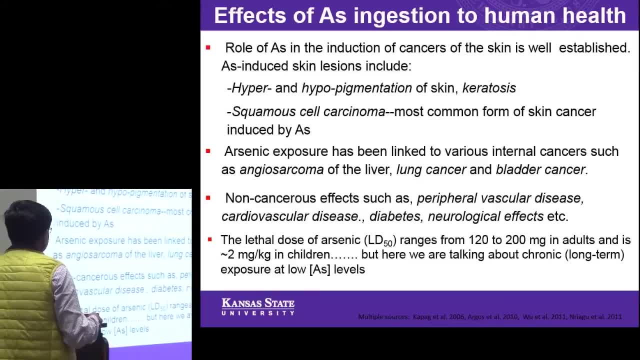 Why is arsenic so important? Very quickly, It's because of its health impact. It causes the skin cancer. Hypo and hyperpigmentation. Also the roughness of the skin, Which is keratosis- It causes the skin cancer. 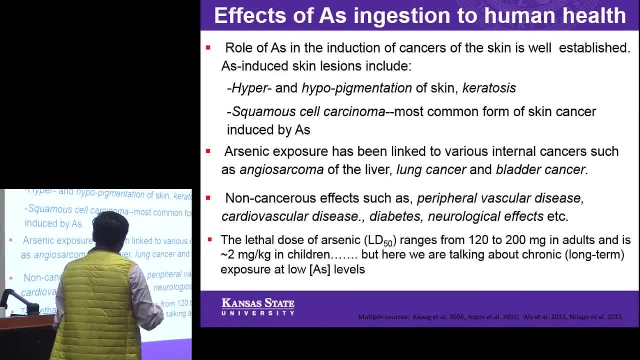 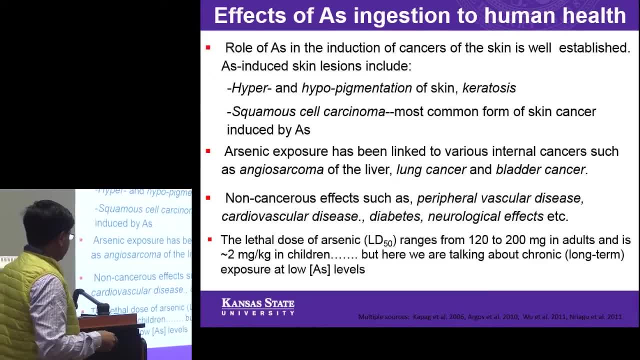 It causes the skin cancer. It causes the skin cancer, But then again, internally It's linked to many cancers In the different organs, Like liver, lung or even bladder. There are some non-cancerous effects also, Like vascular diseases. 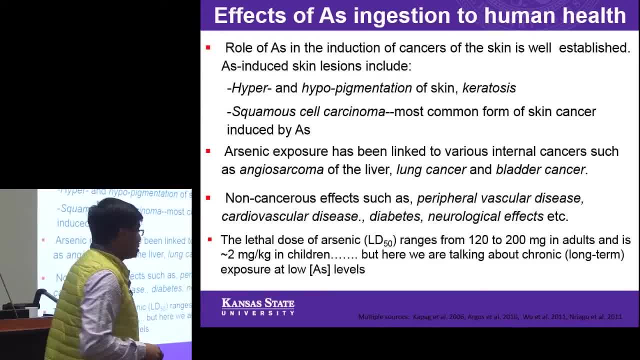 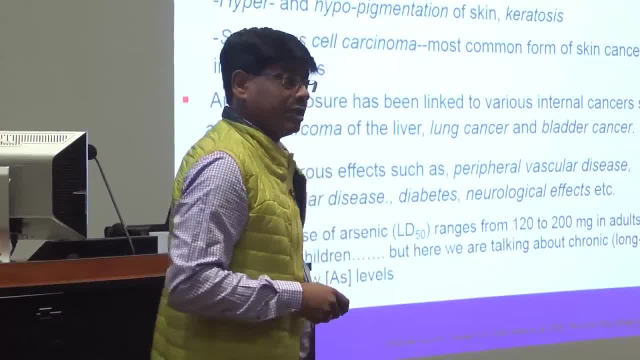 Or even diabetes, is linked to that. The lethal dose of arsenic, The LD50 dose, Is from 120 to 200 milligram in adults, While for children It's 100 milligram per kilogram Within the children. But the point here is that 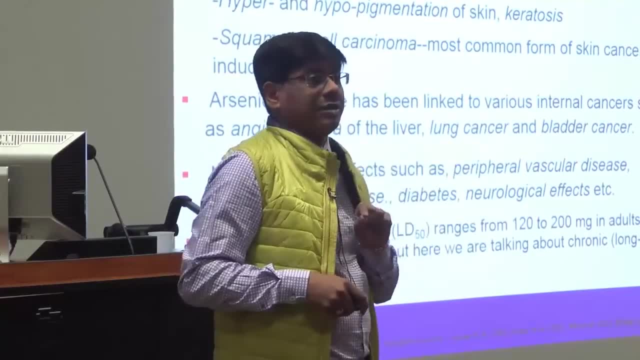 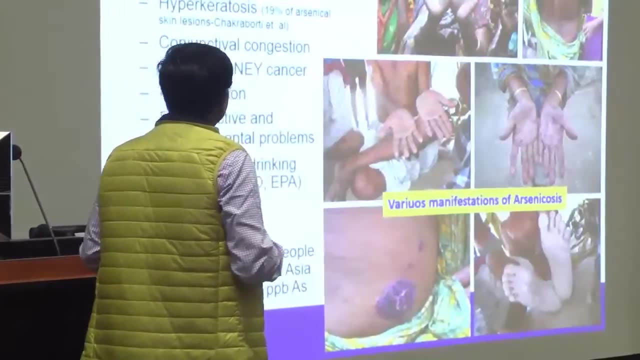 About the chronic or the long term exposure Of this low level of arsenic, Which is very important to understand. What is the time frame you are exposing That person to a low level of arsenic? This is just a very quick overview. 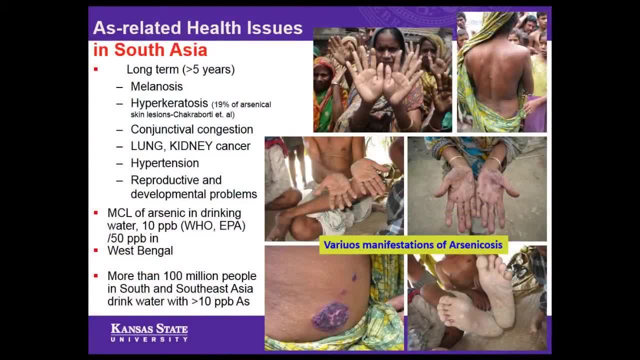 Of some of the scales of works That we have done. This is some parts in India That people have been affected With the problems that I just said From arsenic. So the safe drinking water limit of arsenic Is 10 by WHO. 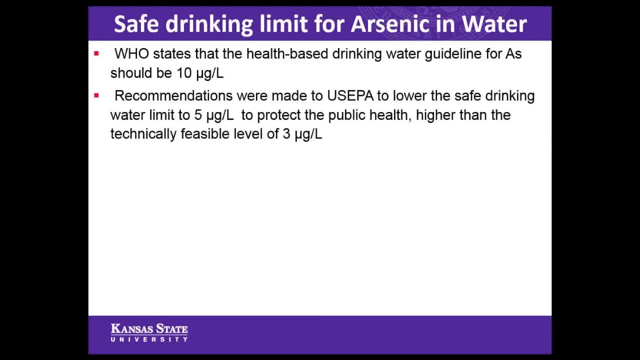 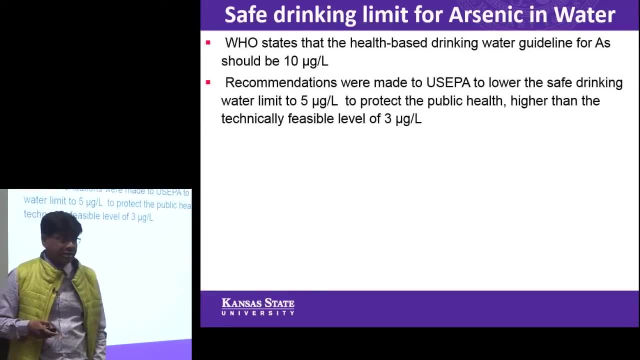 US EPA actually is thinking about Getting it down to 5.. Even at times, maybe to 3.. And this is not just an environmental issue. This becomes a geopolitical issue. Right If my well now is exposed To 5 microgram per liter of arsenic? 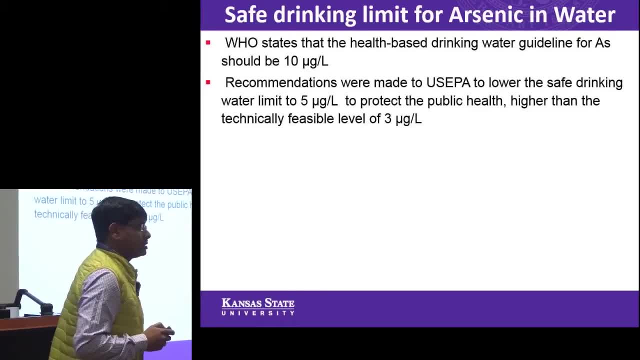 First of all, let me tell you one thing: We have pretty state of the art equipments To analyze arsenic in a dissolved form In the water To up to about 1 microgram per liter. So it is possible. But as we go down the ladder, 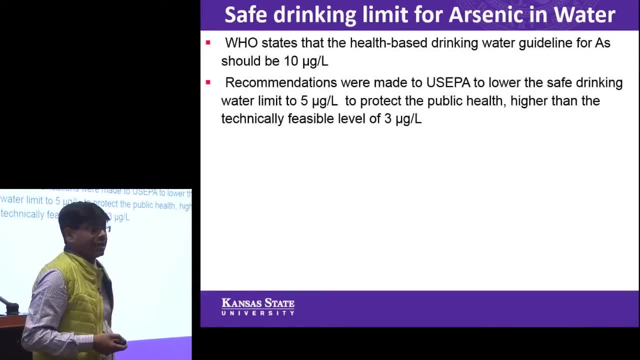 Usually it is much tougher to Make a precise measurement of that arsenic, But 10- that level is easily Possible with high Like mass specs and so on. So EPA is thinking about that In 2002.. It actually came down from 50 to 10.. 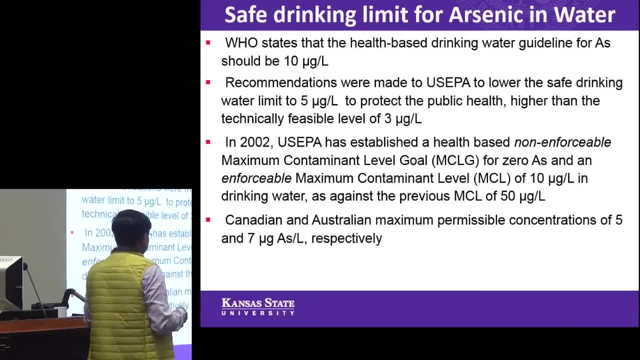 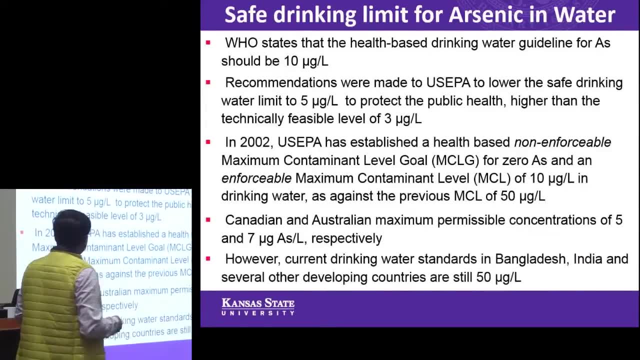 And then Canadian and Australian maximum Permissible limits are 5 and 7. Some parts of Europe actually has 3 microgram per liter- Germany for example- But still if you go to the places Where there is a maximum problem of arsenic. 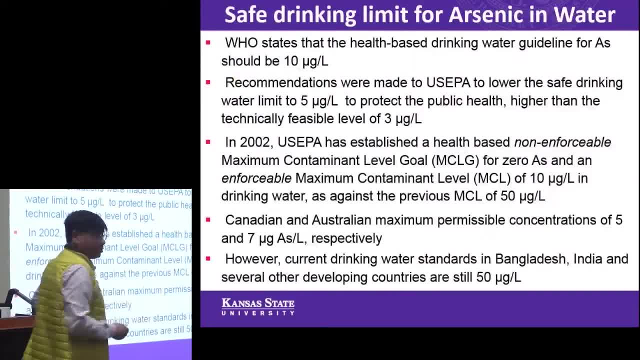 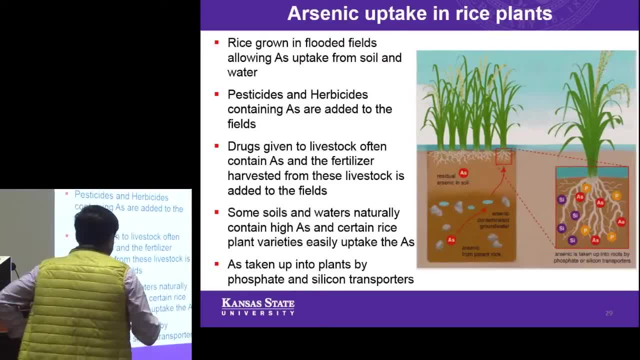 Still because of geopolitical issues. They are still at that, 50 microgram per liter of arsenic. So from there, as I was mentioning, Just not the water. Rice is also a problem. Rice is grown in flooded fields. This flooded, this flooding water. 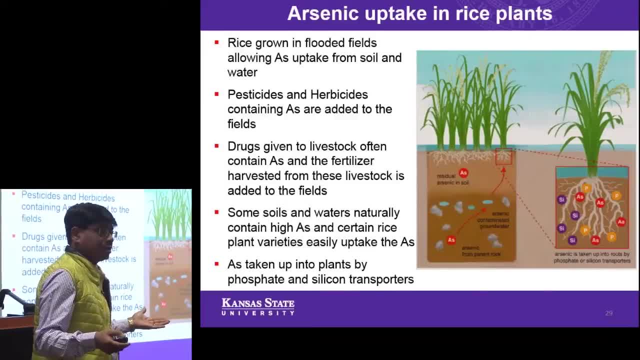 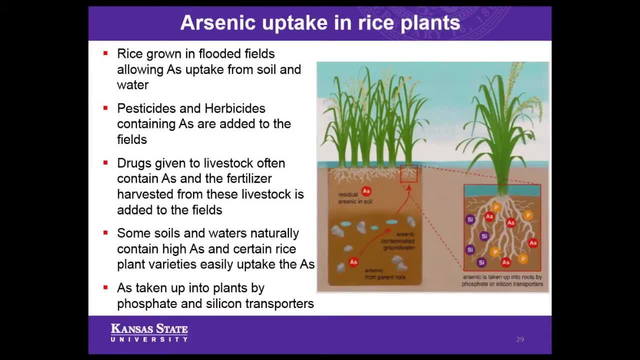 Is essentially high in arsenic too, Because these are irrigated waters. So it's like a double whammy, Because you are really Not only just you are getting it from the water, But the water that you are using to irrigate the land. 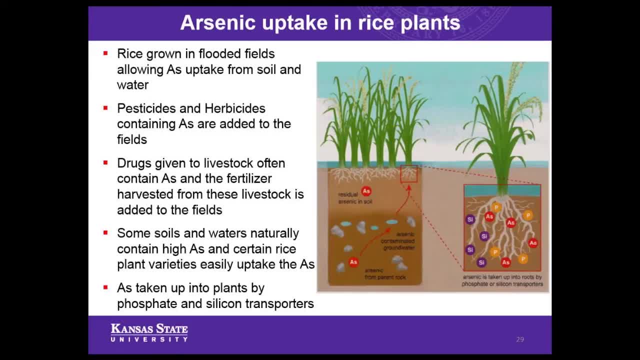 Is going into the plants, Or rather the plant is up taking that water, So it has both. You know pathways, Definitely. we know about pesticides and herbicides That contain arsenic. You know different drugs Are being given to the livestock. 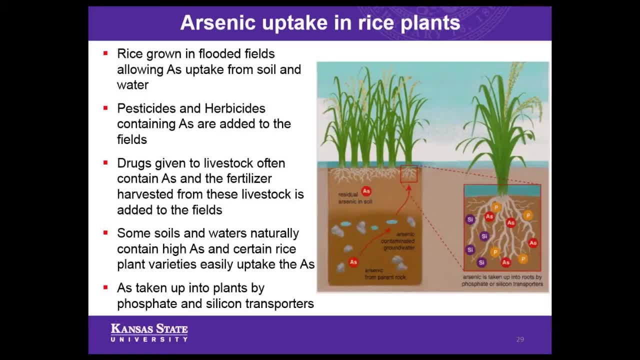 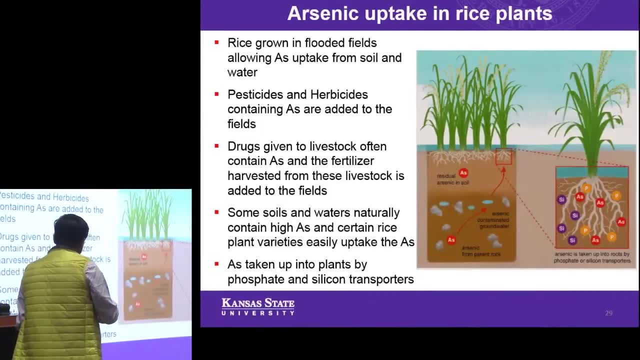 And some soils and waters Naturally contain high arsenic And certain rice varieties Usually up take more arsenic than the others. Arsenic is up taken by Phosphates and silicon transporters. So when we look for arsenic, 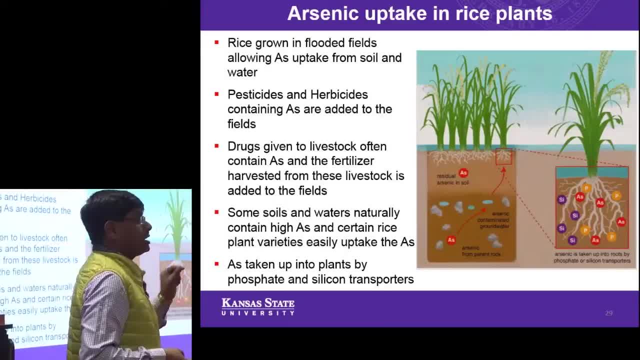 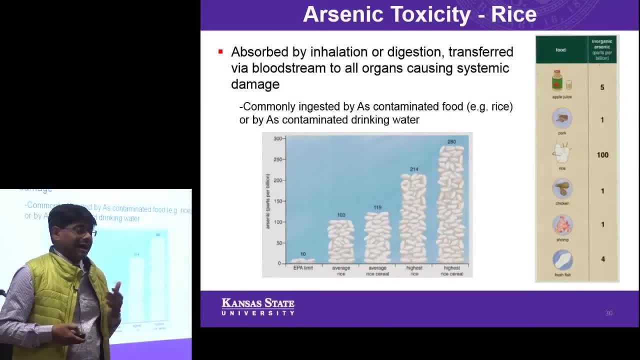 We look for silicon and Phosphate transporters To understand the mechanism Of how arsenic is up taken by these plants. Arsenic is absorbed by rice And, by the way, You might have heard that In the very recent literature by FDA. 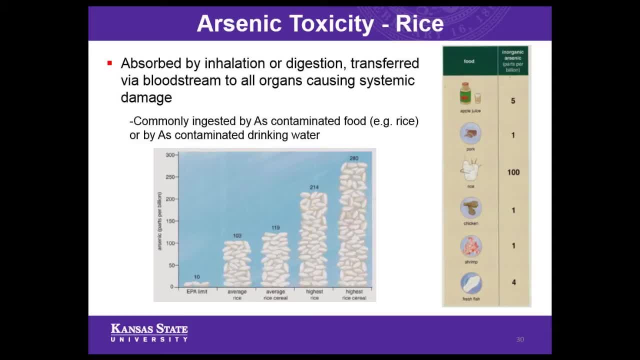 They have been actually regulating A lot of the food grains that we are eating, In this case rice, And food products like rice products Are having, are showing high concentrations of arsenic in it. Now, this is still are very debatable And I wouldn't say it's a controversial. 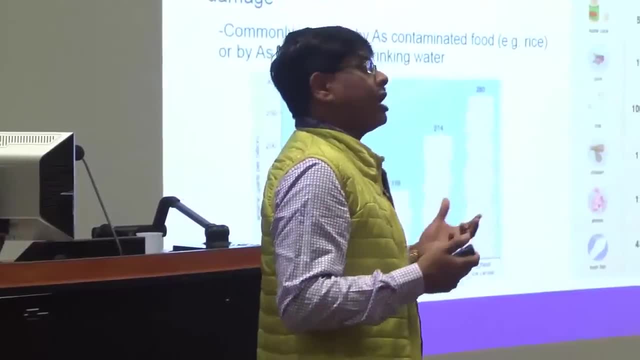 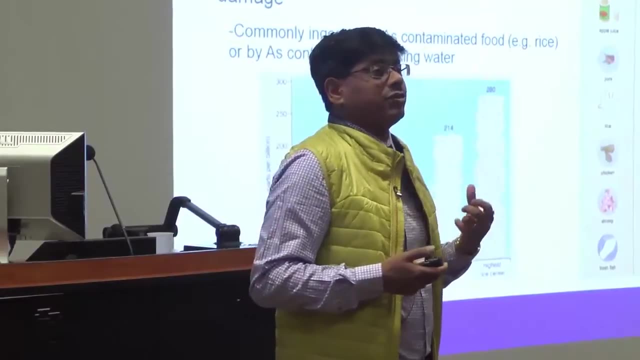 But it was controversial at some point If you go back five years. But more and more research is coming up As to say that you know what is my. What is the proportion of arsenic? We know about water, But what is the proportion of arsenic in rice that is safe? 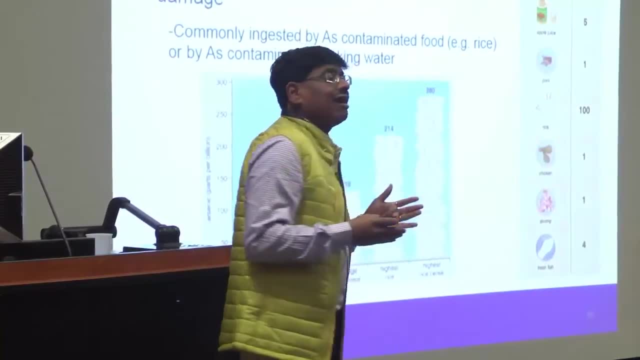 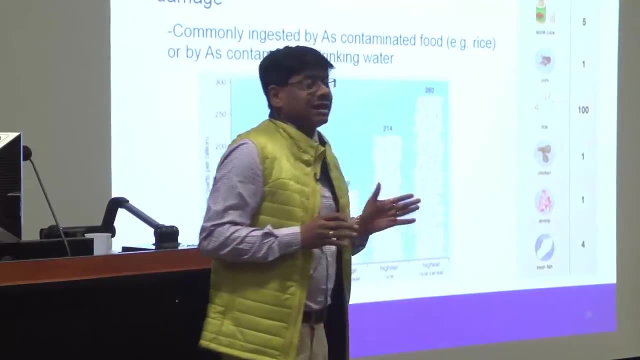 Or which is unsafe. Again, I would say that, rather than going into a pinpoint level, I think it is safe to say that If you, if you are, if you are knowing, If you are interested in that You, you might be able to understand. 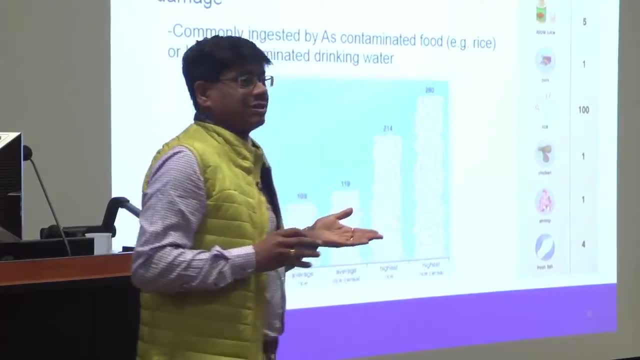 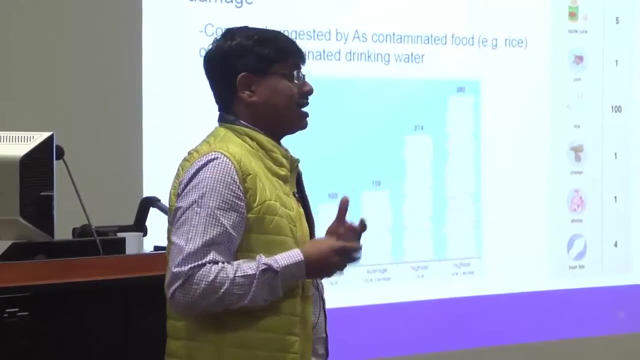 That why some of the rice. We have done a lot of work recently On different types of rice, like brown rice versus white rice, Husks of rice versus the grain of the rice, And there are different ways the arsenic gets Accumulated in these parts. 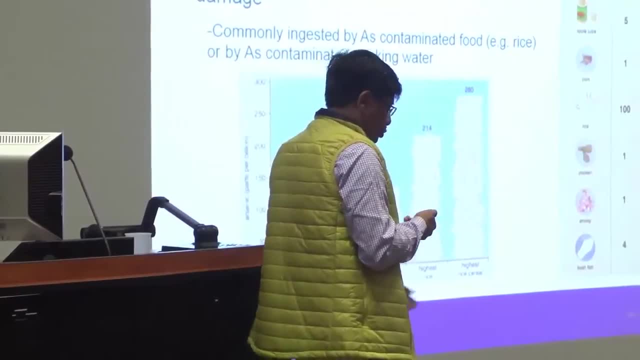 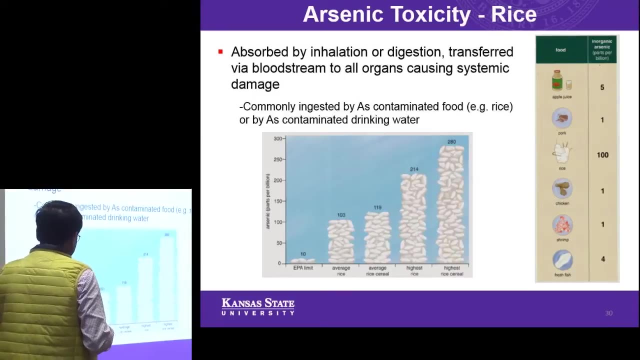 So a lot of work needs to be done. Just to show you the brief idea That you know some of the natural, You might know the cereals that are Getting exposed to arsenic. also, There is a current, Very just a week back. 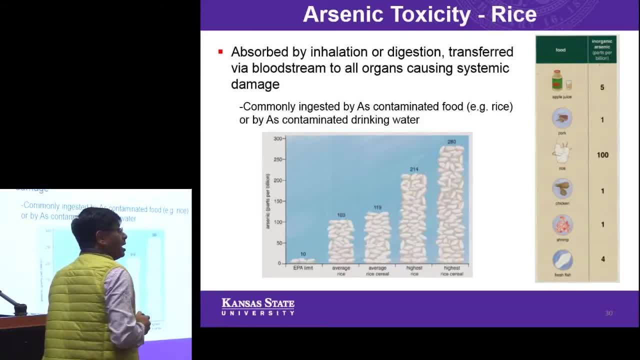 They were showing that in California Some of the cheap wines Are having high concentrations of of arsenic Because of the of the It comes in the water And actually it's the some of the herbicides they're using. Some of the plants are taking up more arsenic. 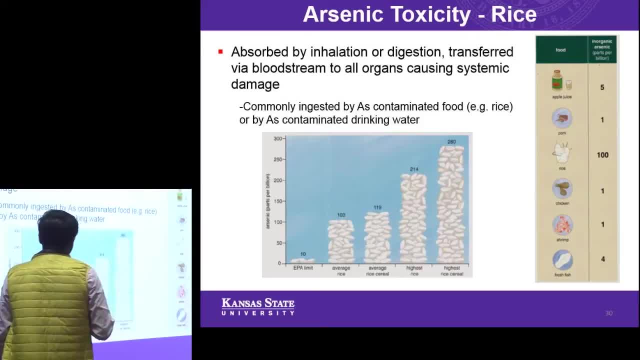 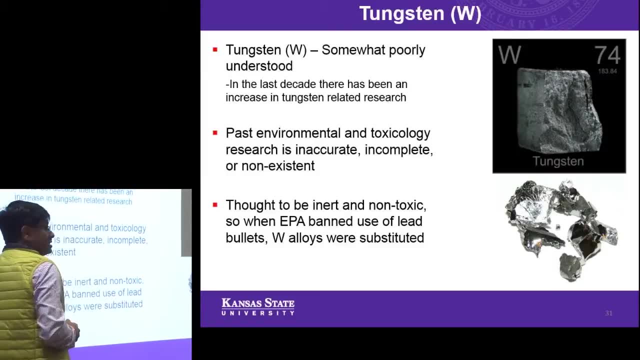 Than the others, And that's where the wine is produced from. So there is a lot to understand. Another element, Just to give a very brief overview, Is tungsten, And you know you might have heard a little bit more about Arsenic before, but tungsten is coming into the picture. 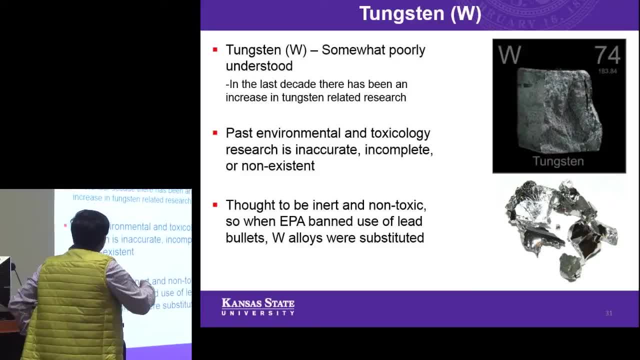 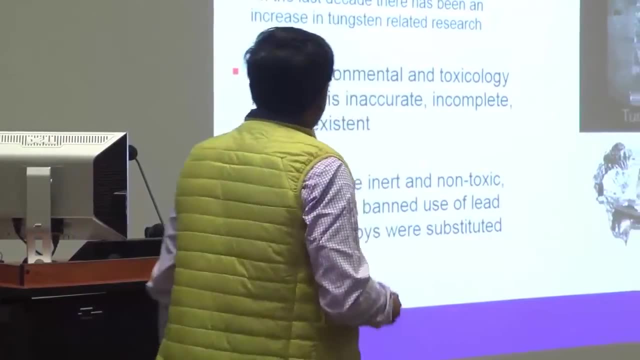 A little bit more, Because tungsten is very poorly understood. In the last decade There has been very minimum tungsten research. Okay, You might think about: Is this element even In nature? I mean this is a strategic metal, But in the past 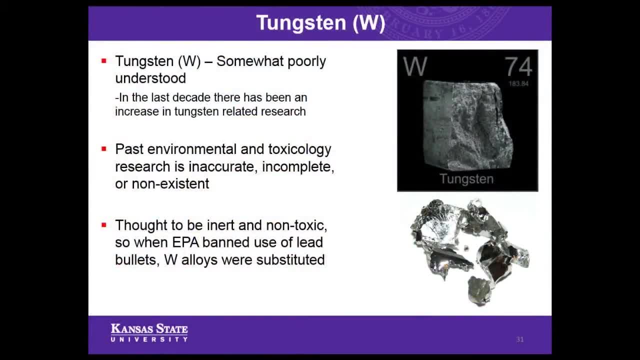 The environmental and toxicology research Is rather inaccurate, Rather incomplete And also non-existent. Actually, EPA before used to think that tungsten Is inert And non-toxic, And it was actually used instead of lead, Which you might know more about. 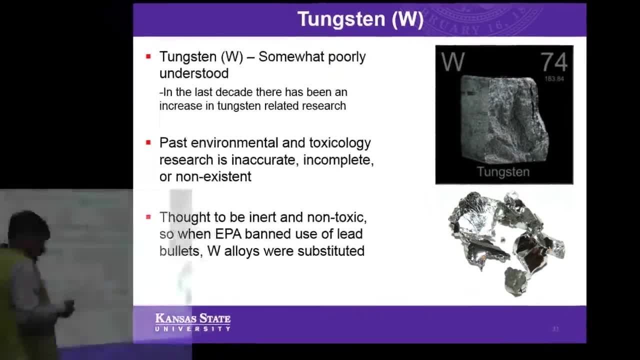 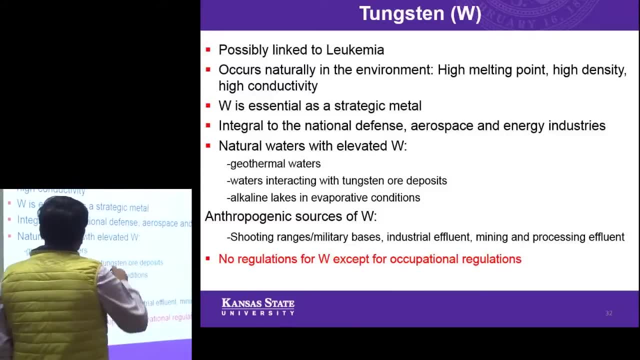 That lead was actually lead bullets were substituted By tungsten alloys. So there was a quite a bit of use for tungsten And I will tell you why. But tungsten was linked to leukemia. I will give the story in a minute. 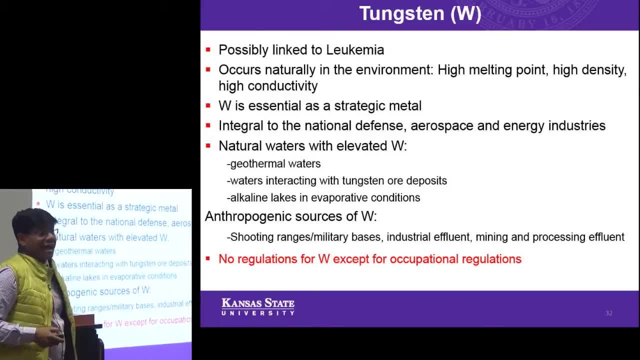 But because tungsten is naturally occurring in the environment And because of its high melting point, High density and high conductivity, It is used as a strategic metal. It is used in national defense, Aerospace and energy industries, Natural waters Which are enriched in tungsten. 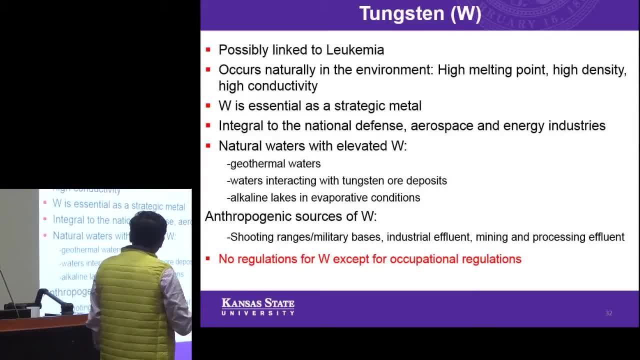 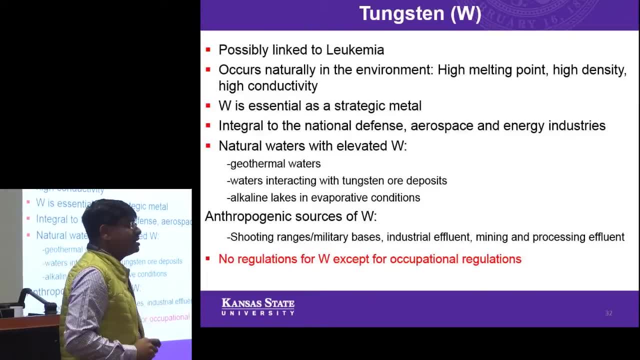 Usually occurs at the geothermal waters, Which are high temperature Waters that are interacting with the tungsten ore deposits, And some of the alkaline lakes. These are very interesting lakes actually. We just visited with our students last semester In near Fallon Nevada. 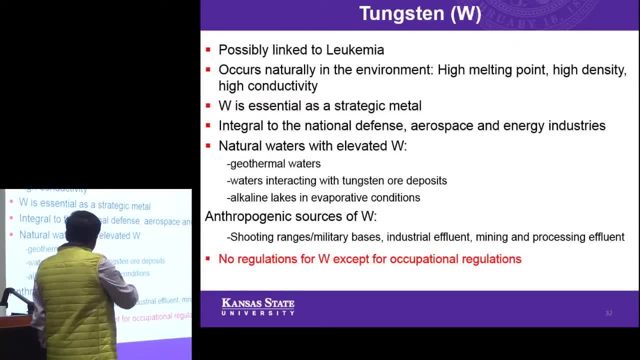 And I will give you the story in a minute. But there are many alkaline lakes That have high concentrations of tungsten in it, Because tungsten loves sulfur Or sulfides, And they bound to sulfides very well And it gets soluble. 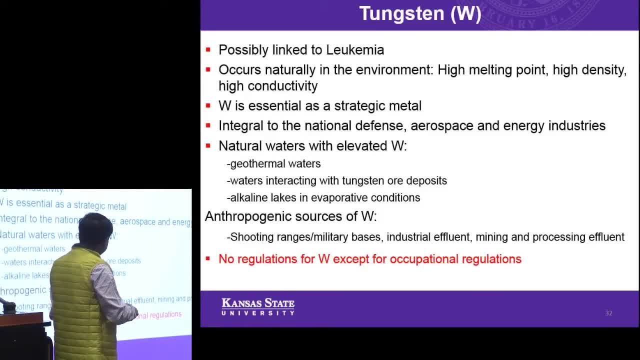 Some of the anthropogenic sources of tungsten are In the shooting ranges or military bases, Industrial effluents, Mining and processing effluents too. There are no regulation as such for tungsten, Except there is only some occupational, Occupational regulations only. 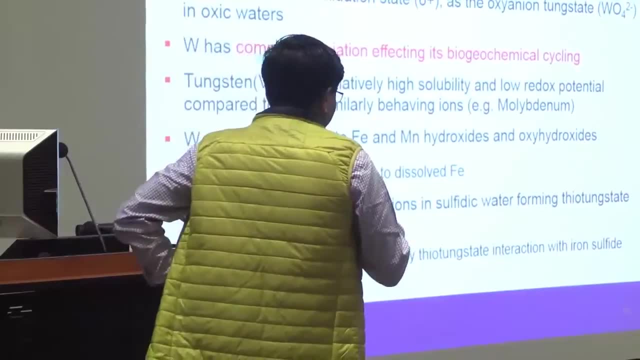 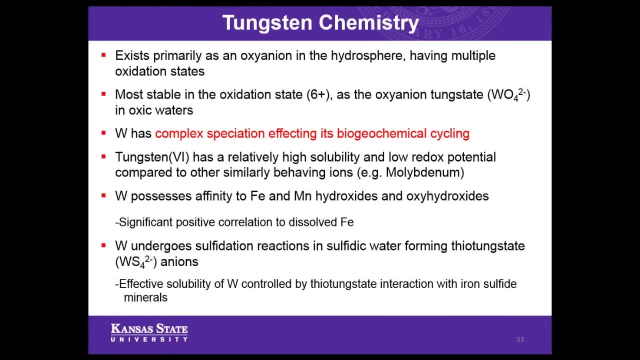 In the hydrosphere, Tungsten occurs, Have multiple oxidation states, But the most important one Is the plastic state And it occurs as As an oxyanion, And it is called the tungstate oxyanion, So it is a very soluble form. 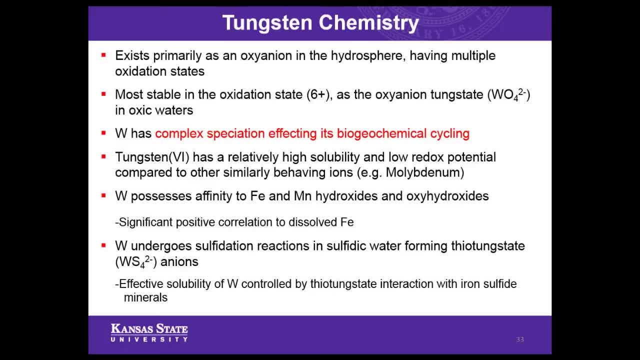 Usually it occurs in an oxic water. Because of its complex speciation process It affects its biogeochemical cycling in the nature. Tungsten is relatively highly soluble In the low redox potential range And similarly it has a common 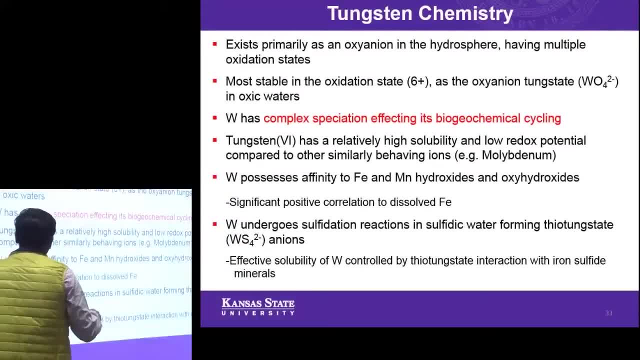 Affinity to molybdenum, As I was talking about Tungsten, possess An affinity to iron oxides And hydroxides, As like arsenic I just mentioned about, And they have a significant positive correlation With amounts of dissolved iron. 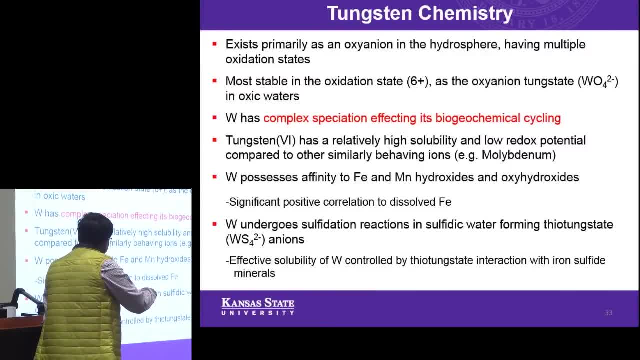 That is in the water. So they are iron lovers. But tungsten can undergo A sulfide reaction process In high sulfide rich waters, Right, And it can form In the water. So the thio tungstate complexes Among all the ions. 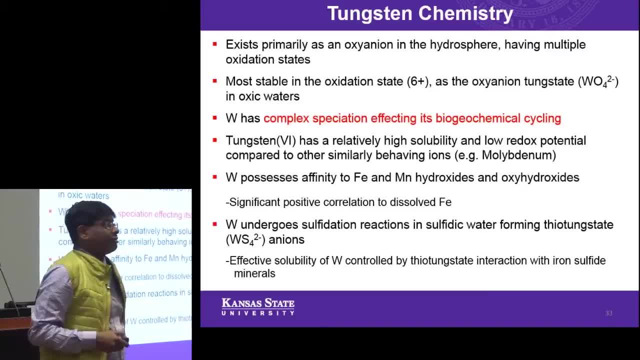 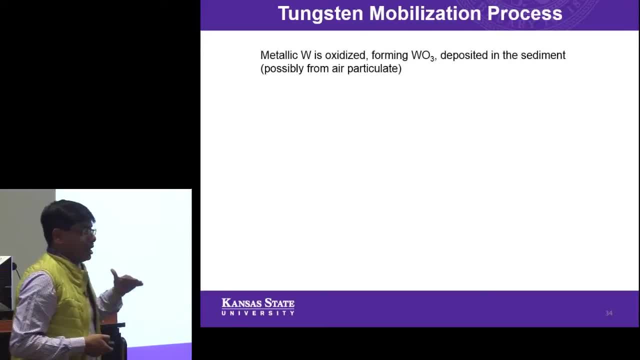 Like even more than tungstate, Are usually effectively soluble And produces a high concentration in the water. So the tungsten mobilization process I just developed a little chart for to understand. It comes as a metal, It becomes oxidized, It becomes WO3, for example. 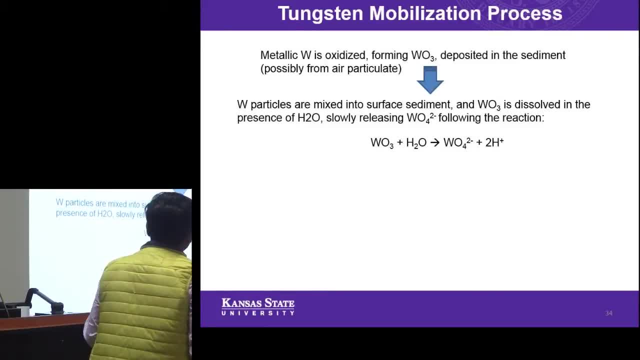 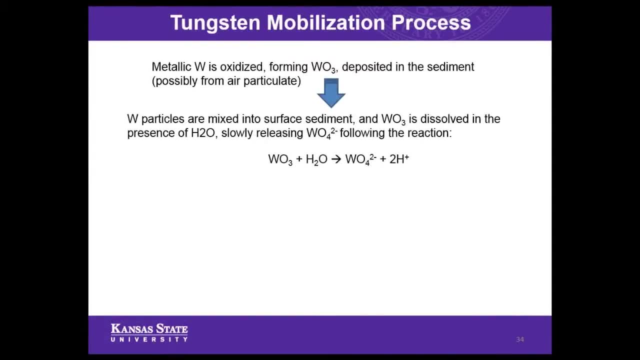 It deposits in the sediment, Possibly from the air particulates, From the surface sediments. The WO3 then dissolves In the presence of water. It slowly releases the tungstate. Slowly releases the tungstate From the following reaction: 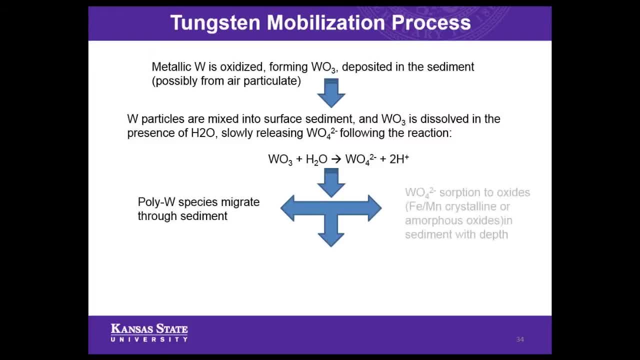 And when this reaction is proceeding, It can go into three different ways. Usually they can form A poly complex. That means it is a much more Longer chain. tungsten complexes, Or the tungstates, Or these tungstate ions, Can get absorbed. 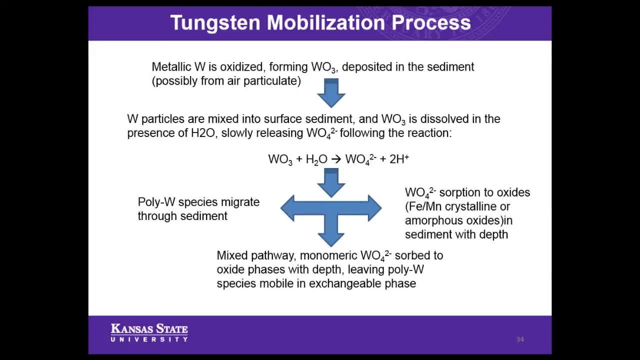 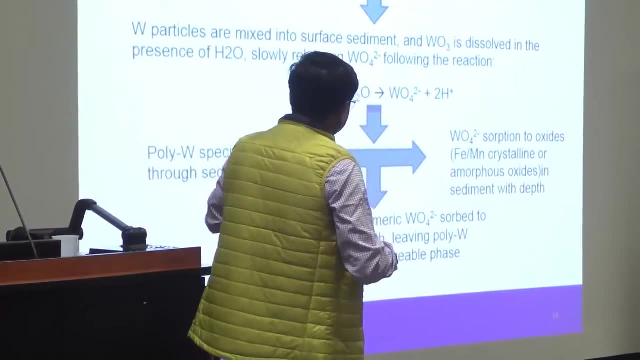 By iron oxides In the sediments And it can differ. And it can vary with depth, Or it can be It can form a mixed pathway Where the tungstate ions Are somewhat It is like both ways. It sorbs onto the sediment particles. 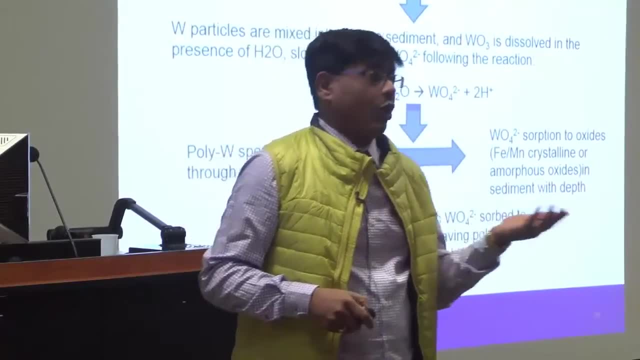 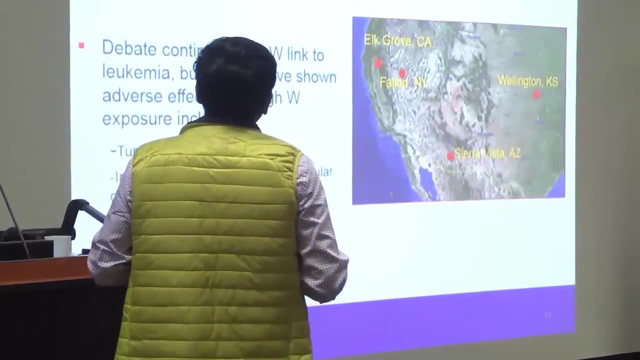 Or it can leave While the poly complexes becomes highly mobile In an exchangeable phase. Exchangeable phase means Much more highly Available to the nature. Okay, Health implications. Childhood leukemia Was attached to Or was linked to this. 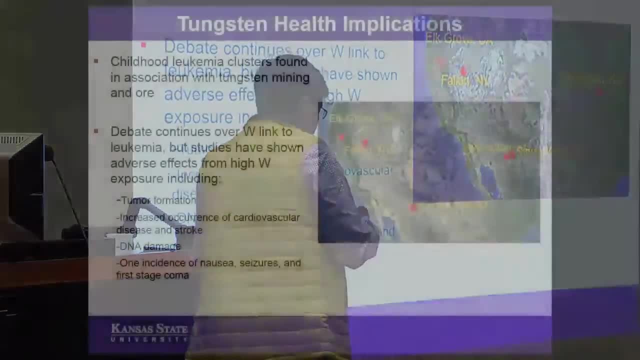 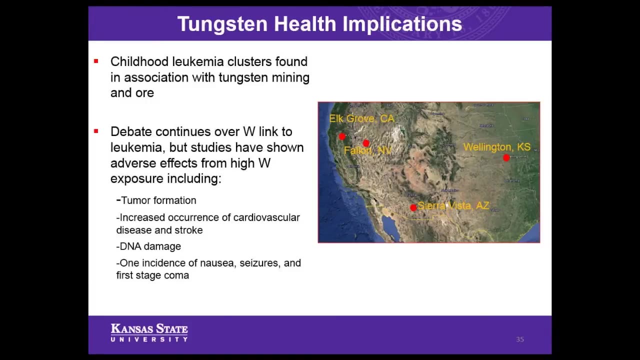 You know, In cluster, These are called the clusters here. The debate still continues, though, Because a tungsten linked to leukemia. The studies have shown that there are adverse effects: Tumor formation, DNA damage, You know, And other cardiovascular diseases. 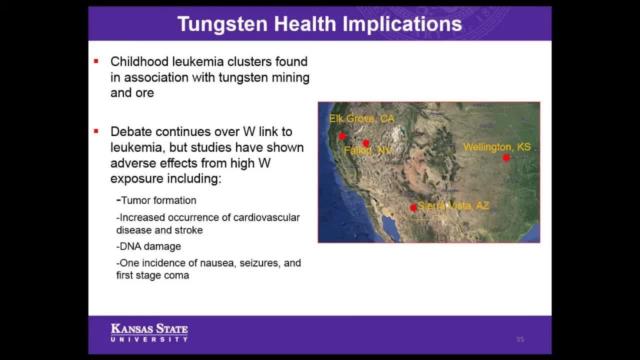 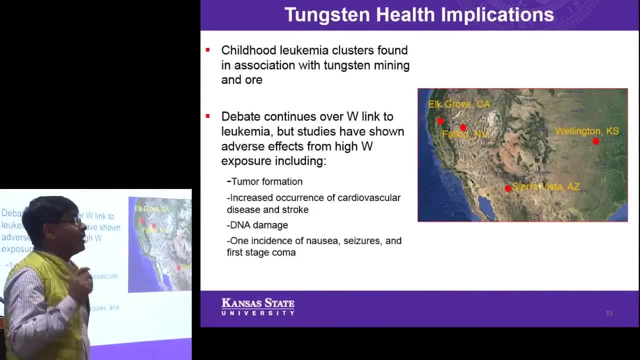 Now And the, And a couple of the places I just wanted to point out: Arizona, Elk Grove, California. You might be Thinking about Wellington, Kansas. You know It's just close by. Actually, It was a very old. 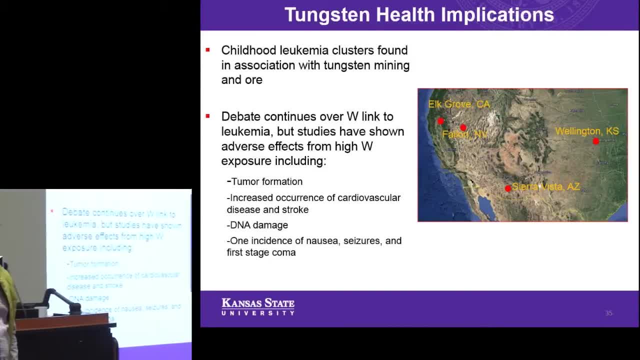 World War II Ammunition site. They used to dump the ammunitions there. There was Very slight concentration of tungsten in the soils. The water doesn't have any tungsten there, But it was reported by the CDC, The Center for Disease Control. 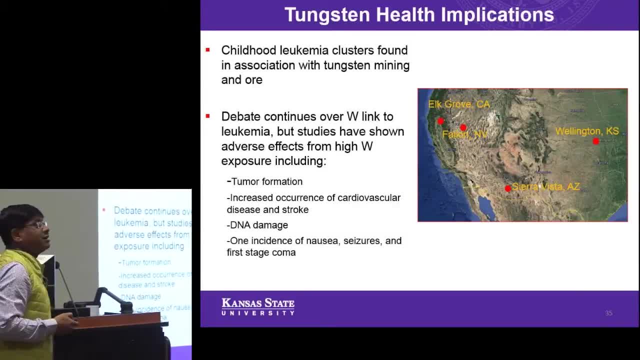 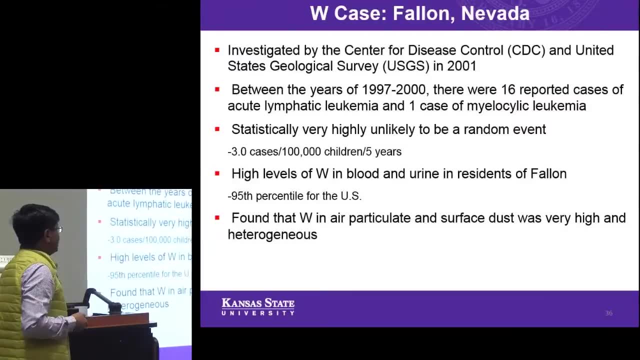 For us to go and check it out. But I have kept it in the map Because maybe in the future We might be able to find If we go and You know, Find tungsten there. It was investigated by the CDC. 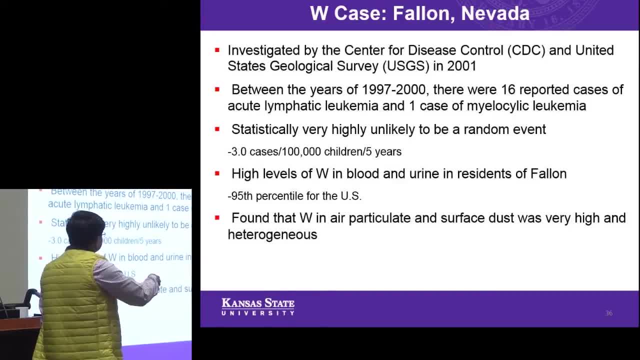 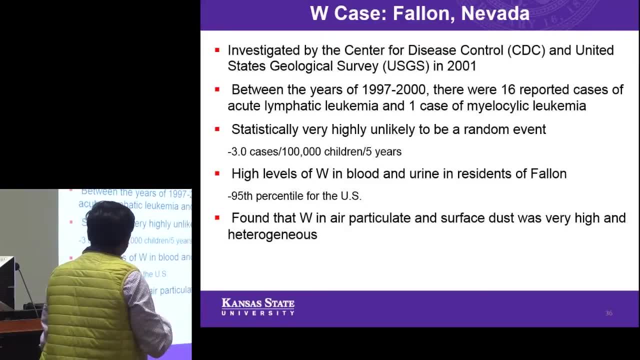 And by the USGS Between 97 and 2000.. There were 16 reported case of acute lymphatic leukemia And statistically This is very highly unlikely to be a random event, Because three cases out of the 100,000 children in five years. 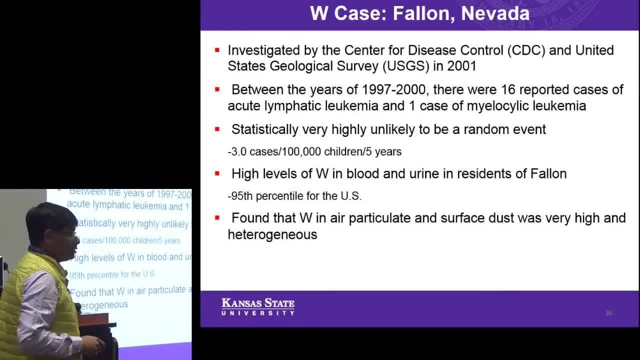 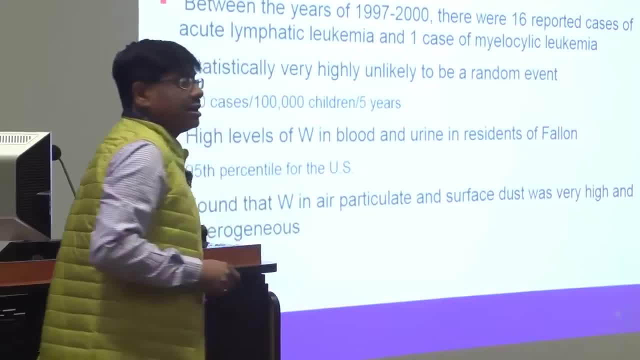 There were high levels of tungsten in blood and urine In the residents of Fallon Nevada were detected. We walked in this area actually And found that tungsten are in the air, particulates also And surface dust And in the Fallon area. 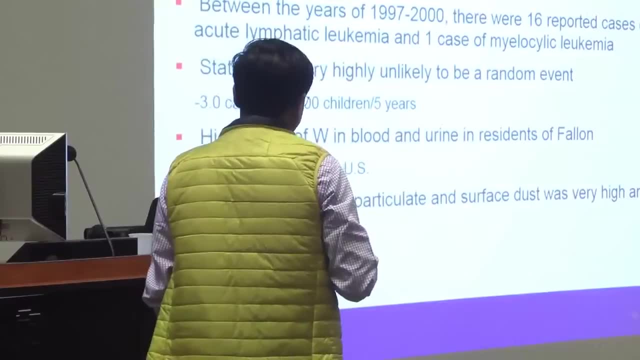 And they are very in the heterogeneous state. These are some of the places in Fallon, For example. This is the town of Fallon. We have sampled quite a bit in three different trips. We are also sampling some of the lakes, The natural lakes. 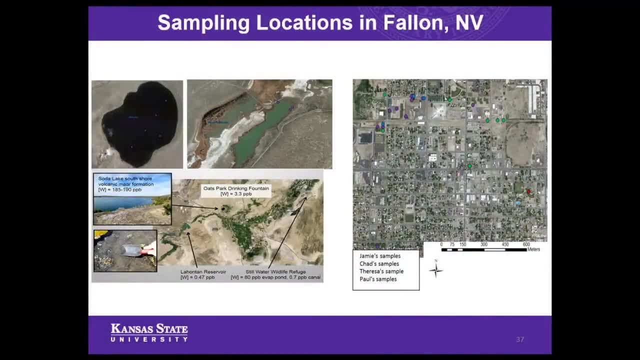 That has high evaporites And also sulfites, And they have high tungsten in them too. Now, This is a classic area Where there is a natural and anthropogenic, both Together. Well, I am not supposed to say that. 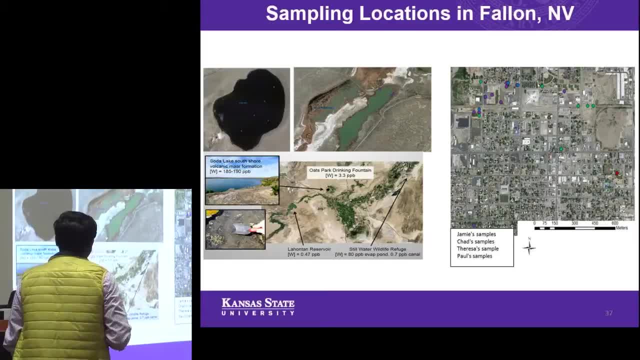 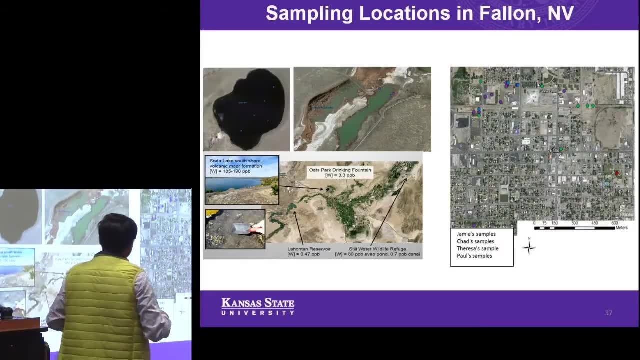 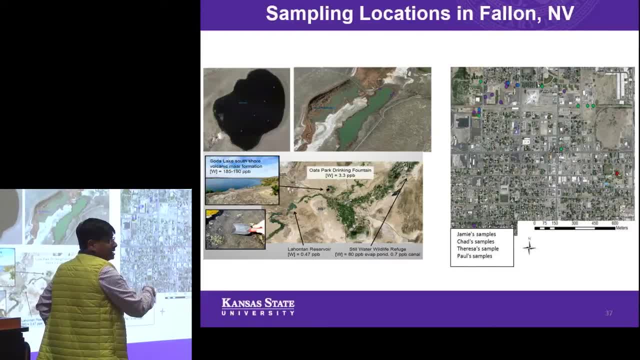 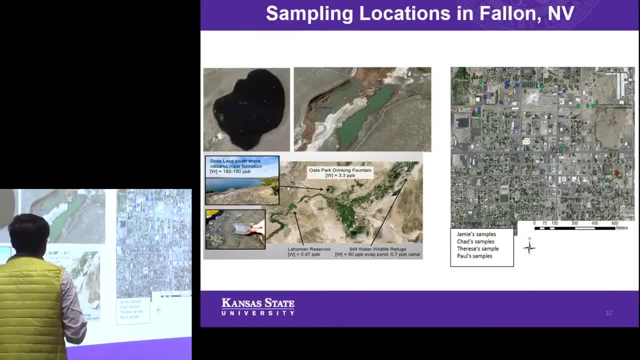 I am still saying it Because this is a Tungsten ore or smeltering plant nearby. Okay, There is a big lawsuit Going on right now Because of With this company And others Like scientists, Not us. 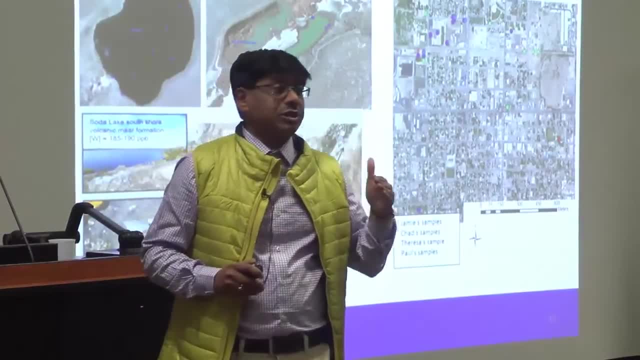 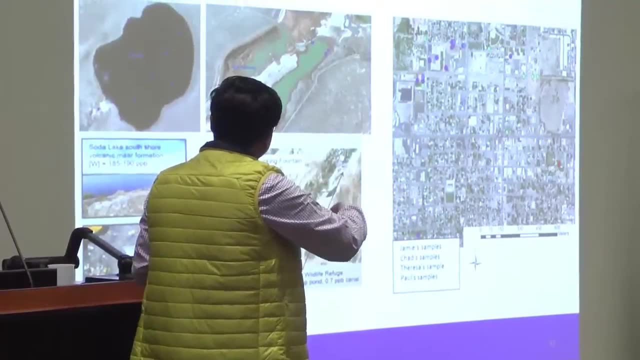 But you know. So Basically A lot of scientists think That That The anthropogenic part Is coming from the smelter plant Nearby In Fallon. But At the same time There are some natural high concentrations of tungsten. 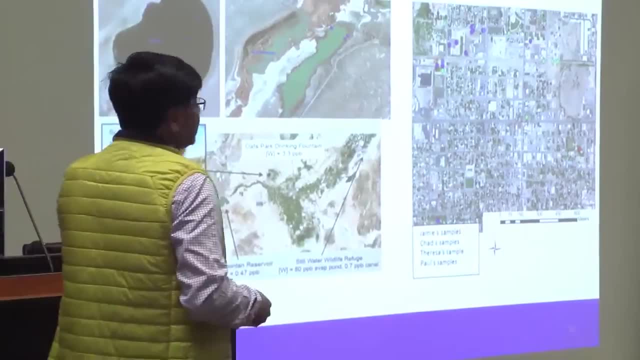 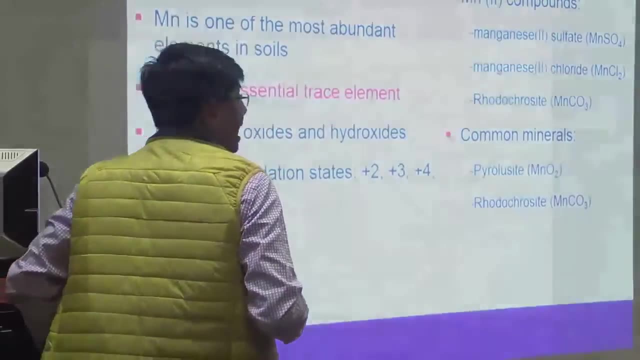 In the lake waters And in the dust- Now, the dust is not always Has to be- can be natural too. just to keep that in mind, the last element that I was going to talk about very quickly is manganese. now, manganese is such an element that 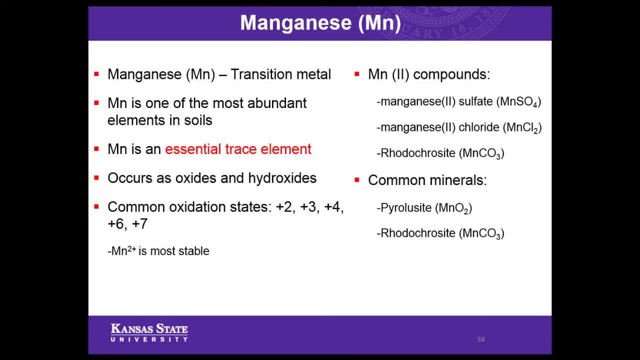 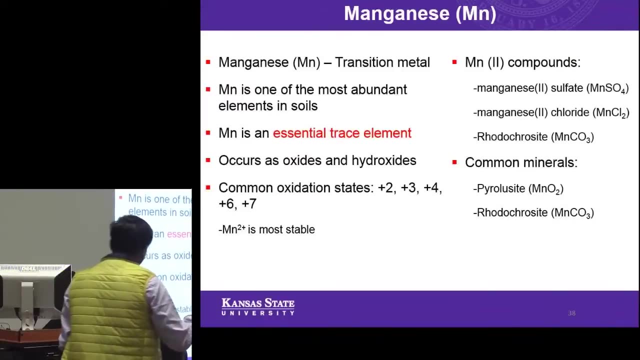 really we don't think about it and it's actually coming into our radar now more than before. manganese is a transition element. it is one of the most abundant elements in the soils and in the sediments. it's an essentially a essential trace element. it can occur as oxides and hydroxides, and the common 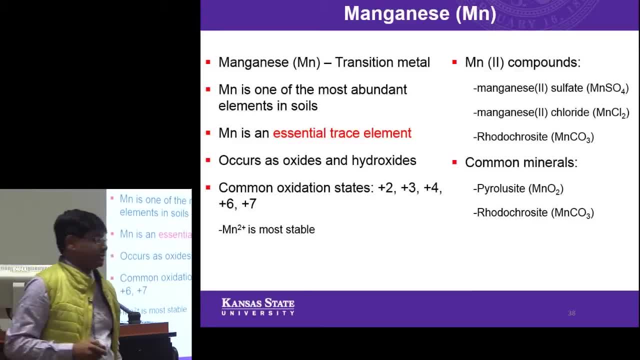 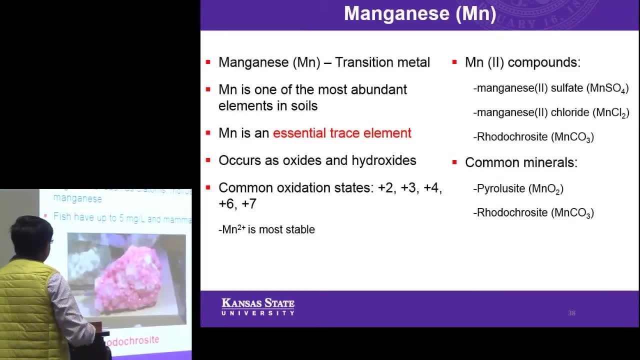 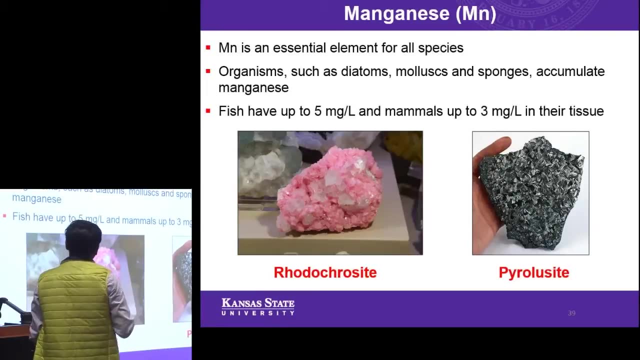 oxidation states. mostly the oxidation state of manganese is passed to. there are various different types of minerals that are present, and common minerals are pyrolysis and carbonate. mineral manganese is an essential element of all species. various organisms are there that have manganese in the tissues. a fish can. 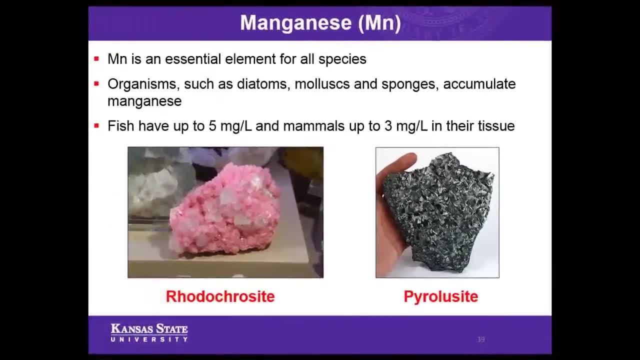 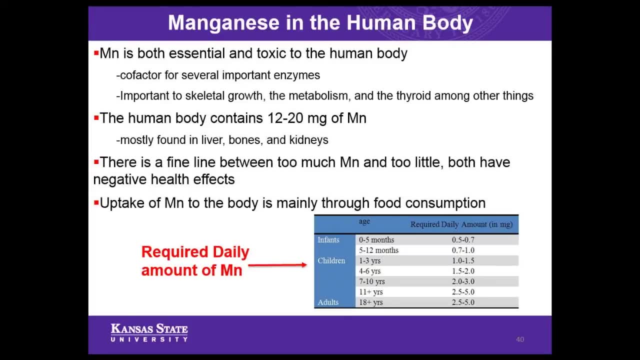 accumulate up to about five milligram per liter, or mammals can accumulate to about three milligram per liter of manganese. manganese is again an essential and a toxic element. it is usually a cofactor- cofactor for several important enzymes. the human body can contain up to about 12 to 20 milligram of manganese, mostly found in liver bones. 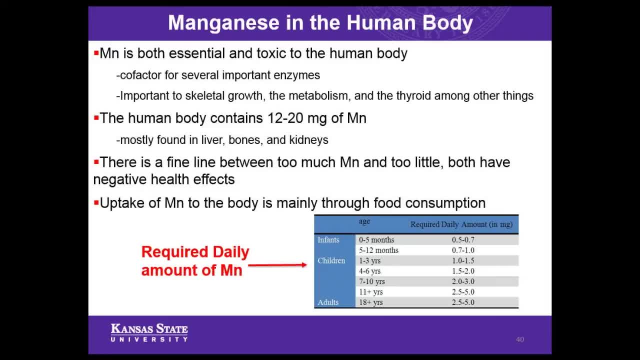 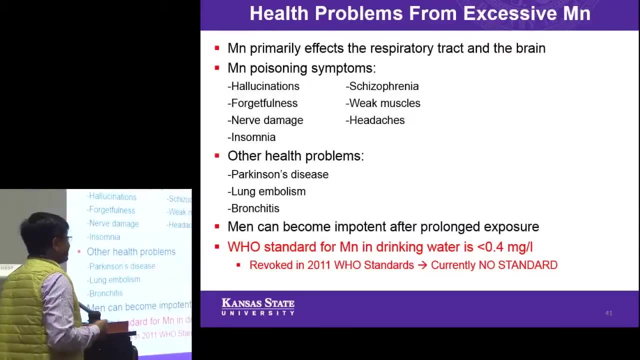 kidneys. but there is a very fine line between too much manganese and too little and both have a rather a negative health effect. and this chart actually gives you a very quick. you know, age wise, what is a daily required limit of manganese. but with the health problems of excessive, manganese comes from excess in the sense. 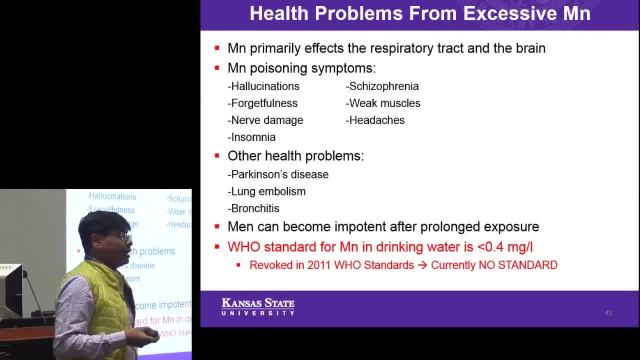 that actually we don't have a particular World Health Organization limit for manganese. it was 0.4- 0.4 milligram per liter or it has to be less than 0.4 milligram per liter, but in 2011, World Health Organization revoked that standard. 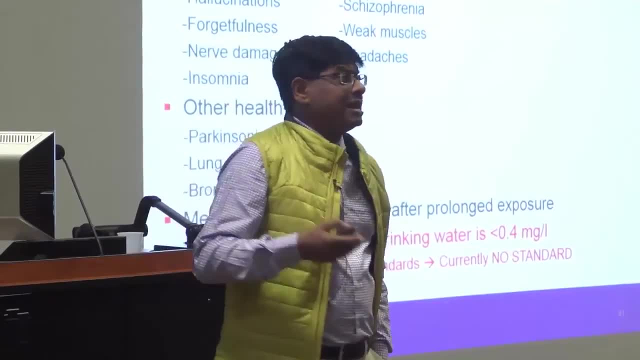 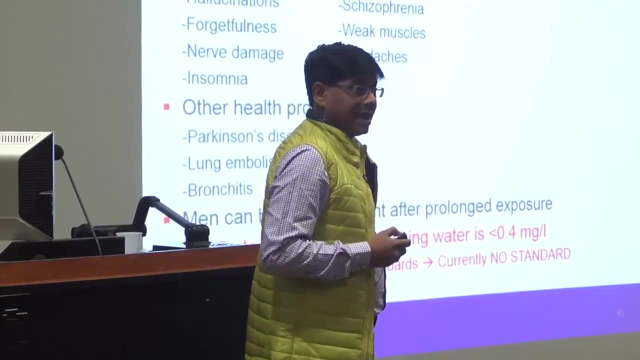 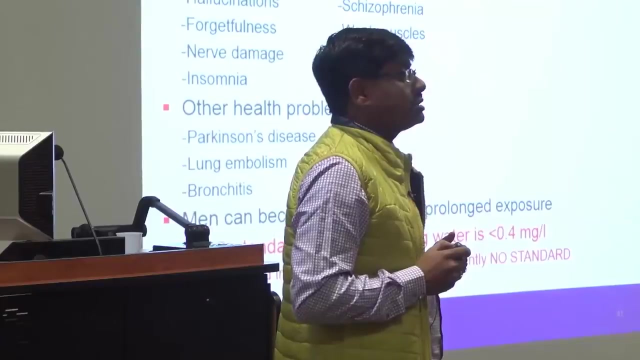 currently there is no standard, but there has been many studies that have been shown that places where there is high iron, those water also contain high manganese, and the reason behind that is that iron and manganese love each other number one in the sediments and in the soils, but iron 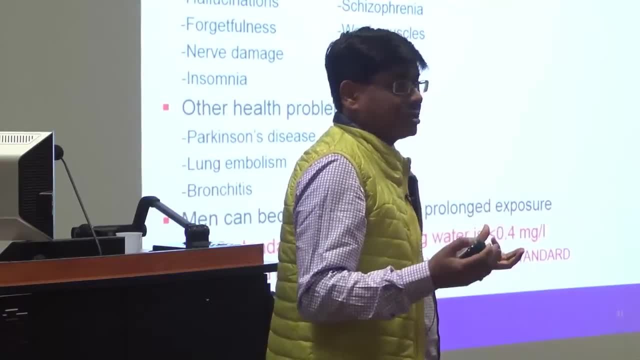 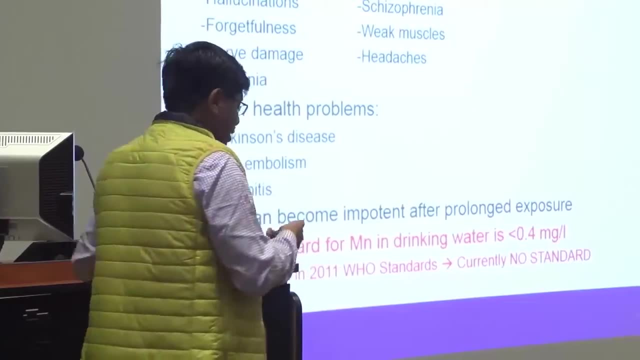 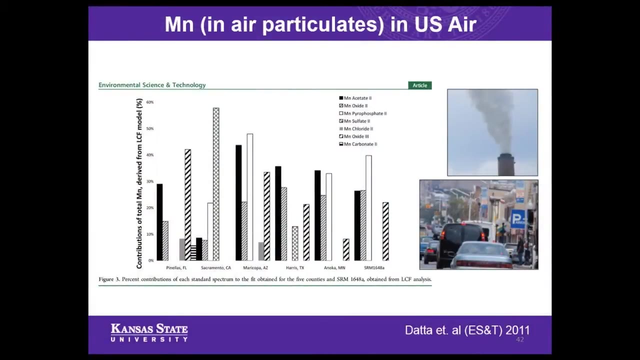 can release, or manganese can release in two different processes. so really the environmental conditions needs to be slightly different to release iron first and then manganese, so manganese can go into water quite equally. this is one of our studies that we did in the air particulate matter. in US the six or 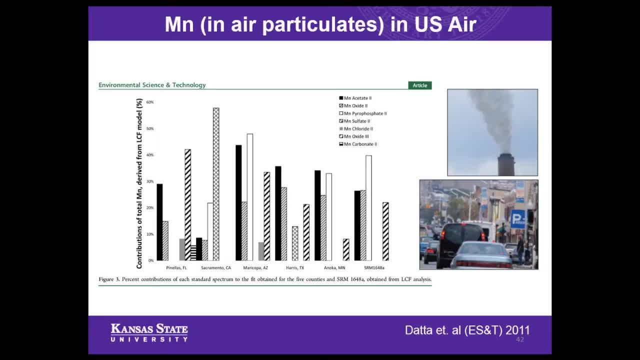 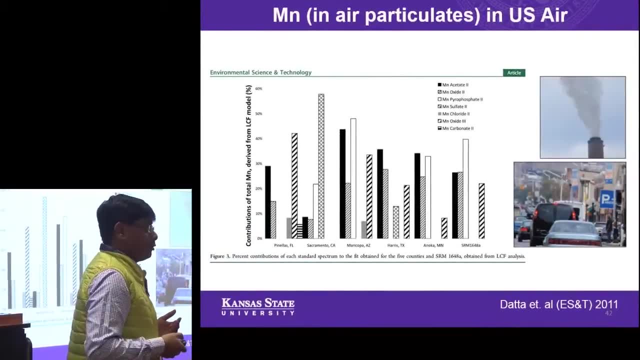 seven different cities that we did. one of the major manganese resource coming, I mean pollution happening from the smokestacks and also from the fuels, because they add additives to the fuels and we actually did concentrations of manganese in the air particulate matter usually the less than 2.5 micron fraction. so because of the time I guess I will just skip. 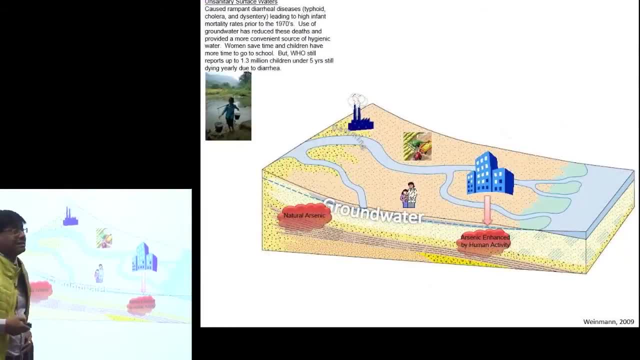 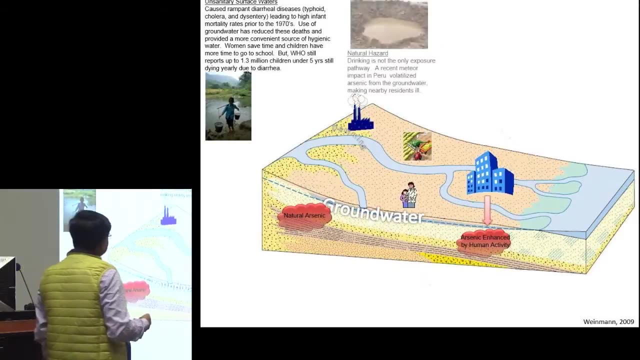 through another important element, but I'll just go to the last slide here about that. what happens in this trace elements and metals and metalloids? it's? it starts with the concentrations in the surface waters. right there is. a major part of it has to be from natural hazards also, or natural contamination, or 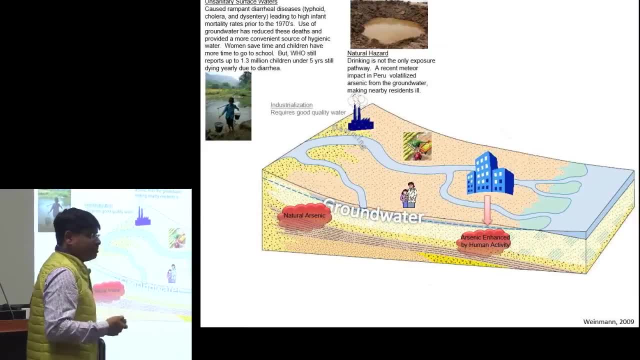 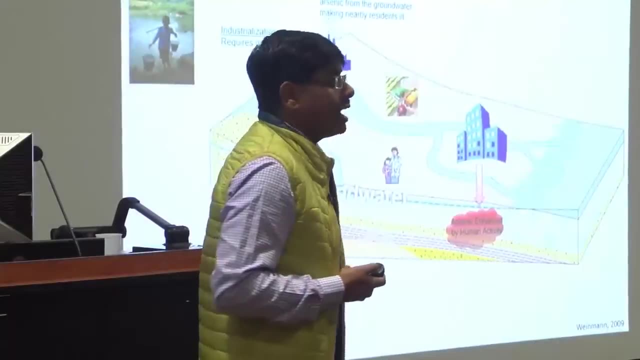 anthropogenic regulation. there is. a big component of these metals, or metalloids, comes from the industrialization process. also, it requires good water quality. there is a lot of health. not only health, but there are social impacts for this heavy metal contamination in water. right there are places where people are shunned. 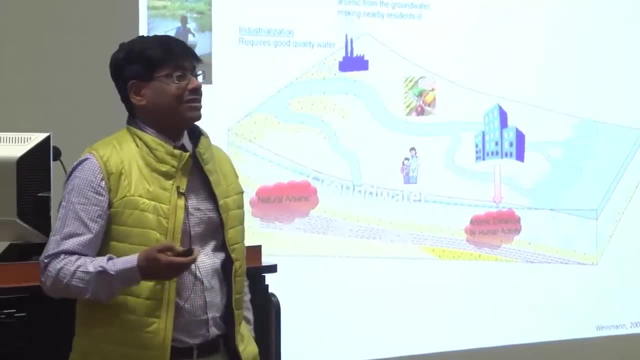 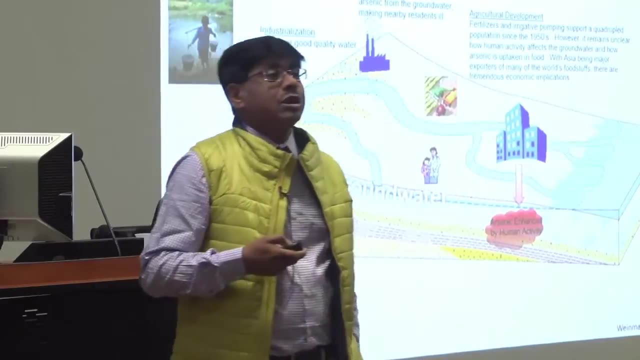 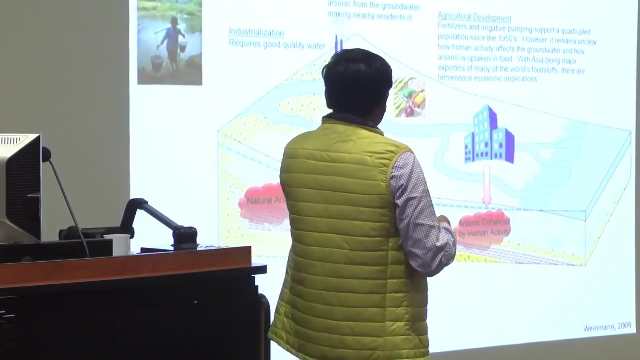 in the community because of having contamination or having some disease that comes from heavy metals and so on. so it has a societal impact also. agricultural development has led to many such uses of herbicides or pesticides, for example, that can, or fertilizers that are, and the processes of irrigation that 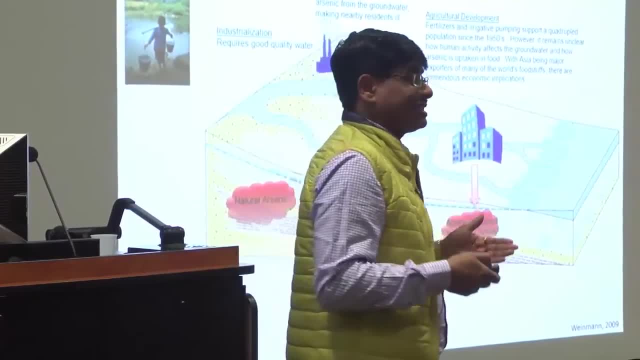 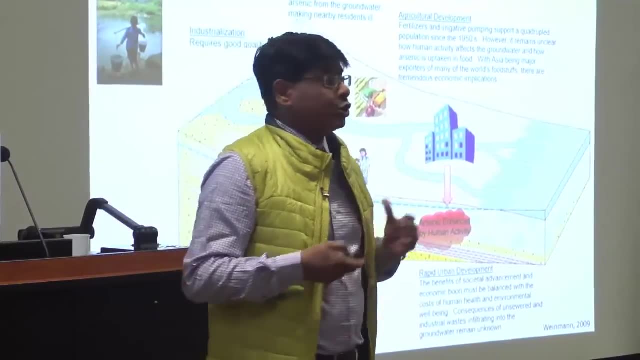 can lead to. it's rather unclear to us that. what is the extent of increasing the pollution? like that way for heavy metals, rapid urban development is happening, so in that way also in some of the places where there is, you know, more of the economic boom, boom is. 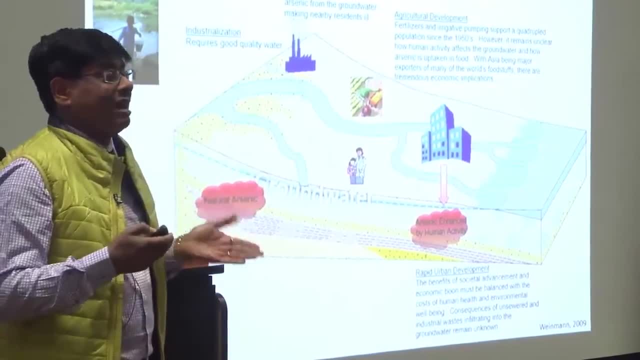 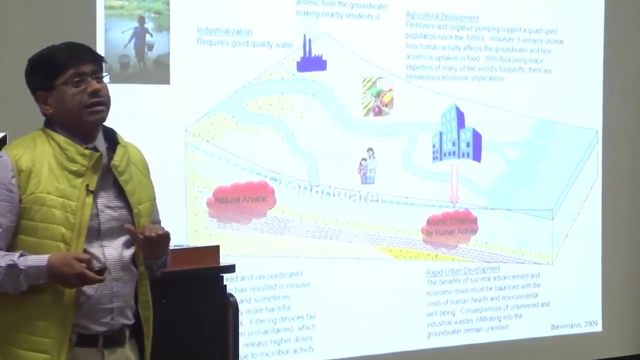 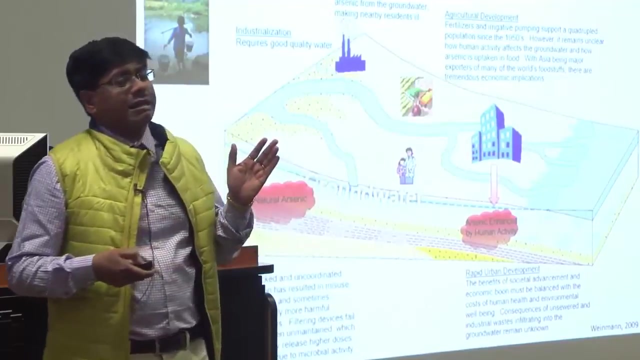 happening there. maybe there is a balance of the human health and the environmental impact and then from there, really the mitigation part, which I didn't cover today. there are a lot of mitigation strategies that are being taken nowadays for different heavy metals. the three that I talked about is the for the 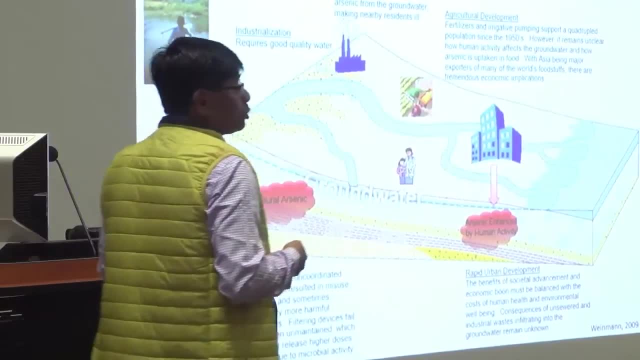 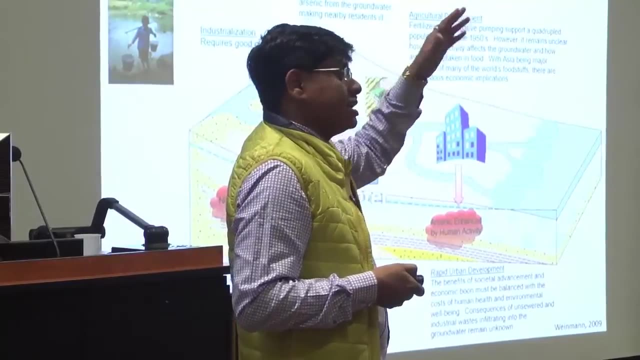 arsenic, manganese and tungsten. the one that I skipped is chromium. I just wanted to point out one thing. you might have seen the movie Erin Brockovich. this is like in year 2000, like in a Julia Roberts movie. it's a classic case of metal pollution from in the water systems, from 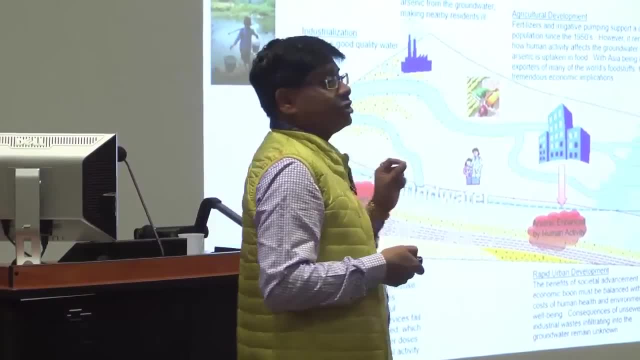 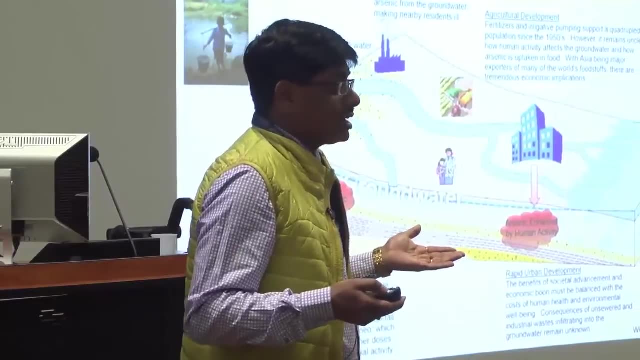 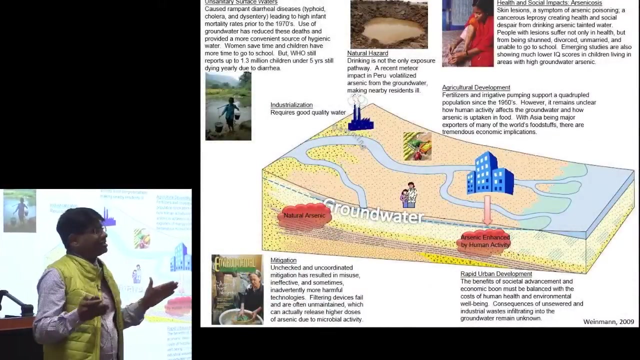 a tannery, for example. right, so tanning industries actually produce a lot of hexavalent chromium, which is six valent chromium that goes into the water and is very, very, very toxic. so, but chromium, you know, in, in, in terms of these elements that that we have worked with, there is a diverse nature of its similarity in their 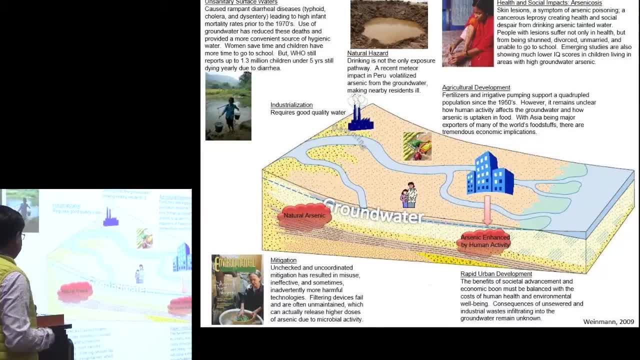 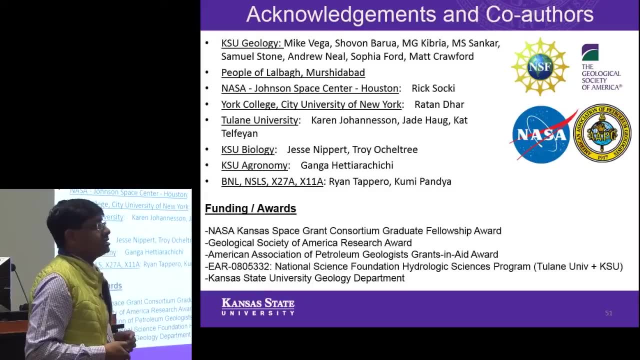 you know the ways they they actually occur in nature and how they process in nature. with that, there are many people to thank for this work. we have been funded, as dr Hutchinson mentioned mentioned, through the years and we are really privileged to work in this area. thank you very much. 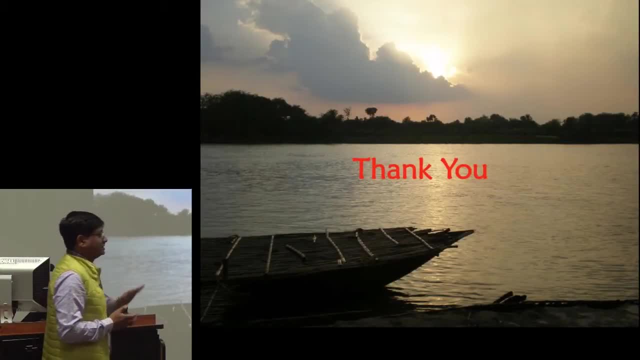 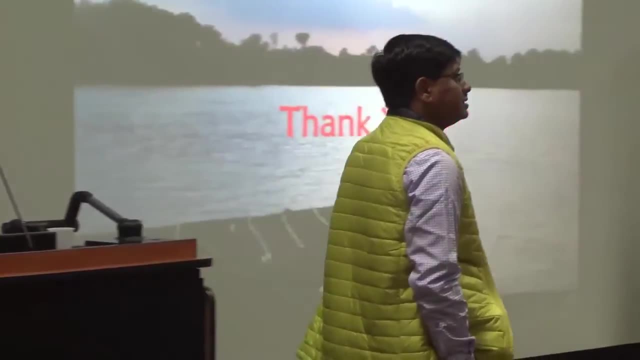 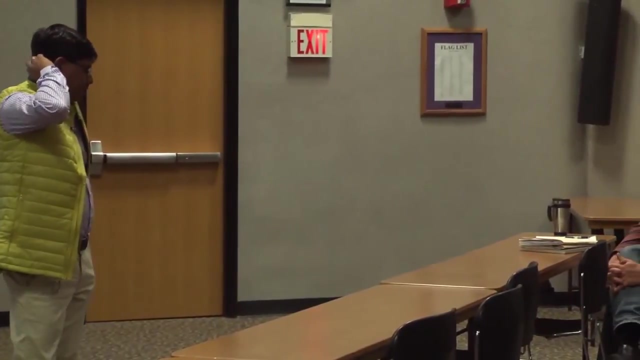 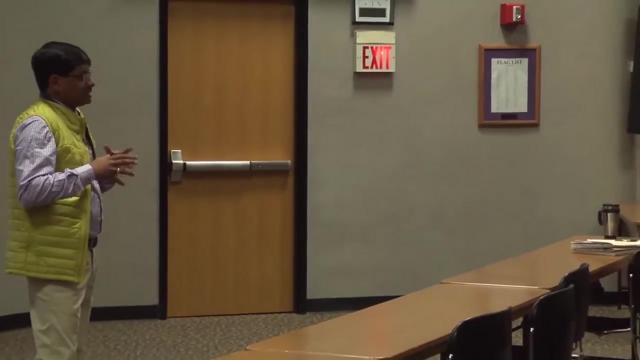 yeah, any techniques that are being used to try and remove some of these heavy metals from the environment? so great question. so, for example, first of all, we need to know that what substrate those heavy metals are in, for example, if it is soil, sediments versus water. water remediation or water filtration systems has been much more. 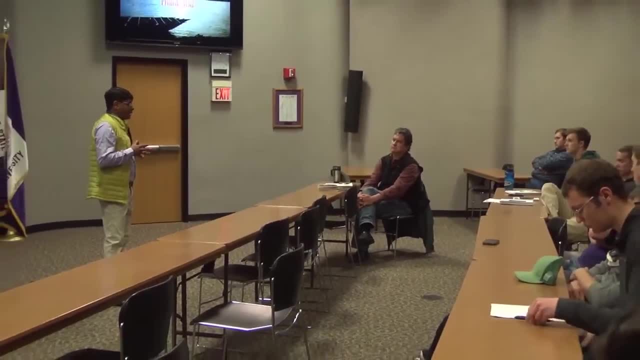 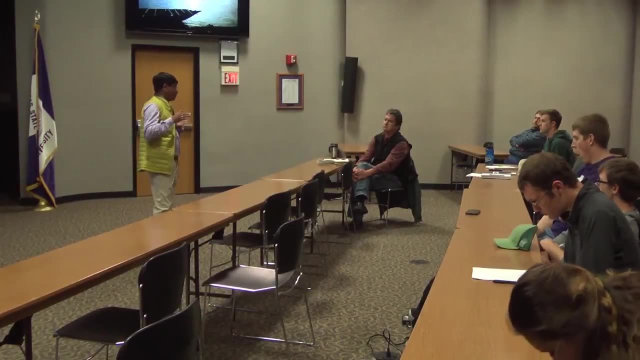 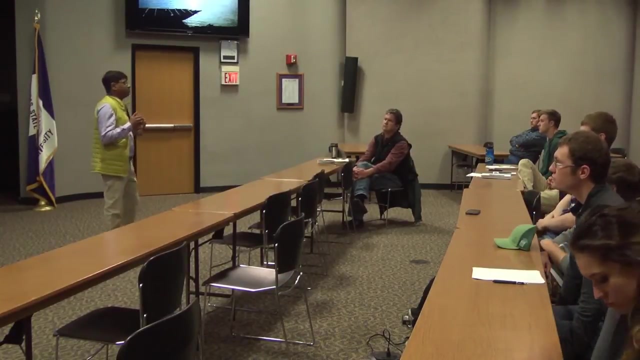 mechanized nowadays. I would say that there are arsenic, for example, or manganese, for example. there are ways to remove the water, manganese or arsenic- from the water, not to the fullest extent, but to a large extent to be drinkable at least. and the part that is important here is that lot of 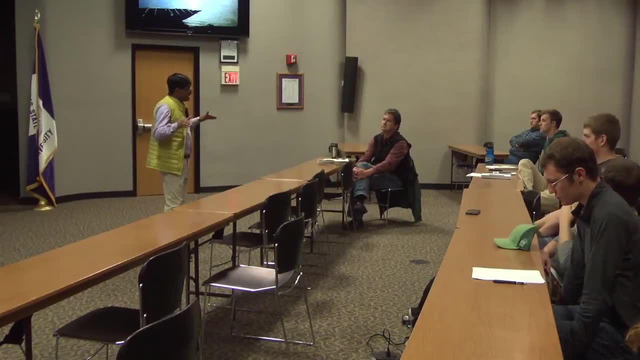 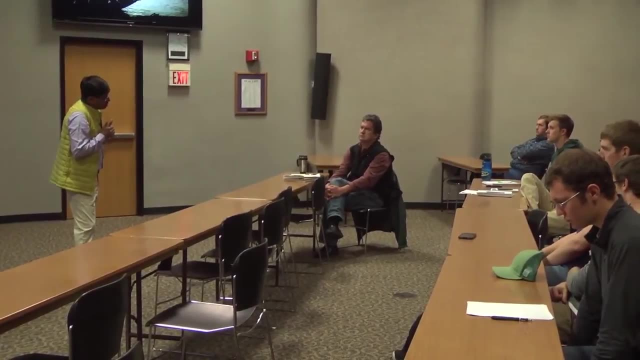 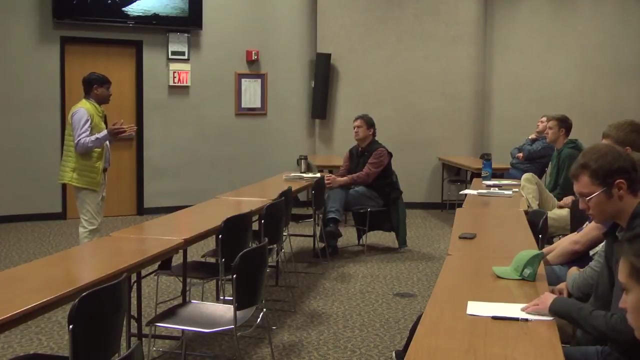 lot of folks think that you have to totally eradicate the concentration of the metals from the water. that's not the case. if you are getting it below the maximum contaminant limit or the MCL, you can still use that water. for example, a water that is 50 microgram per liter of arsenic, for example, you can bathe in. 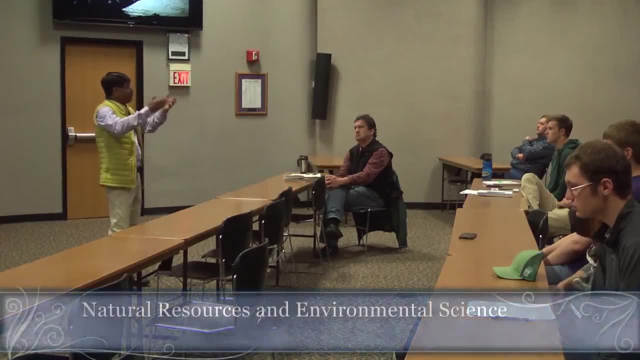 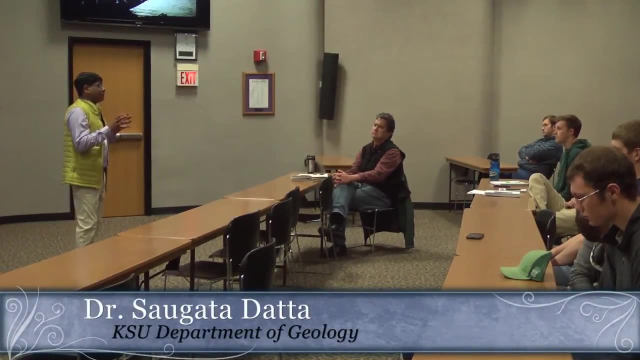 that water, so there is nothing happening with that. but you cannot just imbibe the water for a long period of time. that's when the problem starts to happen. so the so the classic example of kind of understanding these concepts together as how these metals actually behave or how they.